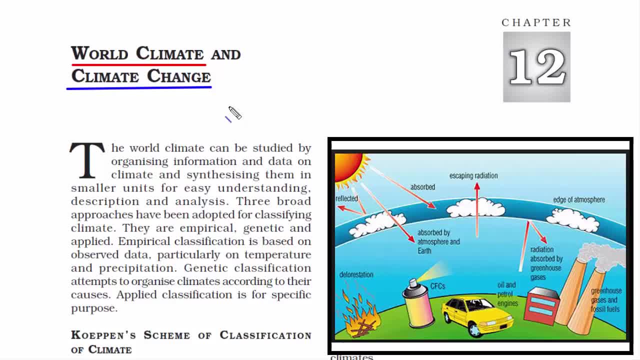 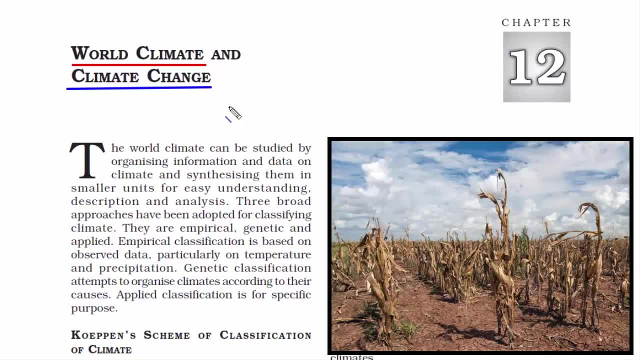 change. So climate change is very closely associated with global warming And it poses a fundamental threat to the land, ocean species and people's livelihood. So these are the two main topics that we are going to read in this chapter, And at the end it will give us a broader 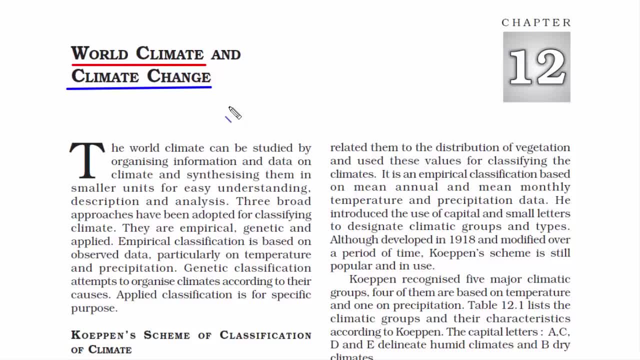 understanding of how climate has a direct impact on the social, economic and cultural aspects of human life. Climate change is classified into three categories: empirical, genetic and applied. Now, what do we mean by that? Before we understand these three categories, I want to quickly say this. let's assume you need 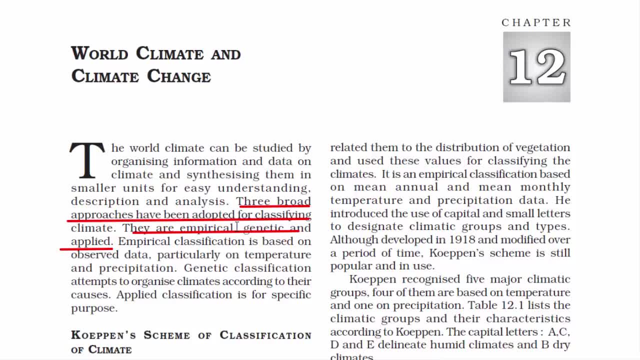 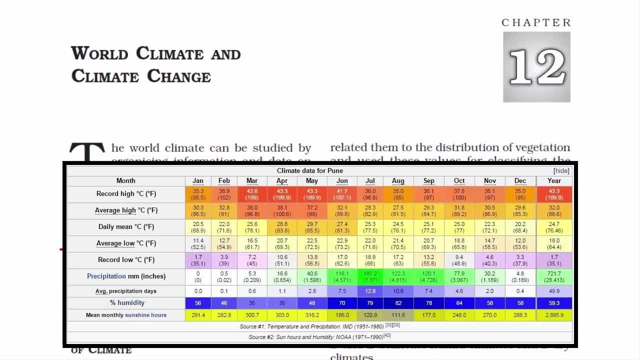 to find out how much the climate of a particular place has changed over time. How do you do that? Well, you need a daily, monthly or yearly record of weather and climate data. right, If you have this data set, you can pretty much find out the average temperature, or you can find out the. 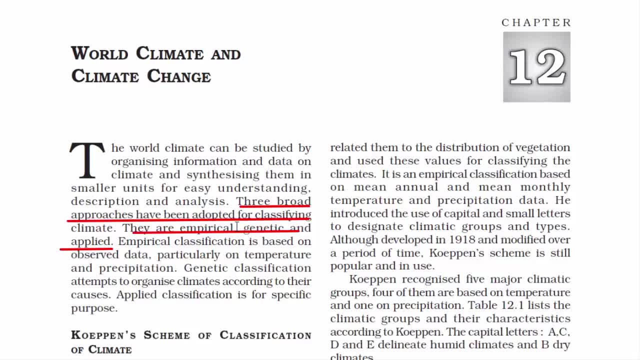 standard deviation as to how much the temperature is. So if you have a data set, you can pretty much find out how much the temperature has changed over time, right? So basically, a climate and a weather record have to be maintained. One good way of collecting such data is you go to Google and search. 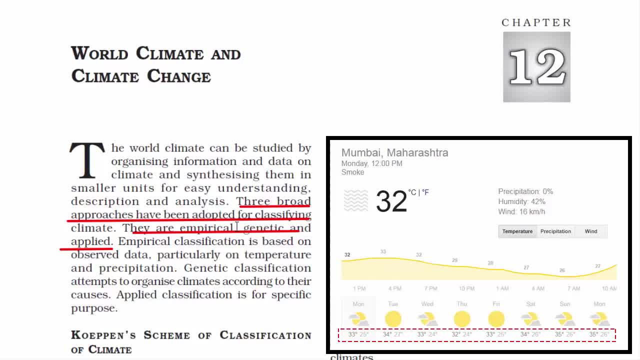 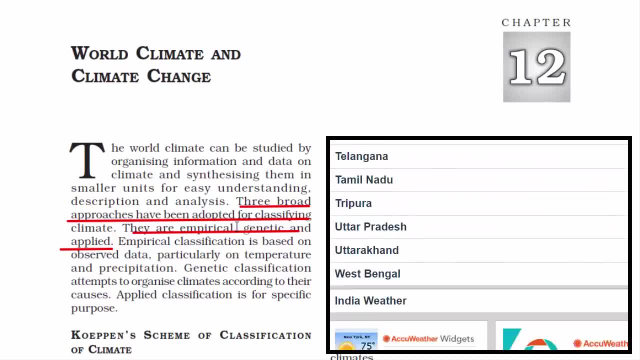 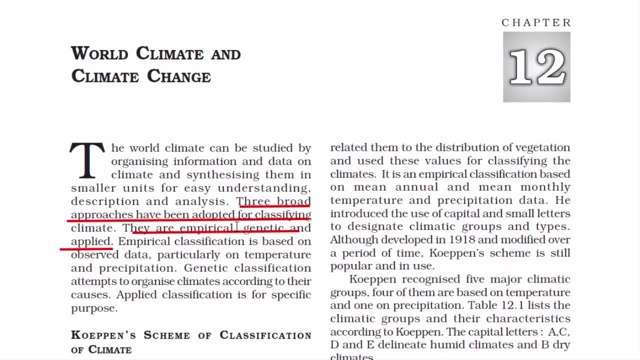 for the temperature of any place, You find daily weather readings. If you copy all these readings in an Excel sheet, that becomes a data set. So, like this, every country's, every region's meteorological department collects and maintains a data set. Alright so far. I hope it's clear Now. let's get back to the three broad categories in which this data set is collected. Now, let's get back to the three broad categories in which this data set is collected. Now, let's get back to the three broad categories in which this data set is collected. Now, let's get back to the three broad categories in which. 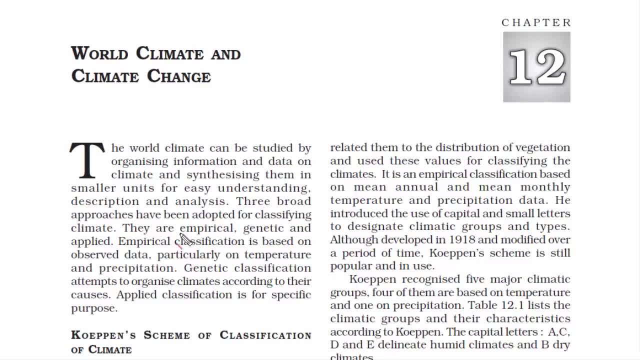 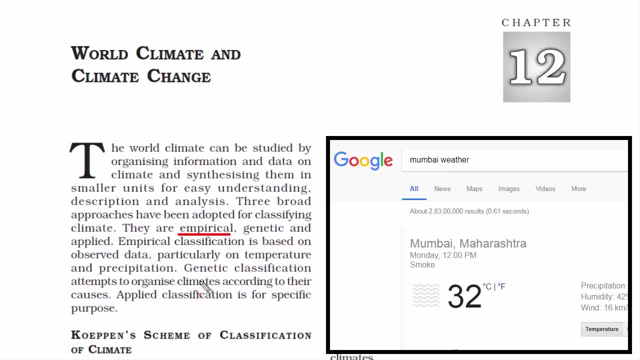 the climate has been classified. The first one is empirical classification. The meaning of the word empirical is factual, real or verified, and observed data. So empirical classification means that the climate has been classified based on observed data. Just go back to the example that. 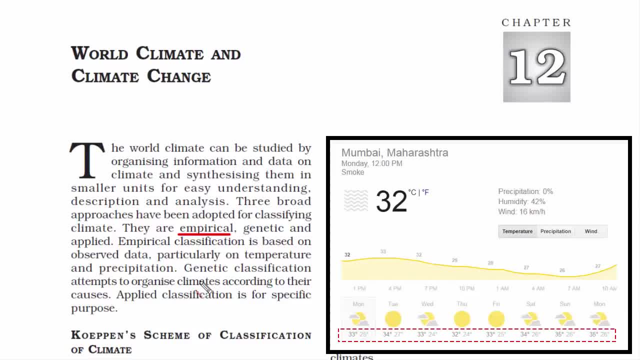 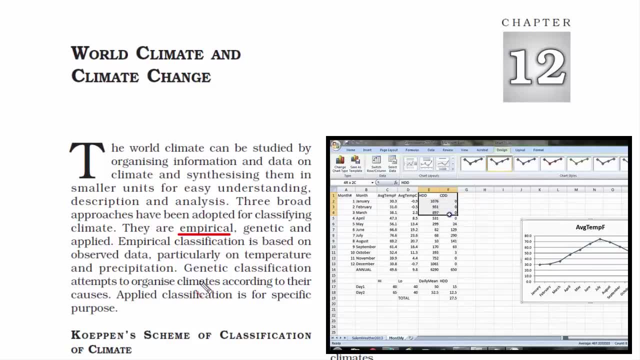 I gave moments back. you go to Google and search for the temperature of a particular place. If you copy all the daily temperature readings and put it in an Excel sheet, that becomes an empirical classification of climate. The second one is empirical classification. So if you copy all the 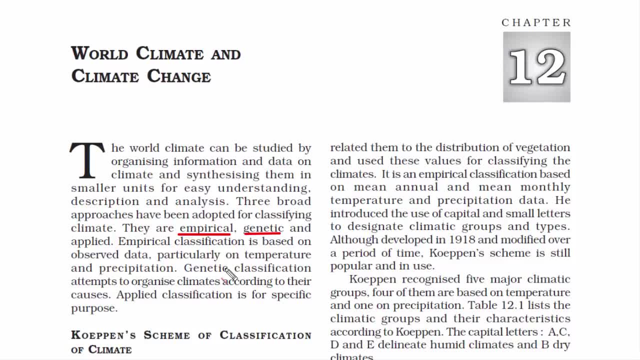 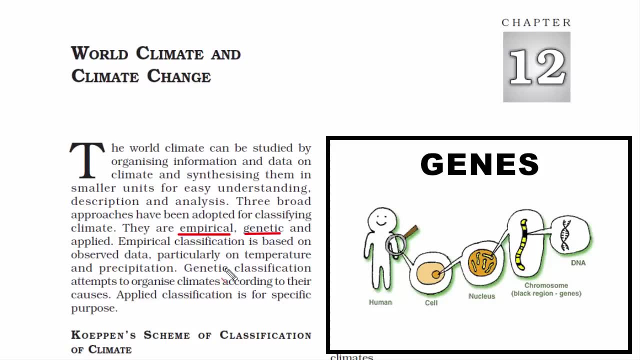 daily temperature readings and put it in an Excel sheet, that becomes an empirical classification of climate. The second one is genetic classification. When you look at the word genetic you must relate it to the word genes, because when we study genes we try to find the origin of whatever we are looking for. So genetic 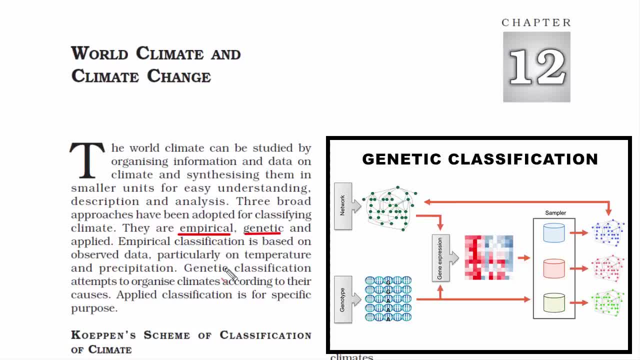 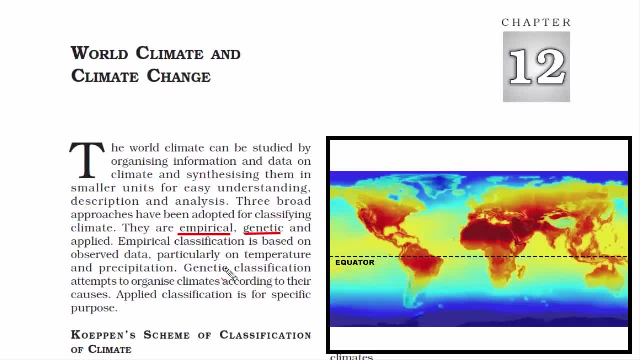 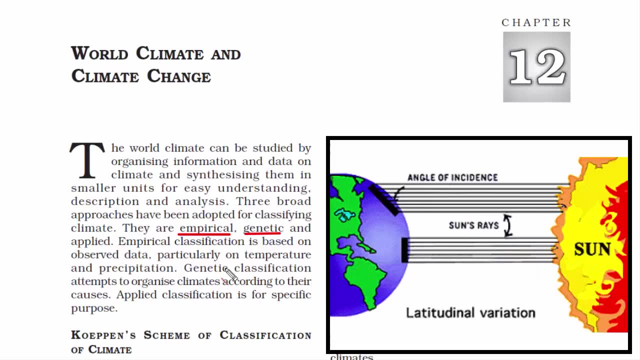 classification of climate means classifying the climate according to their causes or origin. I said climate is not same everywhere. It is due to the differential heating pattern of places on Earth. Now, this differential heating pattern is due to the incoming solar radiation on earth, which is uneven. you know, not all places on earth receive equal amount of. 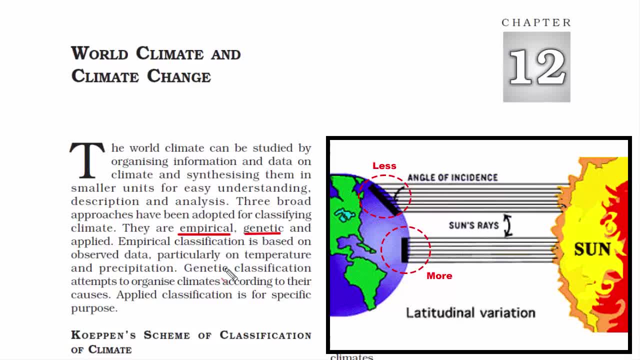 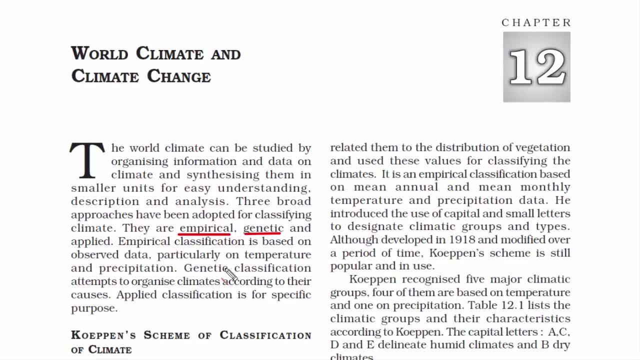 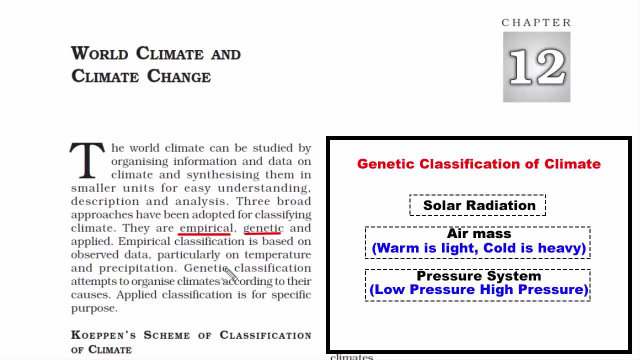 sun rays, and you also know that because of differential heating pattern the air becomes warm as well as cool. then it also causes high and low pressure belts in various places. so when we have genetic classification of climate, it means classifying the climate according to its causes and origin. so here the causes of climate change are due to the elements like solar radiation. 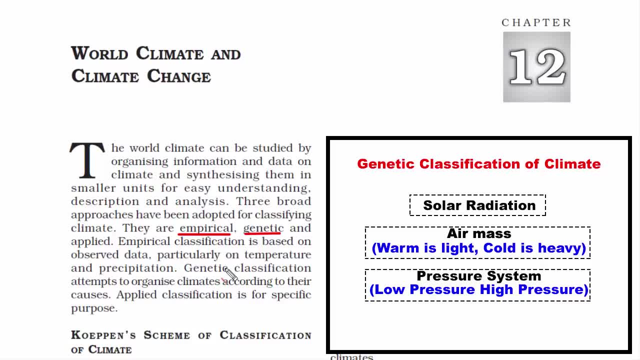 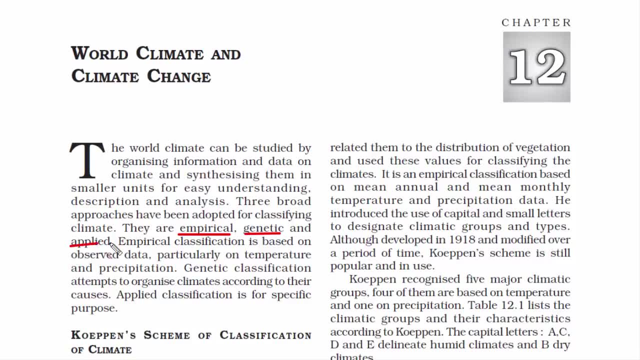 air mass pressure system, etc. so genetic classification of climate is based on its origin or cause. and the third category is applied classification. now, if you look at the word applied, it means to apply for a specific purpose. so applied classification of climate focuses on the needs of economic and social life. i'll give you a quick example. suppose we do classification. 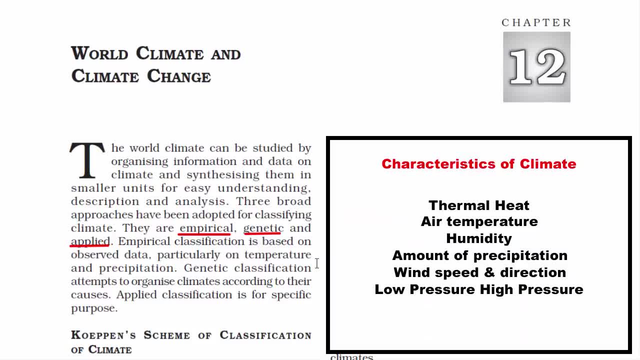 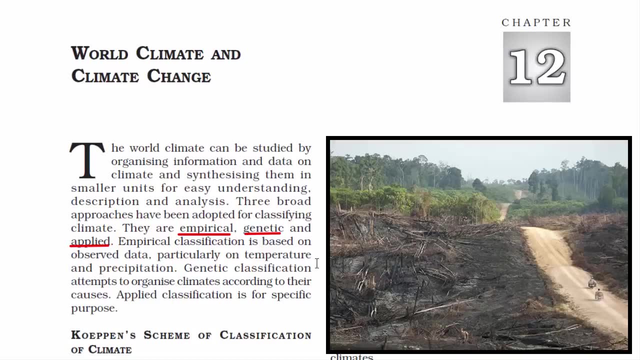 of climate based on characteristics like the thermal heat, humidity condition, temperature, temperature temperature temperature temperature temperature temperature, the nature and speed of the wind and the depth of snow. so this kind of classification can help us in making the economic estimation, for example, housing, construction, large-scale agricultural activity. 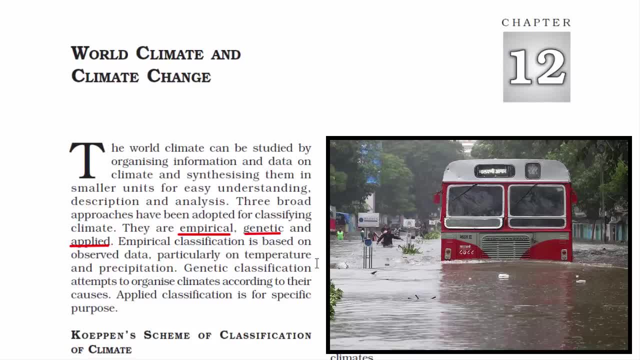 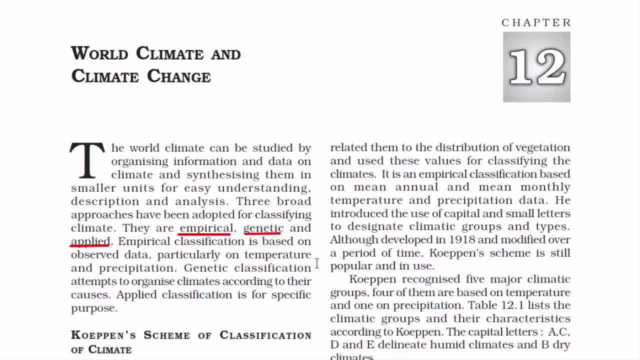 energy generation, then damage to public property due to snow and rain. these are few examples that require economic estimation. in order to conduct an economic estimation of these activities, we need to classify climate so that necessary steps can be taken and resources can be allocated, because, you see, indirectly the climate influences a country's economy and its stability. 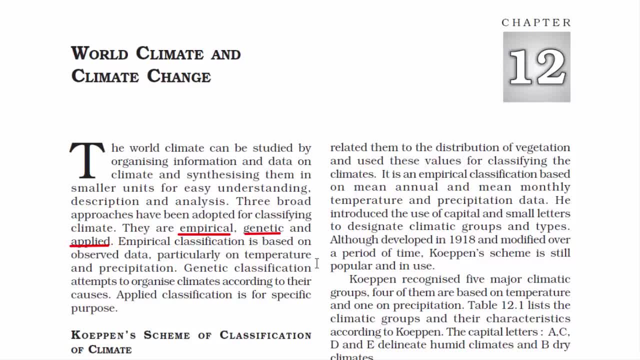 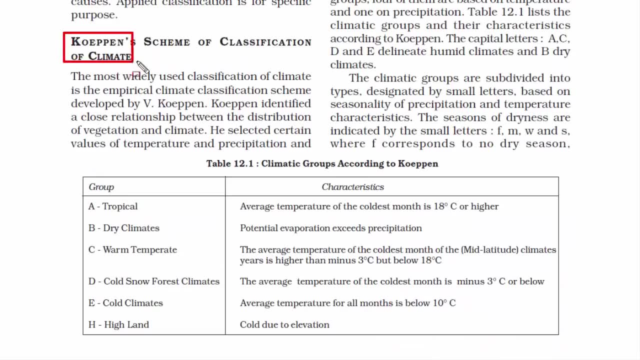 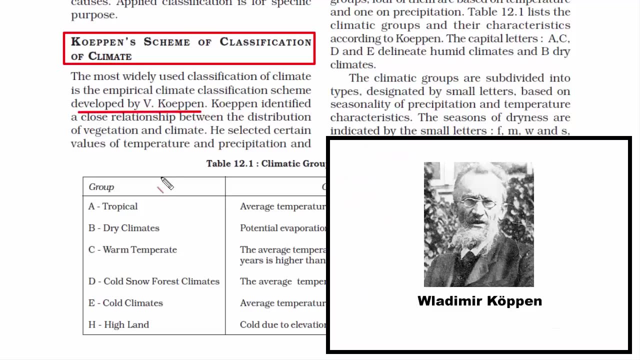 that's why the applied classification of climate is aimed towards taking concrete decision related to the needs of economic and social life. now let's go to the first topic of this chapter: copen scheme of classification of climate. so this person, vladimir copen, who was basically 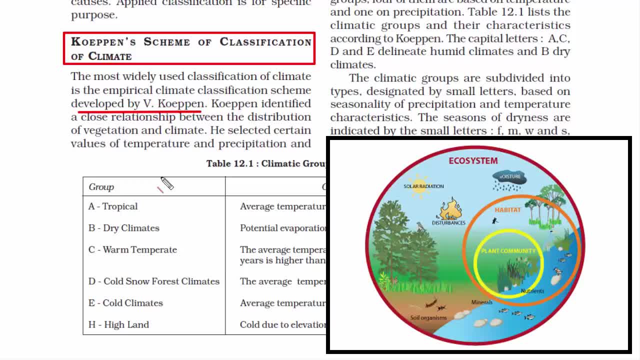 a russian, german climatologist. he classified the climate of the world by finding a close relationship between the vegetation and the climate of a particular region. his aim was to make a chart with formulas and notations that would define the climatic boundaries in such a way that. 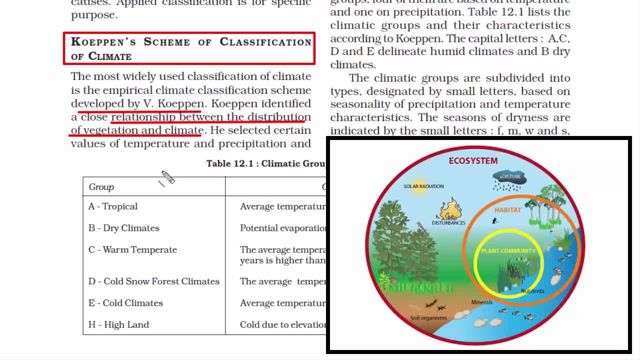 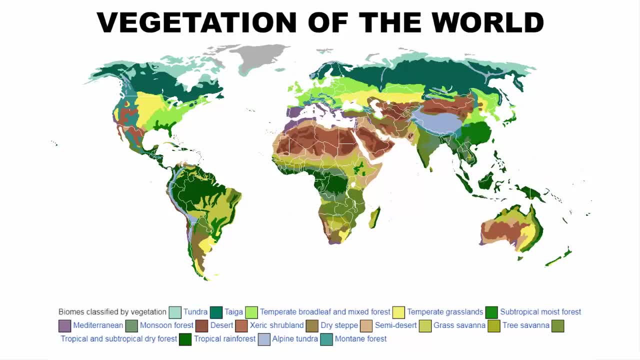 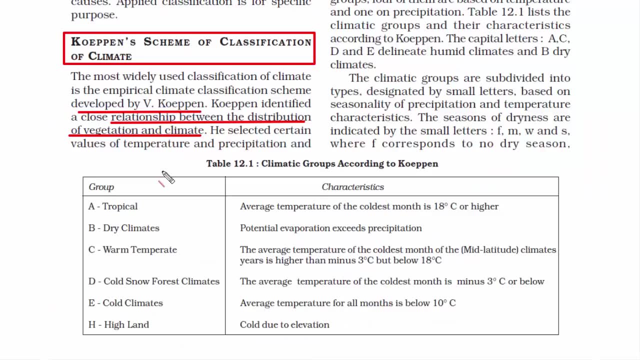 it showed close similarity with the existing vegetation, if i have to say it in a simple way. basically, he looked at the trees and plants of a particular region and then he figured out the relationship between the vegetation and the climate of that region by finding a close relationship between these two. he created a chart which categorized the climate of the region and 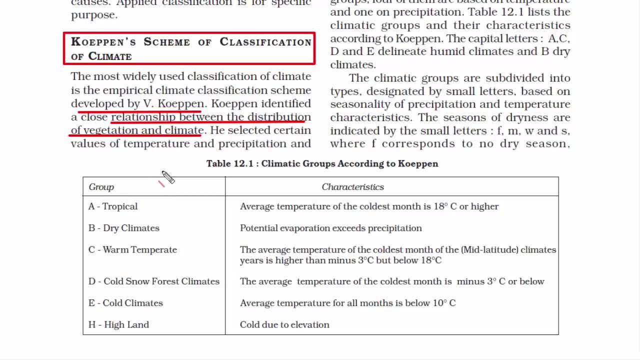 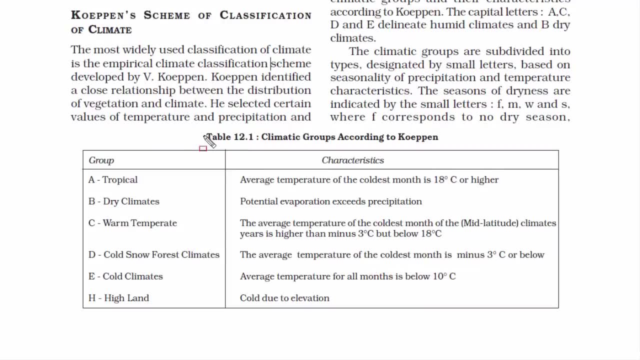 which categorizes different climates in groups, along with their characteristic traits. for categorizing climates in groups, he used capital and small letters. i'll show you the table. on the left column you can see how the capital letters a, b, c, d, e, h have been used to denote climatic groups. 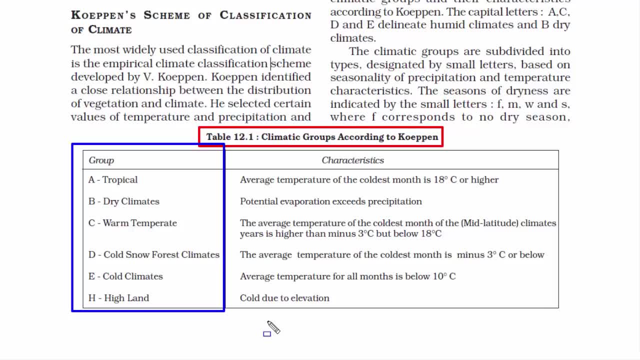 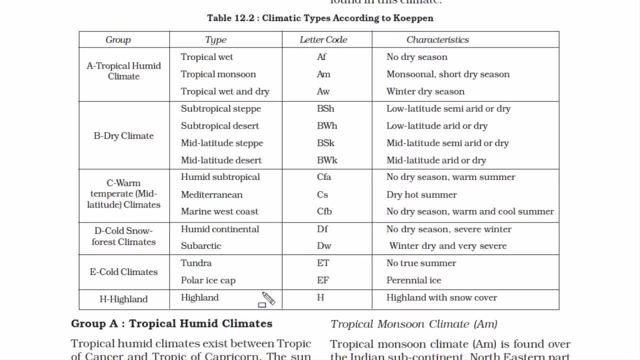 then, on the right column, you can see the respective characteristics. i want you to pause the video and quickly take a look at this table and, don't worry, i'll explain each of these groups in detail. now have a look at this table. the left column is exactly the same, but there are two new columns. 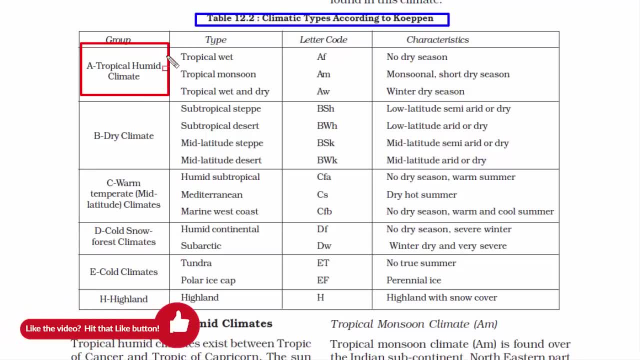 which denote the type and the letter codes. for example, group a is tropical humid climate. under this there are three subdivision or types. they are tropical wet, tropical monsoon and tropical wet and dry. and then you have the letter code which represents the subdivision of climates, and on the extreme right column we have the characteristics of the respective climatic groups. 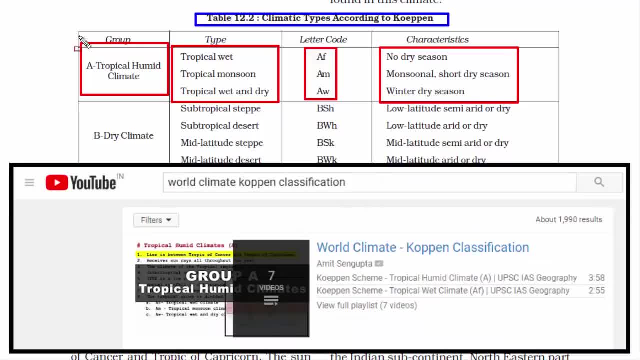 now i have made a separate playlist consisting of short videos on these individual climatic groups. these short videos will come handy and i have explained almost everything about these individual climatic groups in these videos. i'll put the link of the playlist in the description, or you could simply search for world climate coupon classification and you will find the. 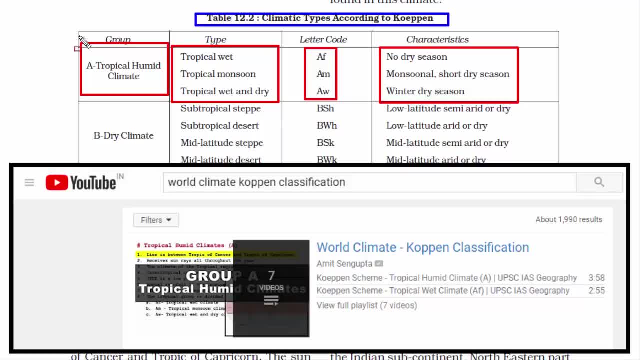 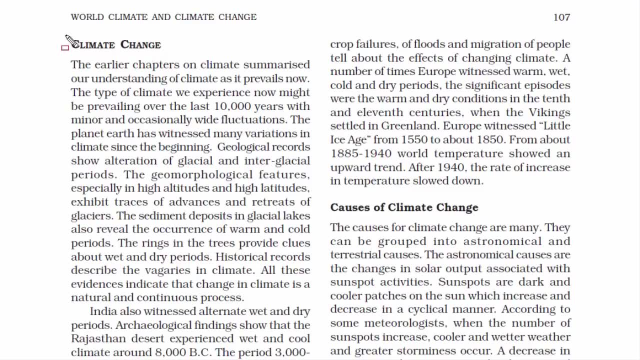 playlist that i'm talking about, so don't forget to check out the playlist. it's an important topic of this chapter, so go to the link and have a look at it. let's go to the link and have a look at it. to the link and have a look at it. let's go to the next topic: climate change. 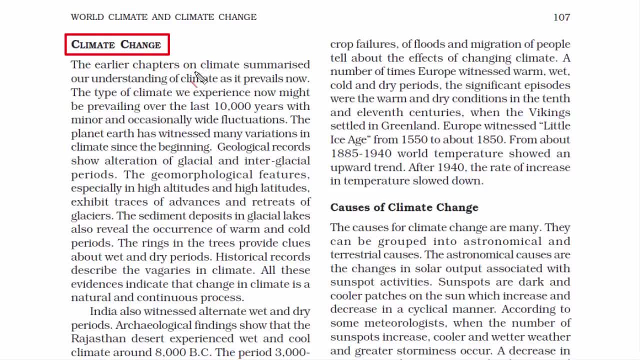 let's go to the next topic: climate change. let's go to the next topic: climate change. before we go much deeper into this topic, before we go much deeper into this topic, before we go much deeper into this topic, i would like to first tell you the. i would like to first tell you the. 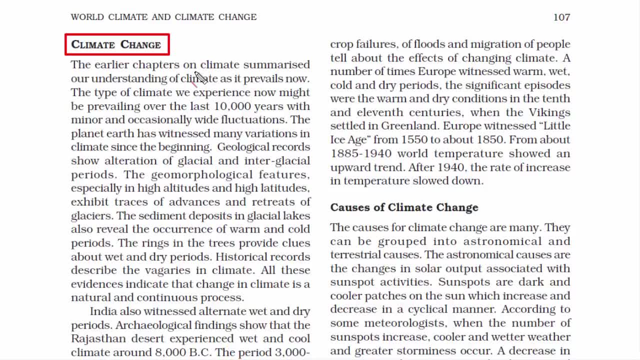 i would like to first tell you the difference between weather and climate, difference between weather and climate, difference between weather and climate. the main difference between the two is the main difference between the two is: the main difference between the two is that weather changes on day-to-day basis. 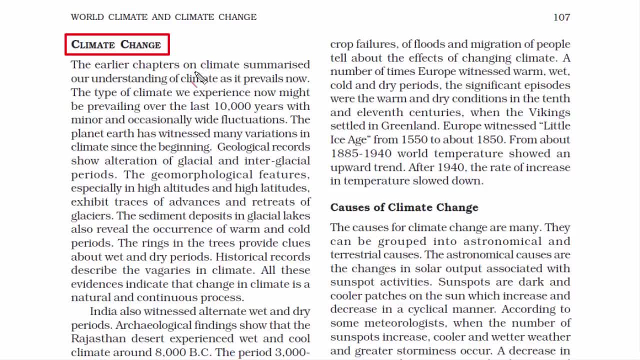 that weather changes on day-to-day basis, that weather changes on day-to-day basis and climate does not change for a longer and climate does not change for a longer and climate does not change for a longer period of time, period of time, period of time. so the key element here is the measure of 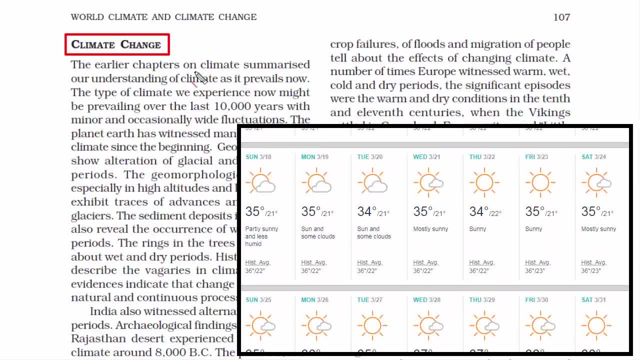 so the key element here is the measure of. so the key element here is the measure of time: time time weather is recorded and observed over. a weather is recorded and observed over. a weather is recorded and observed over a short period of time, short period of time. short period of time and climate is how the overall atmosphere 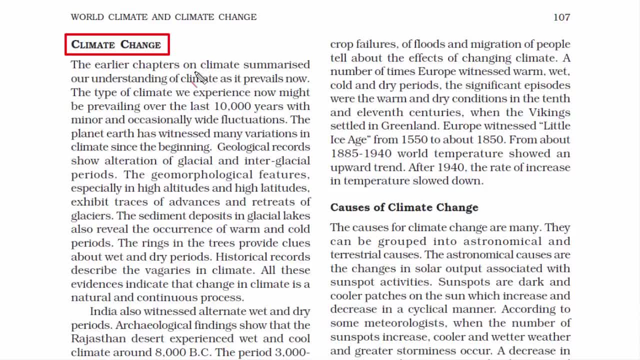 and climate is how the overall atmosphere and climate is how the overall atmosphere behaves over a long period of time, behaves over a long period of time, behaves over a long period of time. now that you know the difference between, now that you know the difference between, now that you know the difference between weather and climate, 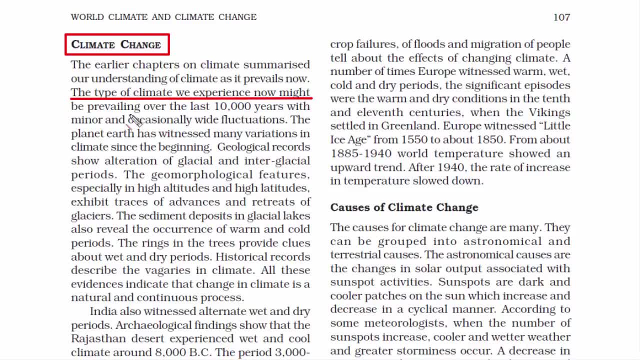 weather and climate. weather and climate here. it says the type of climate we here. it says the type of climate we here. it says the type of climate we experience now might be prevailing over experience now might be prevailing over. experience now might be prevailing over the last 10 000 years. 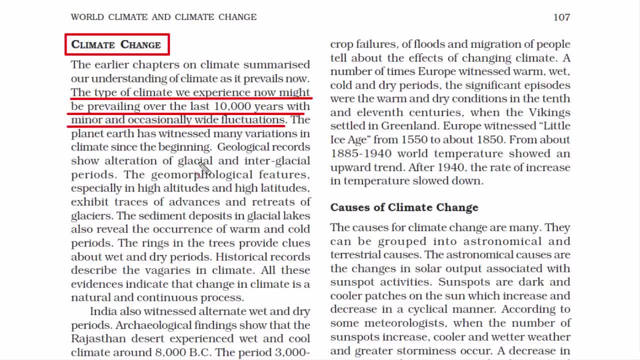 the last 10 000 years, the last 10 000 years with minor fluctuations. i think you can with minor fluctuations, i think you can with minor fluctuations. i think you can easily understand this line, easily understand this line. easily understand this line because, practically, if you see in the 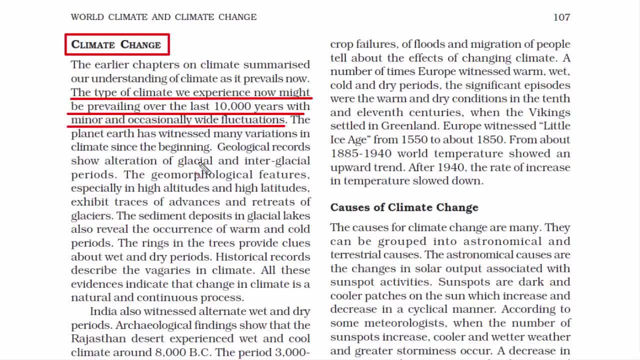 because, practically, if you see in the, because, practically, if you see, in the last 10 000 years, last 10 000 years, last 10 000 years, there hasn't been any major, there hasn't been any major, there hasn't been any major physiographical or geological changes. 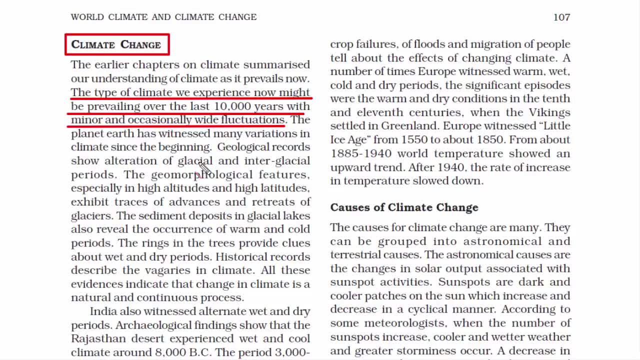 physiographical or geological changes. physiographical or geological changes: when we say 10 000 years ago we are. when we say 10 000 years ago we are. when we say 10 000 years ago, we are somewhat referring to 8 000 to 7 000 bce. 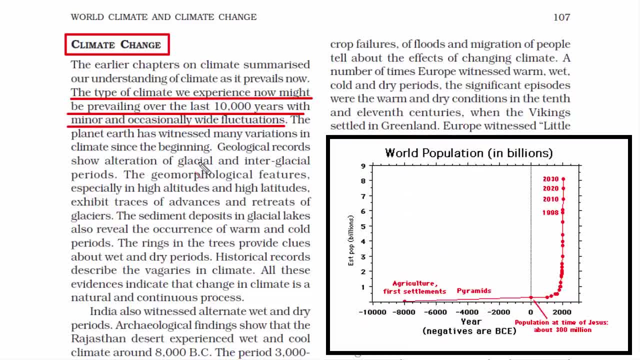 somewhat referring to 8 000 to 7 000 bce, somewhat referring to 8 000 to 7 000 bce. during this time, agriculture was widely. during this time, agriculture was widely. during this time, agriculture was widely practiced, practiced, practiced. of course, the human population was only 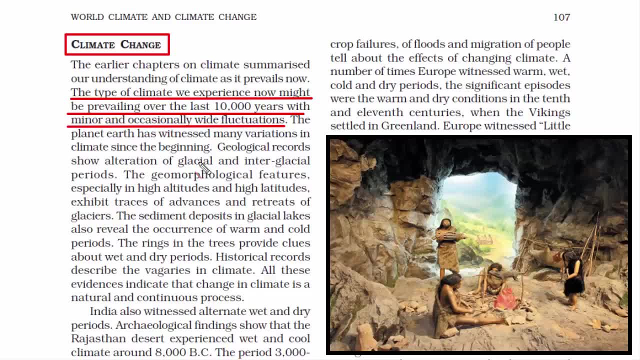 of course the human population was only. of course the human population was only few millions. they mostly lived in caves. few millions, they mostly lived in caves. few millions, they mostly lived in caves and all their food came from wild plants and all their food came from wild plants. 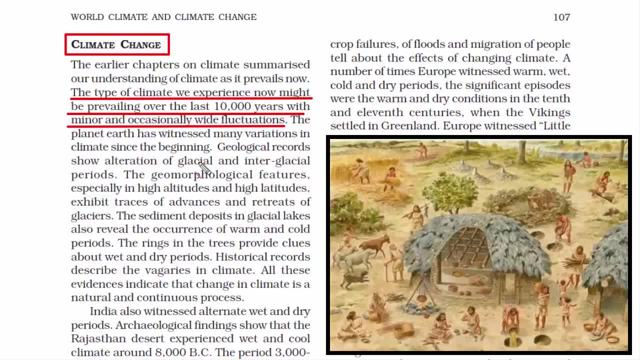 and all their food came from wild plants and animals and animals and animals. then later humans started settling down, then later humans started settling down, then later humans started settling down and in these settlements they and in these settlements they and in these settlements they domesticated some of those animals. 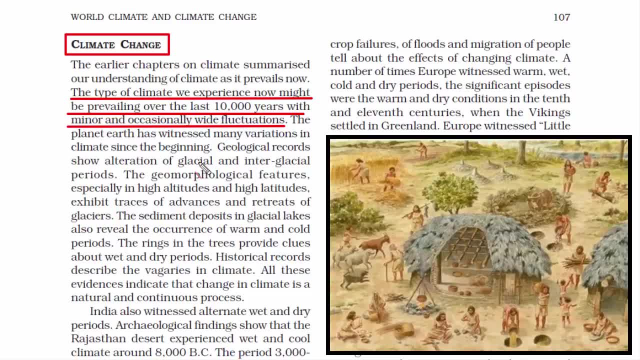 domesticated some of those animals, domesticated some of those animals and started off with agriculture to meet and started off with agriculture to meet and started off with agriculture to meet their food demands, their food demands, their food demands. now you can easily imagine that 10 000. 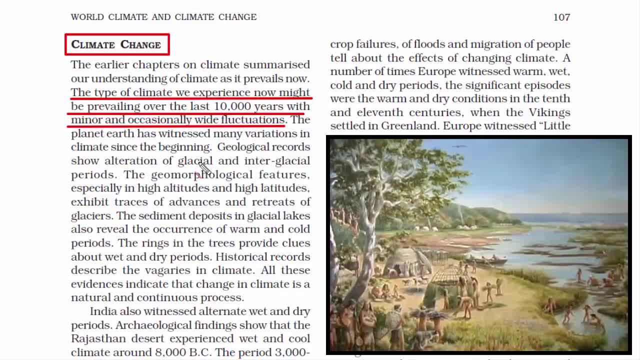 now. you can easily imagine that 10 000 now. you can easily imagine that 10 000 years ago, years ago, years ago, humans chose a particular place as their humans chose a particular place as their humans chose a particular place as their settlement, settlement, settlement, then obviously their primary. 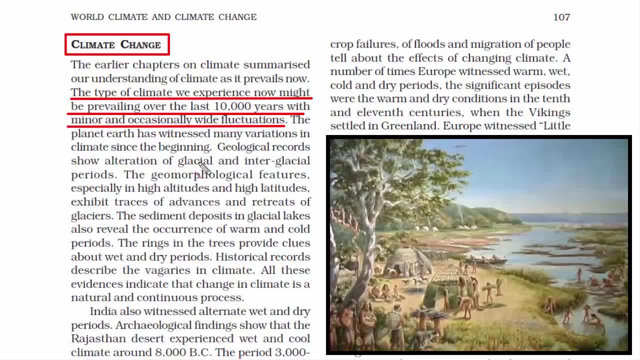 then obviously their primary, then obviously their primary consideration consideration consideration was regarding climate and weather. they was regarding climate and weather. they was regarding climate and weather. they must have noticed the weather and must have noticed the weather and must have noticed the weather and climatic pattern. climatic pattern. 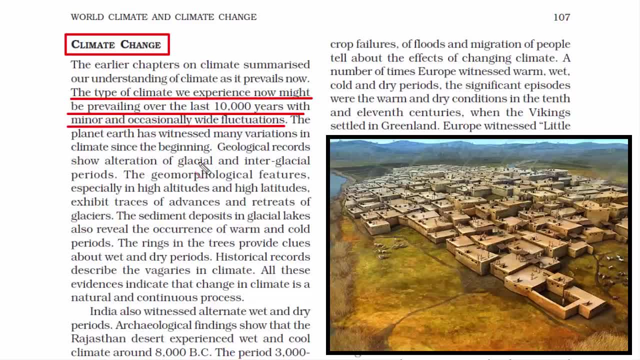 climatic pattern, which definitely formed the basis of which definitely formed the basis of which definitely formed the basis of their settlement, their settlement, their settlement and those settlements grew over time and those settlements grew over time and those settlements grew over time into larger cities and towns, into larger cities and towns. 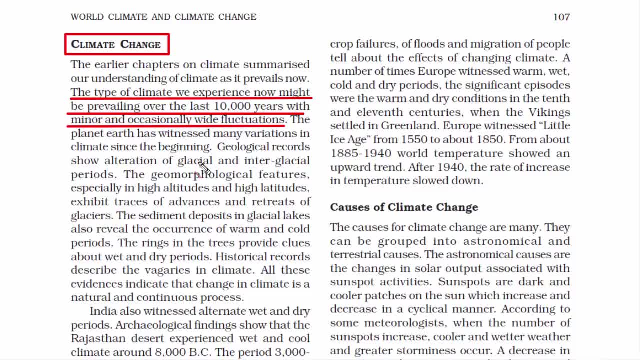 into larger cities and towns. you see, broadly speaking the climate, did you see, broadly speaking the climate? did you see, broadly speaking, the climate did not change, except for few minor not change, except for few minor not change, except for few minor fluctuations. because if there was any fluctuations, because if there was any, 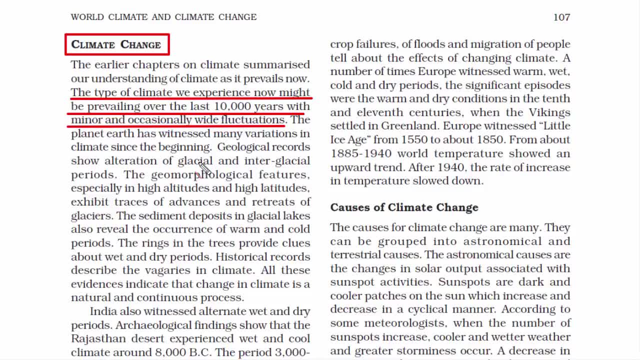 fluctuations, because if there was any major climatic fluctuation, then early major climatic fluctuation, then early major climatic fluctuation, then early humans would have left those places and humans would have left those places and humans would have left those places. and today the climate is slightly different. 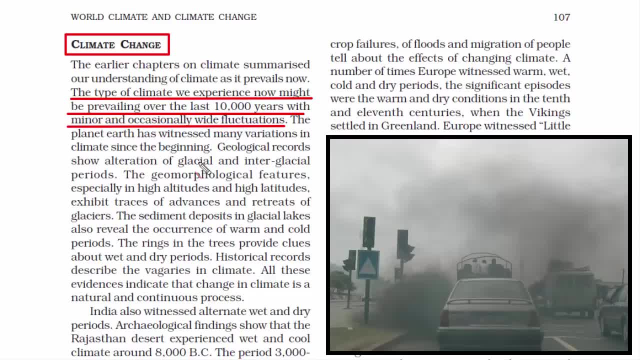 today, the climate is slightly different. today, the climate is slightly different, and these minor fluctuations are due to: and these minor fluctuations are due to, and these minor fluctuations are due to burning of fossil fuels, burning of fossil fuels, burning of fossil fuels. in other words, we inconsiderably pollute. 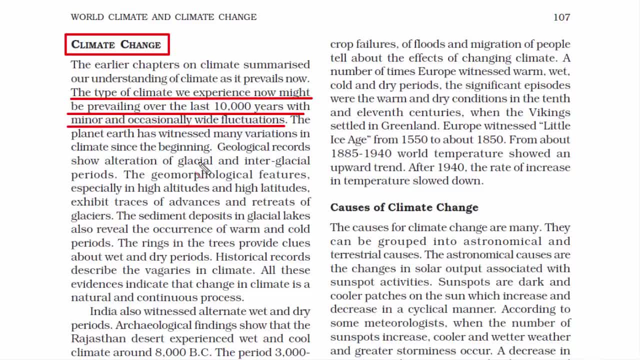 in other words, we inconsiderably pollute. in other words, we inconsiderably pollute the environment and generate more waste, the environment and generate more waste, the environment and generate more waste. so, yeah, this line absolutely makes sense. so yeah, this line absolutely makes sense. so, yeah, this line absolutely makes sense regarding climate, 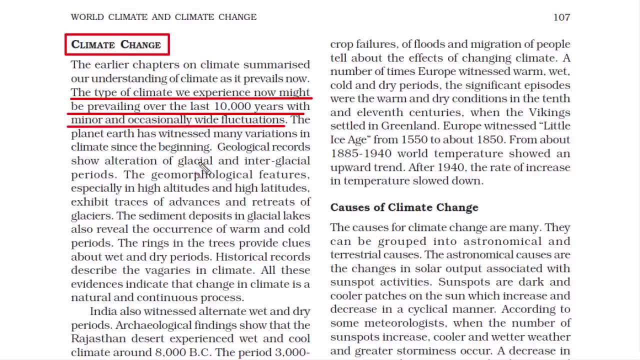 regarding climate. regarding climate, one more thing that you will hear a lot. one more thing that you will hear a lot. one more thing that you will hear a lot these days is about climate change. these days is about climate change. these days is about climate change, and climate change is real. in fact. the 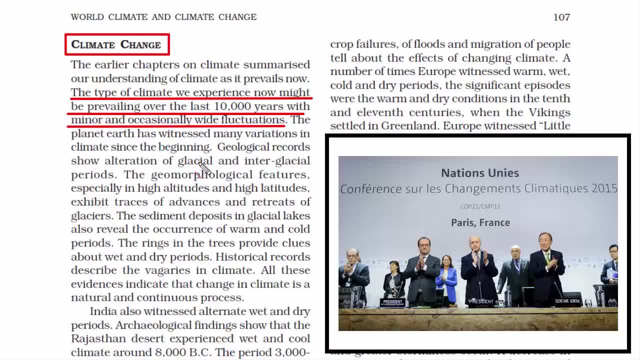 and climate change is real, in fact, the and climate change is real, in fact, the objective of 2015 paris agreement on a objective of 2015 paris agreement on a objective of 2015 paris agreement on a climate change is to limit the overall climate change is to limit the overall. 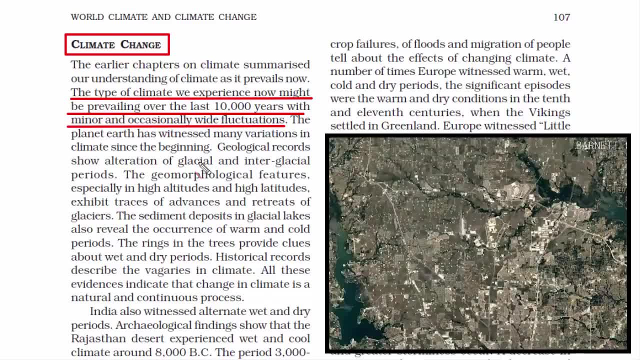 climate change is to limit the overall temperature of the earth, temperature of the earth, temperature of the earth. now climate change is a natural, and now climate change is a natural, and now climate change is a natural and continuous process, continuous process, continuous process, but then in recent times it has been: 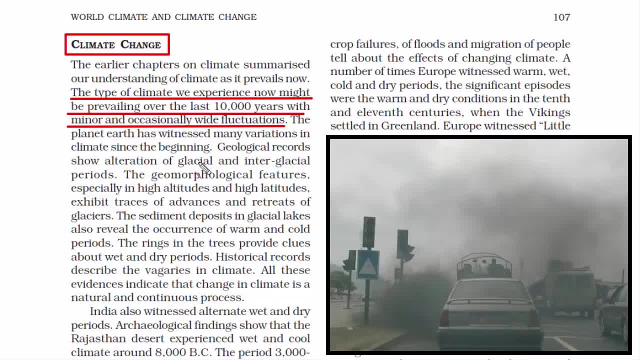 but then in recent times it has been, but then in recent times it has been more because of human activities, more because of human activities, more because of human activities. otherwise, since the beginning of time, otherwise, since the beginning of time, otherwise, since the beginning of time, the change in climate is a natural and 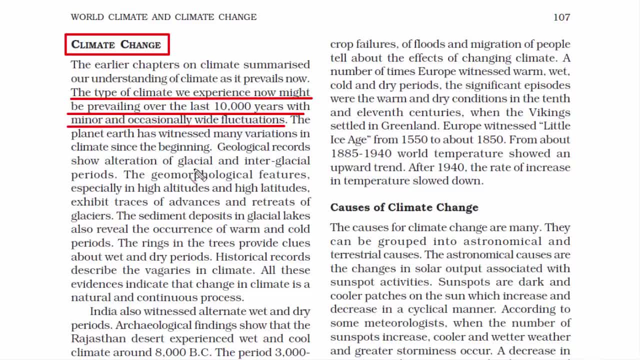 the change in climate is a natural and the change in climate is a natural and continuous process, continuous process, continuous process, and there's a lot of evidence that and there's a lot of evidence that and there's a lot of evidence that proves this theory. if you go to the 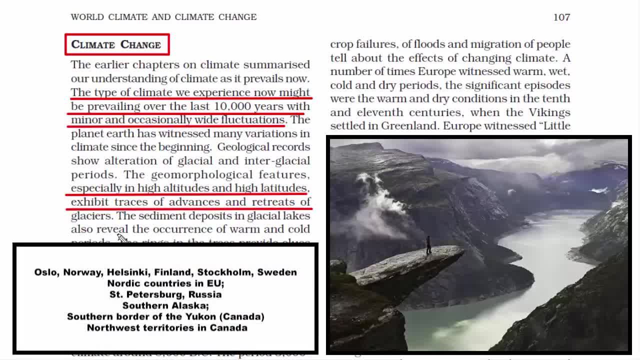 proves this theory. if you go to the proves this theory. if you go to the higher latitude areas- higher latitude areas, higher latitude areas- there you will find steep landform and there you will find steep landform. and there you will find steep landform, and mostly it's due to the melting and 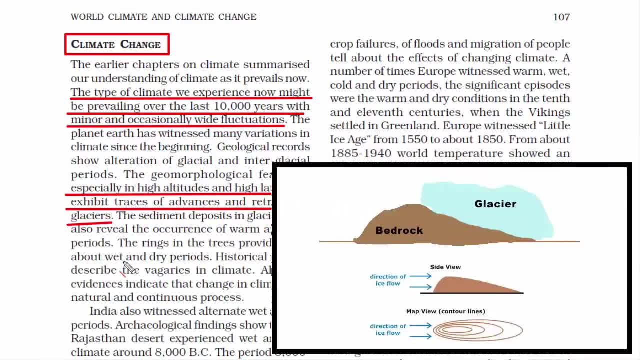 mostly it's due to the melting and mostly it's due to the melting and movement of glaciers: movement of glaciers, movement of glaciers. when temperature changed with time, when temperature changed with time, when temperature changed with time, naturally the glacier started moving. naturally the glacier started moving. naturally the glacier started moving. when glacier melts, it begins melting. 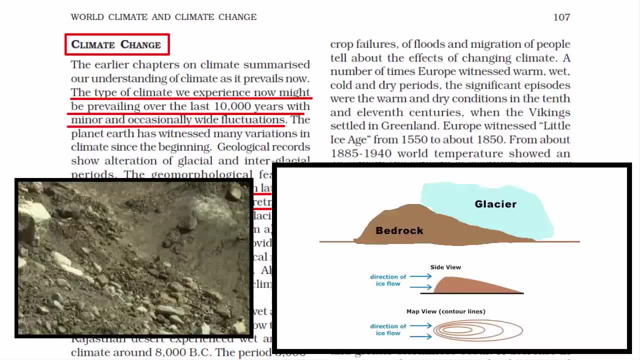 when glacier melts, it begins melting. when glacier melts, it begins melting from lower end, and that makes the from lower end, and that makes the from lower end, and that makes the glacier move towards one direction. which glacier move towards one direction, which glacier move towards one direction, which eventually creates friction for the land. 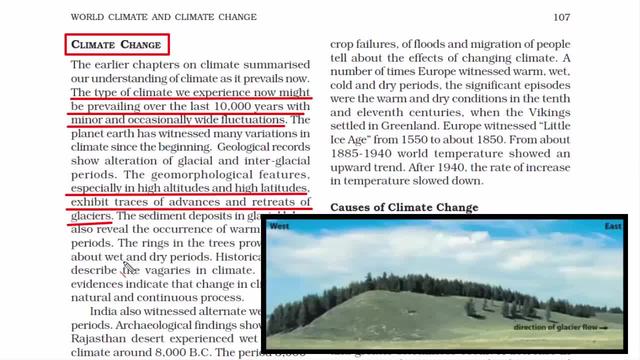 eventually creates friction for the land, eventually creates friction for the land below the glacier to move accordingly below the glacier, to move accordingly below the glacier, to move accordingly. that's how steep landforms were formed. that's how steep landforms were formed. that's how steep landforms were formed. and if you look at the sediment deposits, 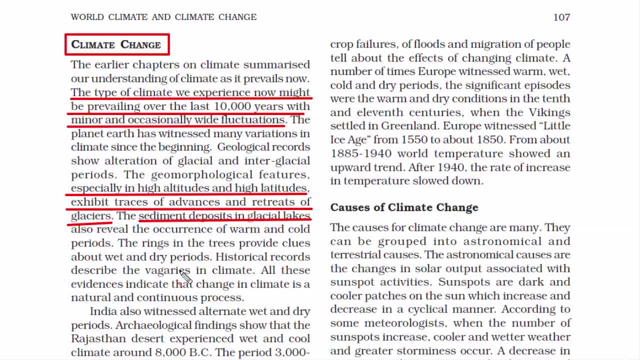 and if you look at the sediment deposits, and if you look at the sediment deposits in glacial lakes, it gives us the in glacial lakes, it gives us the in glacial lakes, it gives us the evidence of warm and cold periods. evidence of warm and cold periods. 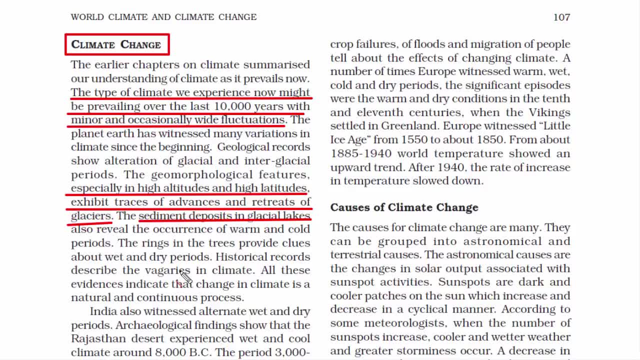 evidence of warm and cold periods because glacial lakes are formed due to. because glacial lakes are formed due to. because glacial lakes are formed due to melting of glaciers, melting of glaciers, melting of glaciers. so basically, a glacier is an ice sheet. so basically, a glacier is an ice sheet. 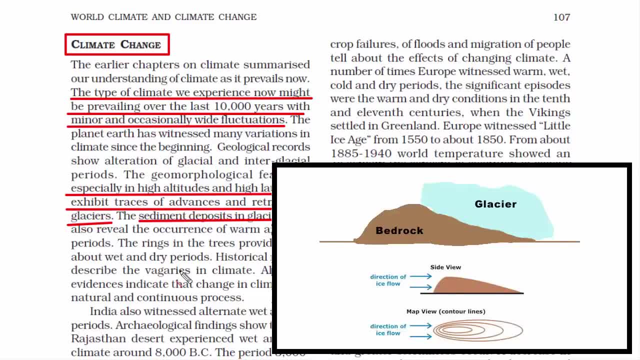 so basically, a glacier is an ice sheet that lies on a bedrock. when glacier that lies on a bedrock. when glacier that lies on a bedrock, when glacier melts, it creates a friction on the melts. it creates a friction on the melts. it creates a friction on the underlying bedrock. the bedrock starts to. 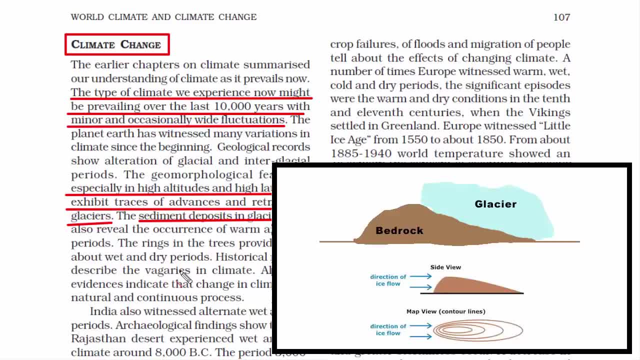 underlying bedrock. the bedrock starts to underlying bedrock. the bedrock starts to erode into tiny sediments that later on erode into tiny sediments that later on erode into tiny sediments that later on gets deposited in glacial lakes. gets deposited in glacial lakes. 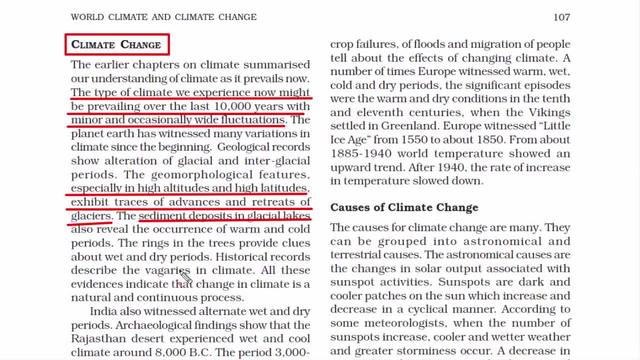 gets deposited in glacial lakes. so you see, it's a natural mechanism that. so you see, it's a natural mechanism that. so you see, it's a natural mechanism that works when temperature is cool, works when temperature is cool, works when temperature is cool and eventually gets warm. and finally, if 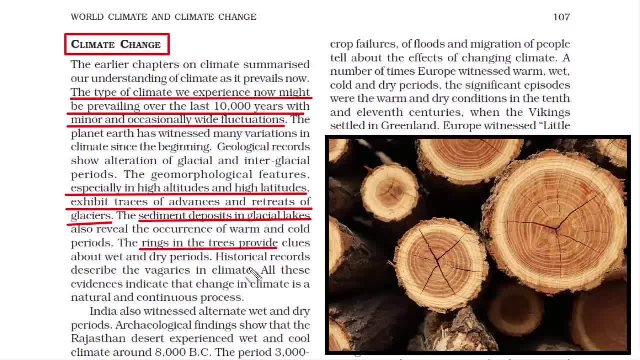 and eventually gets warm, and finally, if and eventually gets warm. and finally, if you look at the, you look at the, you look at the rings in a tree. it tells us a lot about rings in a tree. it tells us a lot about rings in a tree. it tells us a lot about wet and dry periods. 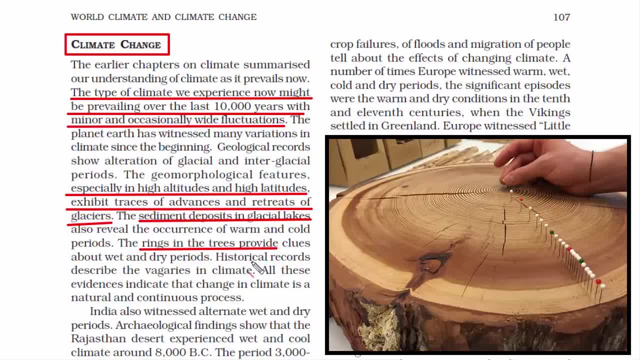 wet and dry periods. wet and dry periods, i mean there's a scientific method of. i mean there's a scientific method of. i mean there's a scientific method of looking at these three rings, looking at these three rings, looking at these three rings, and that can tell you the exact year. 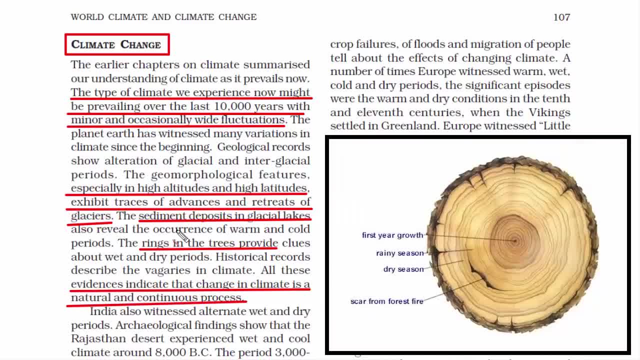 and that can tell you the exact year, and that can tell you the exact year when they were formed. when they were formed, when they were formed, and by looking at the size of the ring, and by looking at the size of the ring, and by looking at the size of the ring, we can figure out whether it was cold. 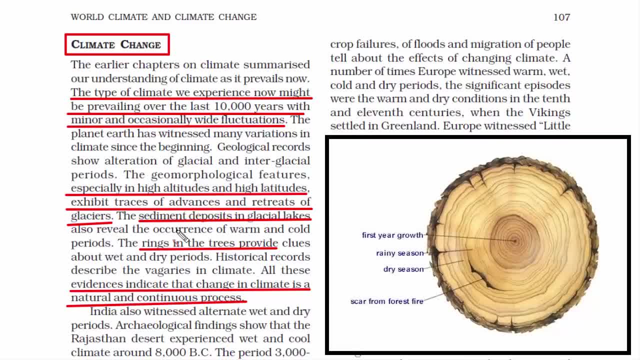 we can figure out whether it was cold. we can figure out whether it was cold year or warm year year or warm year, year or warm year. during cold years the ring is bigger and during cold years the ring is. during cold years the ring is. during cold years, the ring is comparatively smaller. 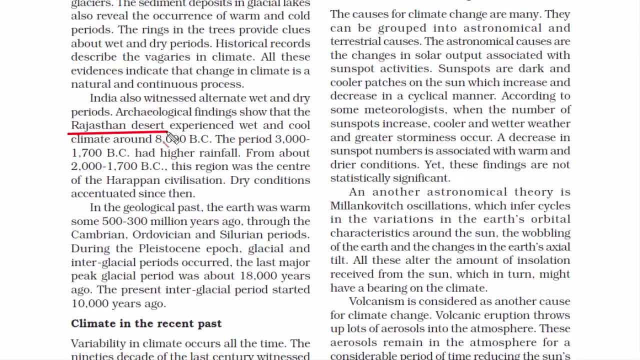 comparatively smaller, comparatively smaller. if you want to know an example of, if you want to know an example of, if you want to know an example of climate change which is related to our climate change, which is related to our climate change, which is related to our country, india. 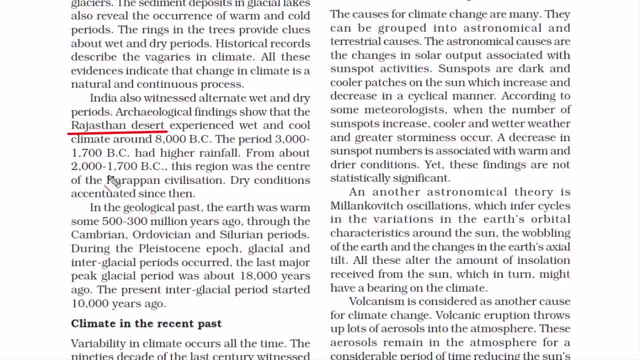 country india, country india. so here they have very nicely mentioned, so here they have very nicely mentioned, so here they have very nicely mentioned about the rajasthan desert, about the rajasthan desert, about the rajasthan desert around 10 000 years ago. that is around around 10 000 years ago. that is around 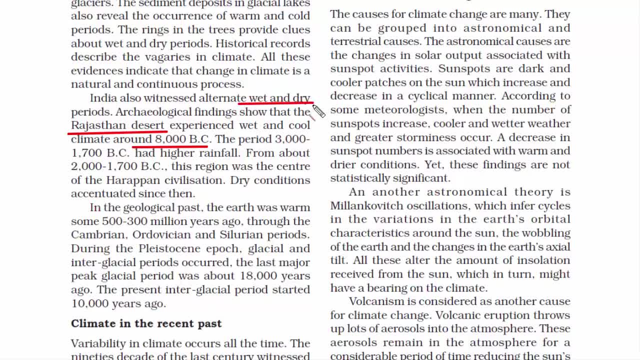 around 10 000 years ago, that is, around 8 000 bce- 8 000 bce- 8 000 bce. rajasthan experienced wet and cool rajasthan experienced wet and cool. rajasthan experienced wet and cool climate. that means once upon a time. it. 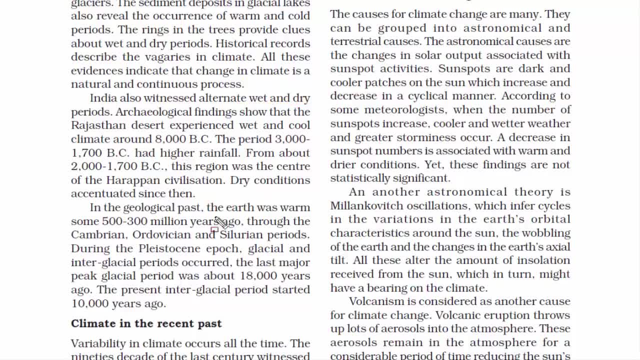 climate. that means once upon a time. it climate. that means once upon a time. it rained heavily in rajasthan desert, rained heavily in rajasthan desert, rained heavily in rajasthan desert, and it was all so cool, but then during. and it was all so cool, but then during. 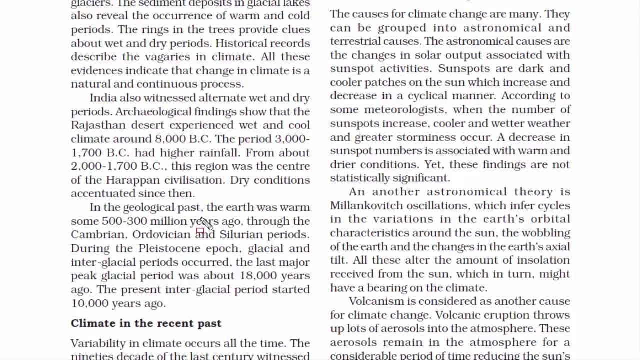 and it was all so cool. but then, during night time, anyhow, deserts are cold right. night time, anyhow, deserts are cold right. night time, anyhow, deserts are cold right. so what is interesting is knowing that. so what is interesting is knowing that. so what is interesting is knowing that it rained heavily once upon a time in 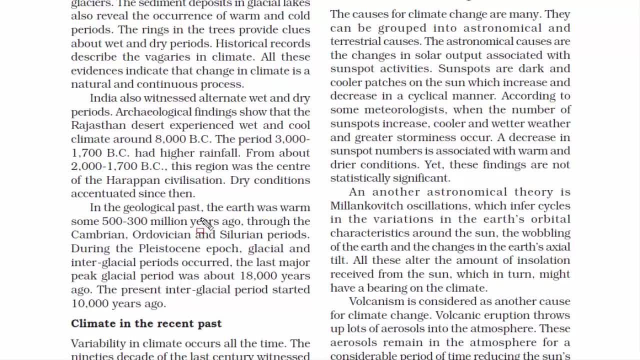 it rained heavily once upon a time in. it rained heavily once upon a time in the desert of rajasthan, the desert of rajasthan, the desert of rajasthan. now, if you have a general curiosity, now, if you have a general curiosity, now, if you have a general curiosity about how did the sand in the desert? 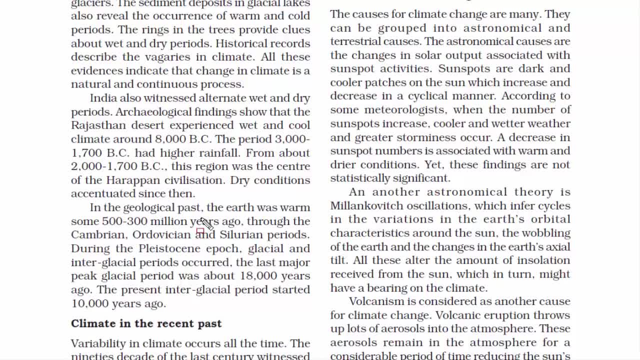 about how did the sand in the desert, about how did the sand in the desert appear? i mean from where it came. how did appear? i mean from where it came. how did appear? i mean from where it came. how did it all happen? then you need to it all happen, then you need to. 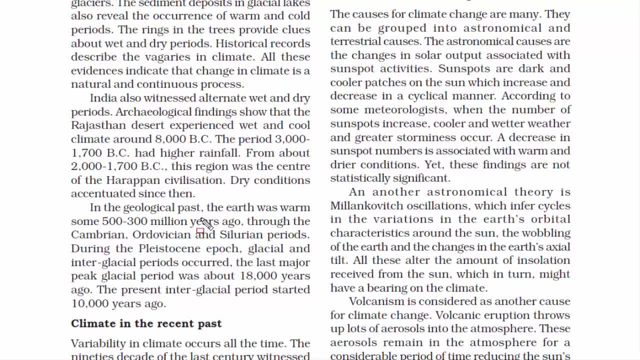 it all happen, then you need to understand that there can be two. understand that there can be two, understand that there can be two possible reason: either the desert possible reason, either the desert possible reason. either the desert appeared due to movement of earth's huge, appeared due to movement of earth's huge. 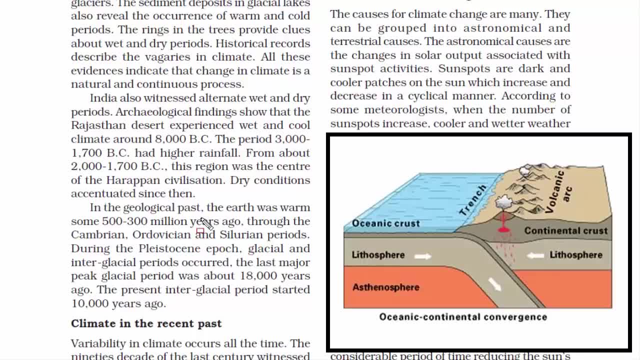 appeared due to movement of earth's huge land plates. i'm talking about the land plates. i'm talking about the land plates. i'm talking about the movement of earth's lithosphere, because movement of earth's lithosphere, because movement of earth's lithosphere, because of that, massive geological changes take 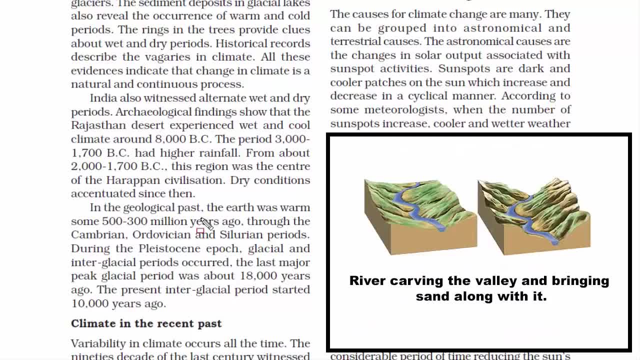 of that massive geological changes take, of that massive geological changes take place. so that place, so that place, so that that could be one possible reason, or the that could be one possible reason, or the that could be one possible reason, or the second reason could be. second reason could be. 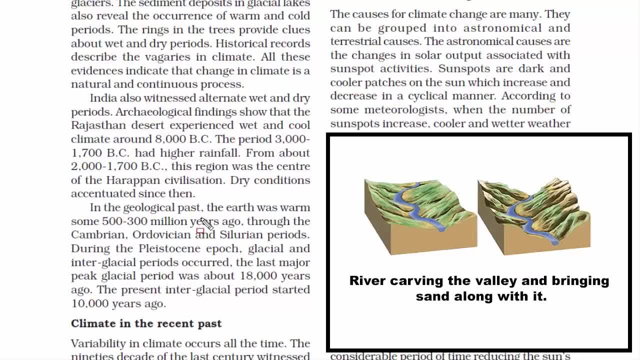 second reason could be: maybe this sand in the desert came, or maybe this sand in the desert came, or maybe this sand in the desert came or appeared because of the appeared, because of the appeared, because of the rivers or streams that must have eroded, rivers or streams that must have eroded. 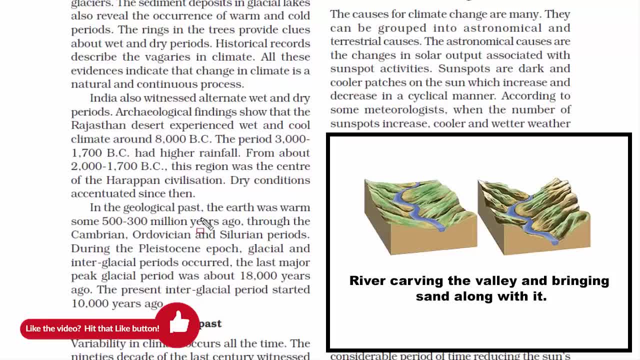 rivers or streams that must have eroded rocks into tiny sediments, rocks into tiny sediments, rocks into tiny sediments. or the river might have carried the, or the river might have carried the, or the river might have carried the sediments from one place to another. 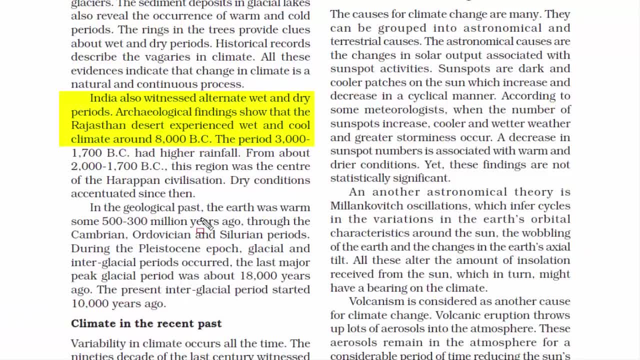 sediments from one place to another, sediments from one place to another. so these are the two possible reason. so these are the two possible reason. so these are the two possible reason. and now, when we read here that the. and now when we read here that the. 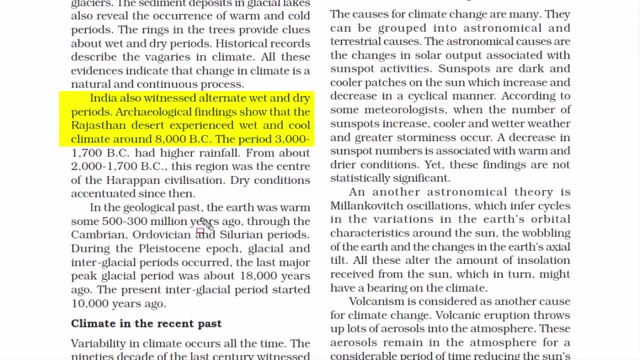 and now when we read here that the rajasthan desert experienced wet and rajasthan desert experienced wet and rajasthan desert experienced wet and cool climate around 10 000 years ago. cool climate around 10 000 years ago. cool climate around 10 000 years ago, then the possible reason is maybe at 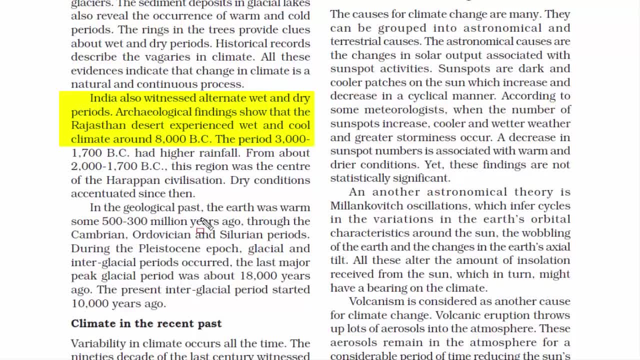 then the possible reason is: maybe at then. the possible reason is maybe at that time, that time, that time, massive portion of the rajasthan desert, massive portion of the rajasthan desert, massive portion of the rajasthan desert, must have been under a river, must have been under a river. 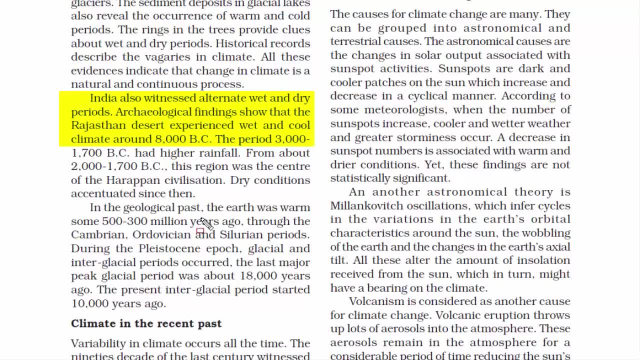 must have been under a river. well, if that's the case, then the desert. well, if that's the case, then the desert. well, if that's the case, then the desert. we see today, once upon time was covered. we see today, once upon time was covered. we see today, once upon time was covered with green trees. 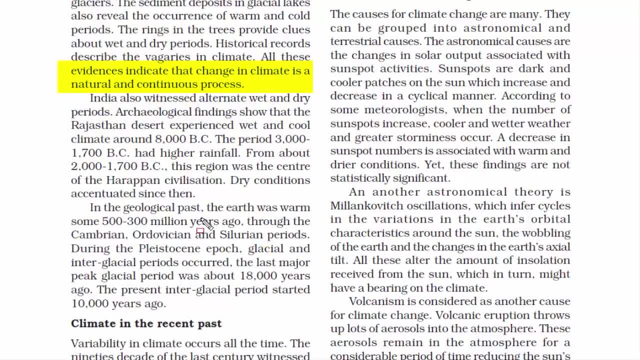 with green trees, with green trees with this example, we understand that, since, with this example, we understand that, since, with this example, we understand that, since the beginning of time, the change in the beginning of time, the change in the beginning of time, the change in climate is a natural and continuous 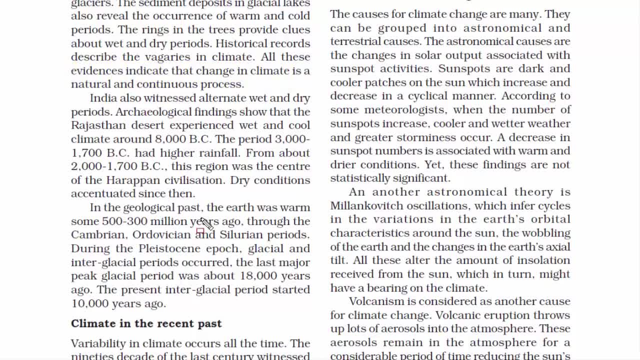 climate is a natural and continuous climate is a natural and continuous process process, process and the type of climate we experience now and the type of climate we experience now and the type of climate we experience now might be prevailing over the last 10 000, might be prevailing over the last 10 000. 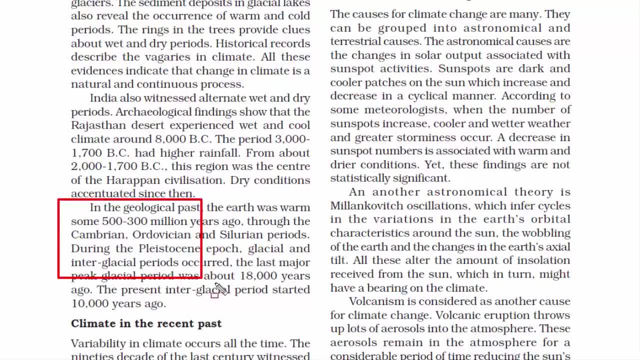 might be prevailing over the last 10 000 years with minor fluctuations, years with minor fluctuations, years with minor fluctuations. about this little paragraph. i'll make a about this little paragraph. i'll make a about this little paragraph. i'll make a separate video on earth's. 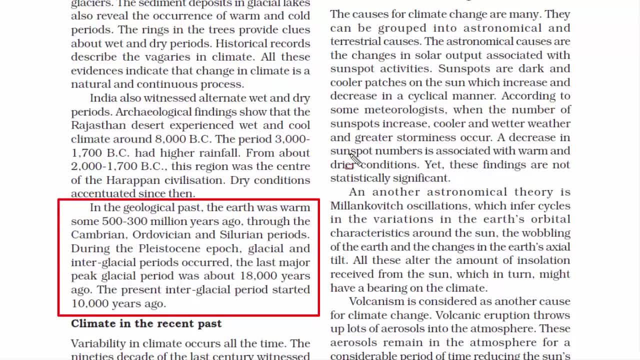 separate video on earth's, separate video on earth's geological time scale. in that i'll geological time scale, in that i'll geological time scale, in that i'll explain what the earth went through, explain what the earth went through, explain what the earth went through a different period of time, and it will 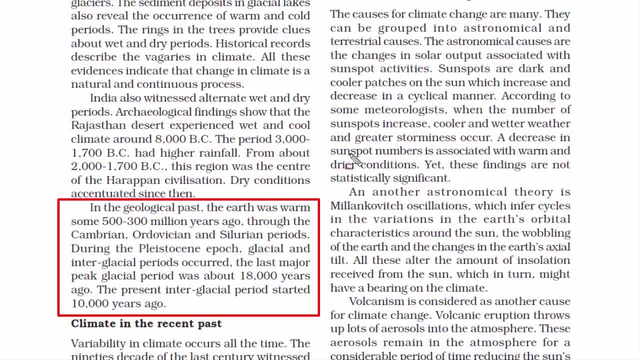 a different period of time, and it will a different period of time and it will give you a broad understanding about the, give you a broad understanding about the, give you a broad understanding about the earth's history with respect to time and earth's history with respect to time, and. 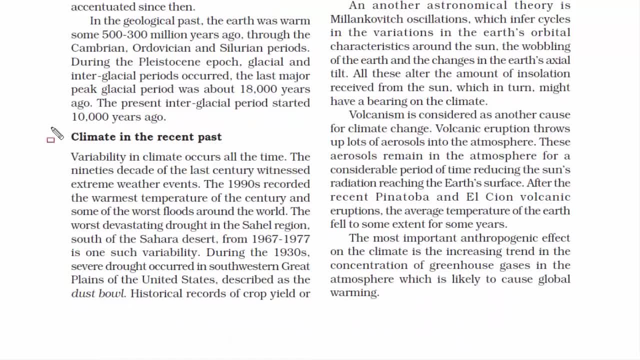 earth's history with respect to time and relationships of events. relationships of events. relationships of events. all right, let's go to the next topic. all right, let's go to the next topic. all right, let's go to the next topic. climate in the recent past- climate in the recent past. 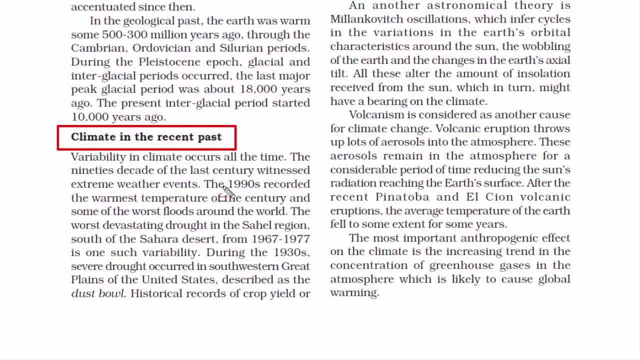 climate in the recent past. so recent past means 100 to 200 years from so. recent past means 100 to 200 years from so. recent past means 100 to 200 years from today today. today, i mean industrial revolution took place. i mean industrial revolution took place. 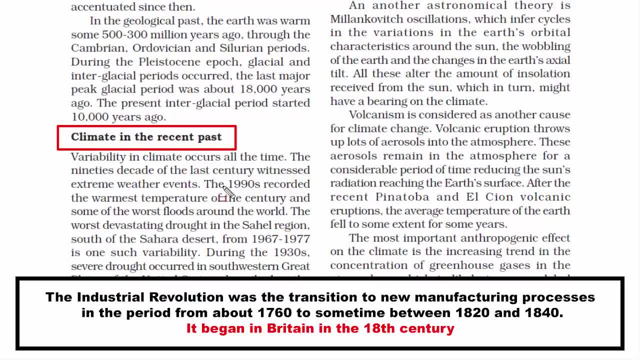 i mean industrial revolution took place in 19th century around 1880, in 19th century around 1880, in 19th century around 1880. since then, the earth's temperature, since then the earth's temperature, since then the earth's temperature readings have risen continuously. 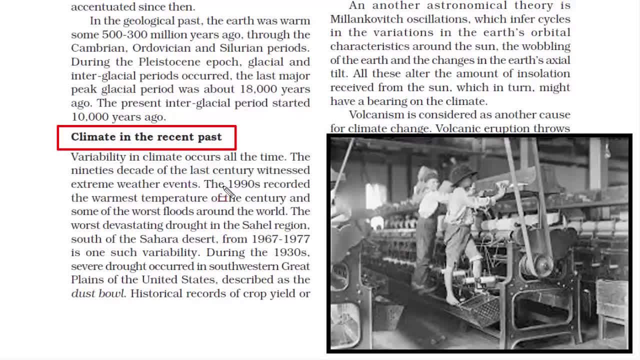 readings have risen continuously. readings have risen continuously. i mean no doubt that industrial. i mean no doubt that industrial. i mean no doubt that industrial revolution made life easier. but then we revolution made life easier. but then we revolution made life easier. but then we also need to look at the cost. 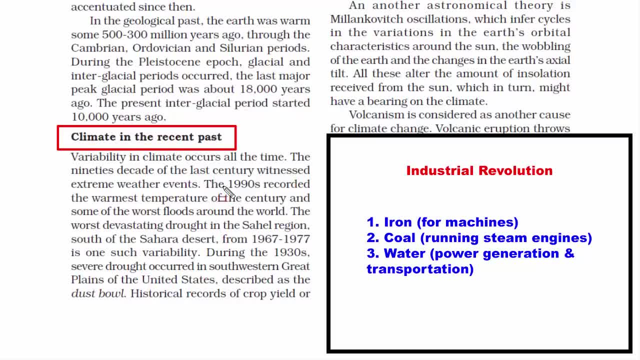 also need to look at the cost, also need to look at the cost. if you see industrial revolution was, if you see industrial revolution was, if you see industrial revolution was dependent on, dependent on dependent on three key natural resources. that is iron. three key natural resources. that is iron. 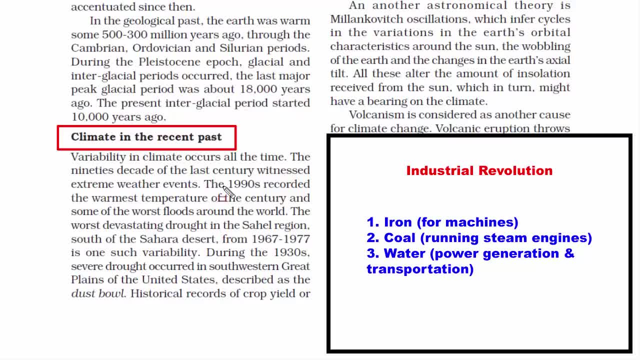 three key natural resources, that is, iron, coal and water. coal and water. coal and water- now. iron was used for machinery. water was now. iron was used for machinery. water was now. iron was used for machinery. water was used as a source of power. used as a source of power. 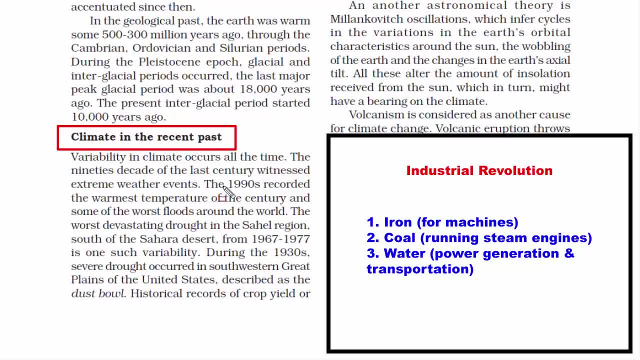 used as a source of power, and also as a mode of transportation, and, and also as a mode of transportation, and, and also as a mode of transportation. and then coal was used to power, then coal was used to power, then coal was used to power steam engines. you see, coal is a fossil. 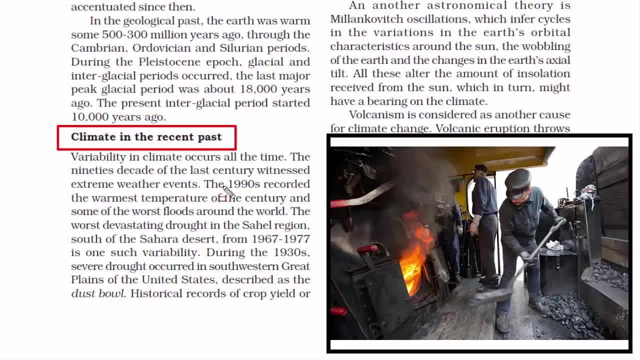 steam engines- you see, coal is a fossil. steam engines. you see, coal is a fossil fuel. steam engines and other kinds of fuel steam engines and other kinds of fuel steam engines and other kinds of machines of industrial revolution. machines of industrial revolution. machines of industrial revolution used cold as a fuel, now burning vast. 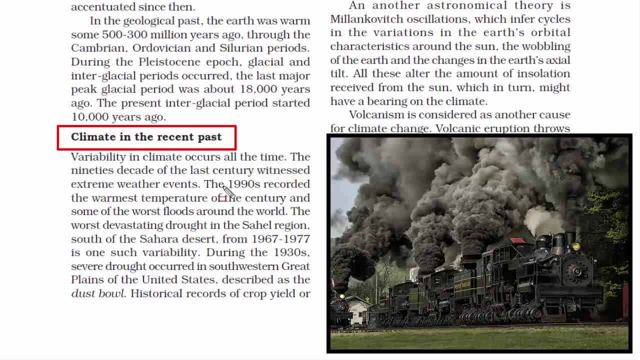 used cold as a fuel, now burning vast. used cold as a fuel, now burning vast quantities of quantities of quantities. of coal produced enormous amount of smoke. coal produced enormous amount of smoke. coal produced enormous amount of smoke and that led to air pollution and that led to air pollution. 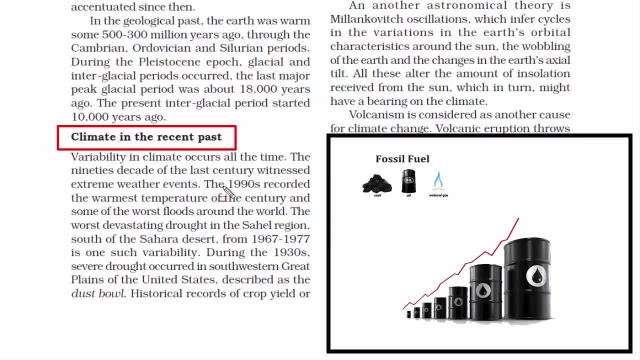 and that led to air pollution, and it even continues today, or maybe i'll, and it even continues today, or maybe i'll, and it even continues today, or maybe i'll go on to say that it is much more. go on to say that it is much more. 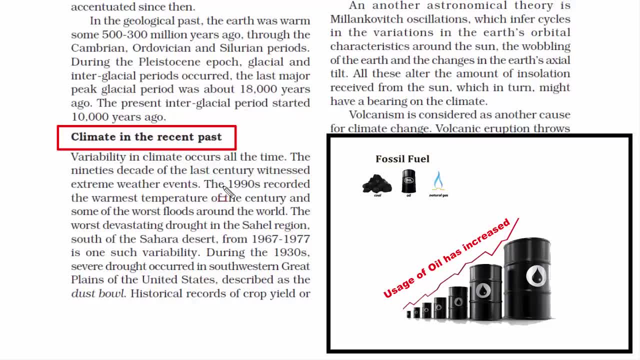 go on to say that it is much more today, today, today. so, in a nutshell, burning of fossil fuels. so, in a nutshell, burning of fossil fuels. so, in a nutshell, burning of fossil fuels is one major contributor towards, is one major contributor towards, is one major contributor towards global warming and climate change. 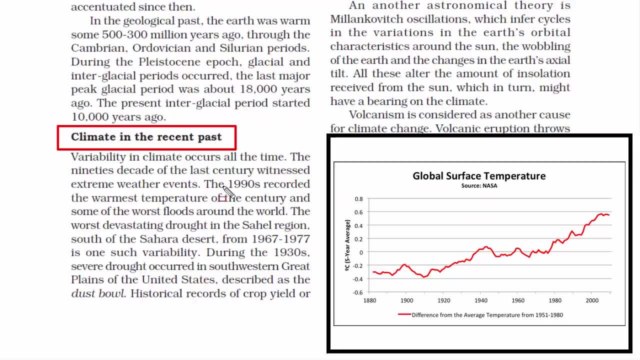 global warming and climate change. global warming and climate change: one degree rise in the surface. one degree rise in the surface, one degree rise in the surface. temperature of the earth is actually a temperature of the earth. is actually a temperature of the earth is actually a matter of concern, because even one 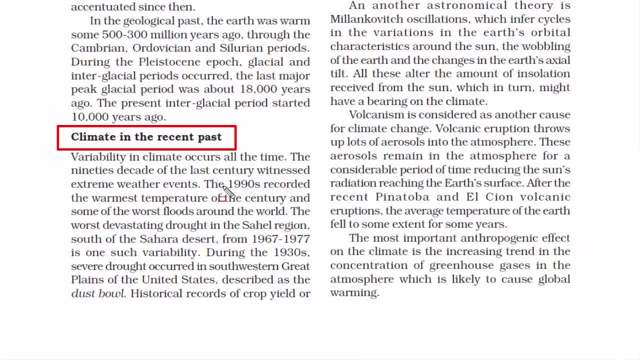 matter of concern, because even one matter of concern, because even one degree rise in temperature is enough to degree rise in temperature is enough to degree rise in temperature is enough to warm all the ocean land and the warm, all the ocean land and the warm, all the ocean land and the atmosphere. 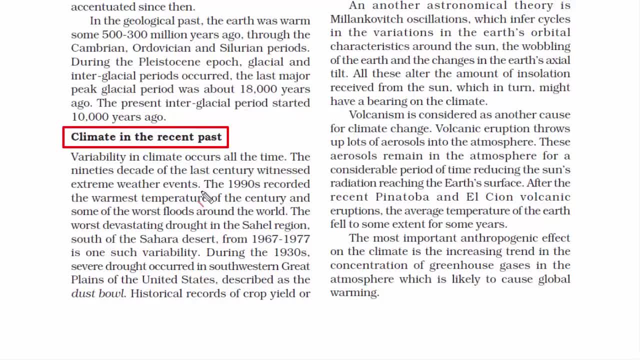 atmosphere, atmosphere. so that was a brief synopsis on climate. so that was a brief synopsis on climate. so that was a brief synopsis on climate change since the industrial revolution. change since the industrial revolution. change since the industrial revolution. however, i want you to pause the video. or. however, i want you to pause the video, or 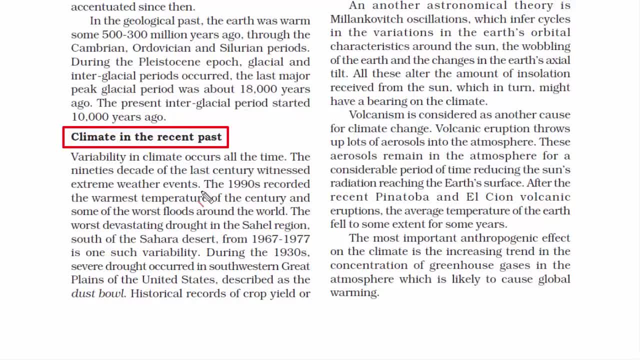 however, i want you to pause the video or maybe look at your textbook and go. maybe look at your textbook and go. maybe look at your textbook and go through these dates and their through these dates and their through these dates and their respective events that were recorded. respective events that were recorded. 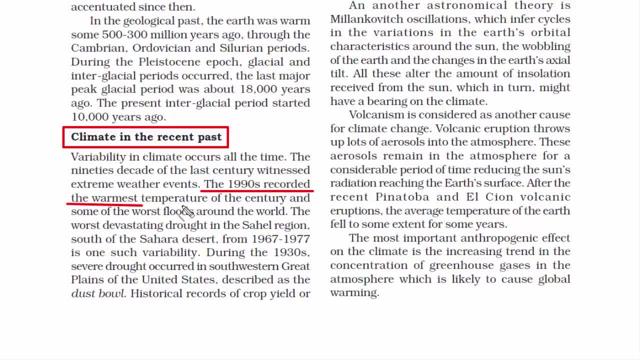 respective events that were recorded. so here it says: the 1990s recorded the. so here it says the 1990s recorded the. so here it says: the 1990s recorded the warmest temperature of the century, warmest temperature of the century, warmest temperature of the century and some of the worst floods around the. 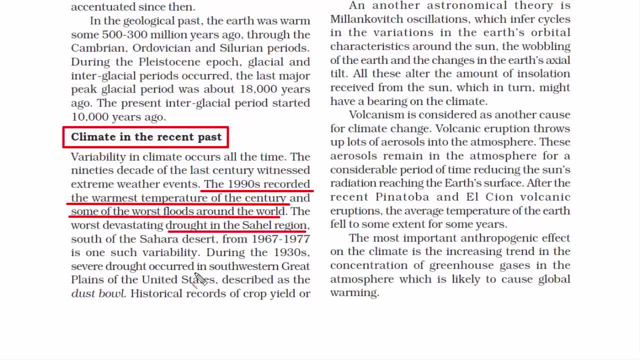 and some of the worst floods around the and some of the worst floods around the world took place during that time. world took place during that time. world took place during that time then. one of the worst drought that then. one of the worst drought that then. one of the worst drought that occurred during 1960s and 70s. 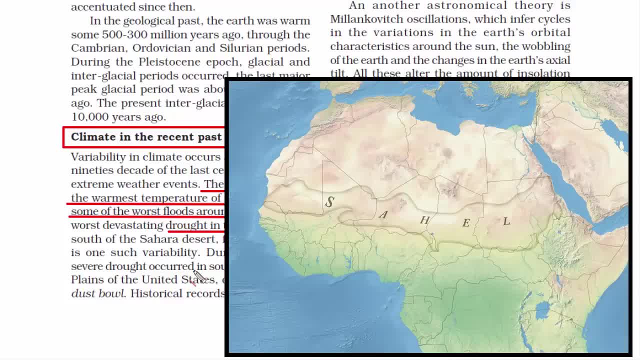 occurred during 1960s and 70s. occurred during 1960s and 70s. was in sahel region. i'll show you where was in sahel region. i'll show you where was in sahel region. i'll show you where sahel is. 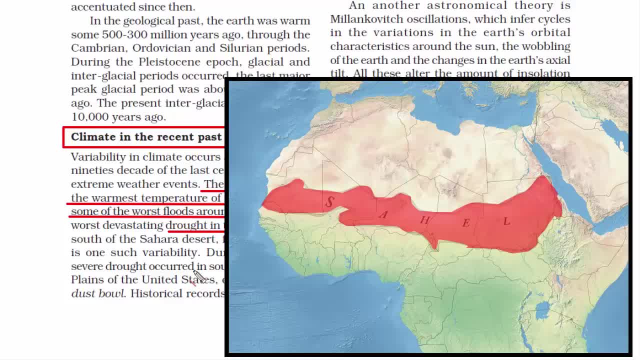 sahel is sahel. is this region over here? sahara desert? is this region over here, sahara desert? is this region over here? sahara desert is here. the northern part of africa, here the northern part of africa, here the northern part of africa, countries like algeria, djibouti, egypt. countries like algeria, djibouti, egypt. countries like algeria, djibouti, egypt, libya, morocco, somalia, sudan and tunisia. libya, morocco, somalia, sudan and tunisia. libya, morocco, somalia, sudan and tunisia are part of sahara desert. 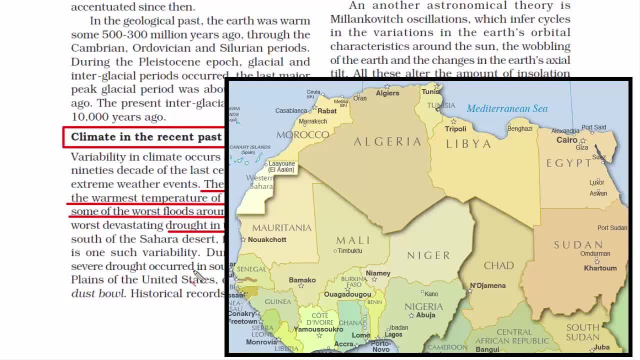 are part of sahara desert are part of sahara desert, and below that we have mauritania mali, and below that we have mauritania mali, and below that we have mauritania mali, niger, shad and sudan, which are 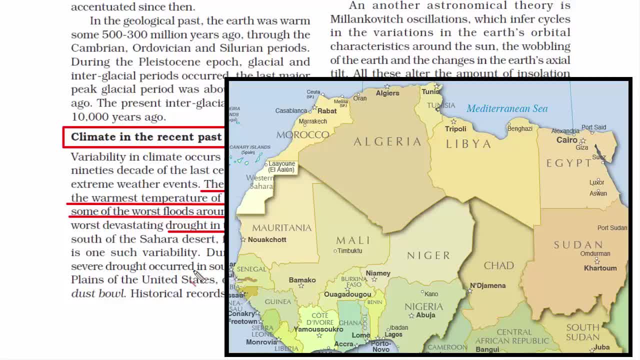 niger shad and sudan, which are niger shad and sudan, which are sub-saharan countries, sub-saharan countries, sub-saharan countries. meaning they are not 100 percent part, meaning they are not 100 percent part. meaning they are not 100 percent part of sahara desert. 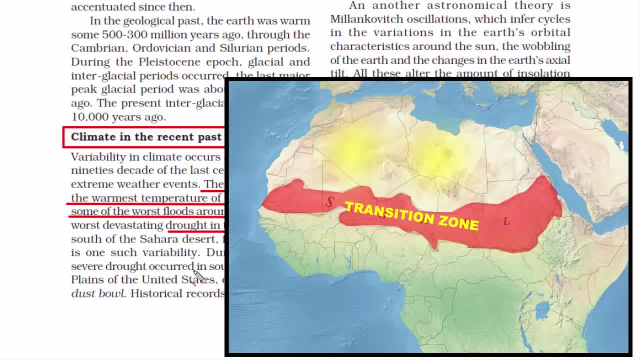 of sahara desert, of sahara desert. so that makes this region sahel as a. so that makes this region sahel as a. so that makes this region sahel as a transition zone between an arid and transition zone between an arid and. 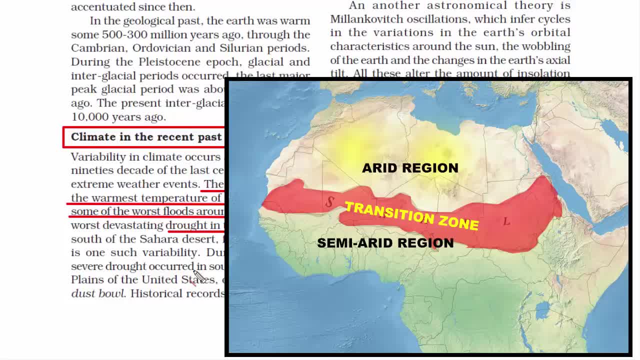 transition zone between an arid and semi-arid region. semi-arid region- semi-arid region- so arid- means completely dry region. which so arid means completely dry region which so arid means completely dry region which is a desert, and semi-arid means there is. 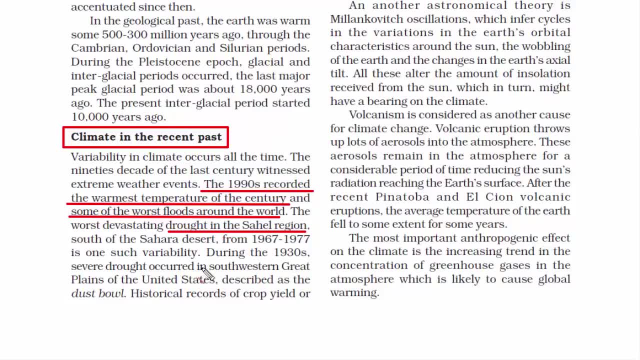 is a desert, and semi-arid means there is is a desert and semi-arid means there is a little bit of vegetation. due to a little bit of vegetation, due to a little bit of vegetation, due to very low rainfall. then during the 1930s, 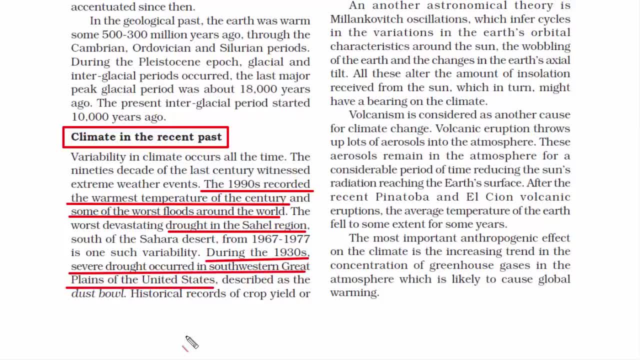 very low rainfall then during the 1930s, very low rainfall then during the 1930s. there was a severe drought in. there was a severe drought in. there was a severe drought in southwestern great plains of united southwestern great plains of united southwestern great plains of united states. 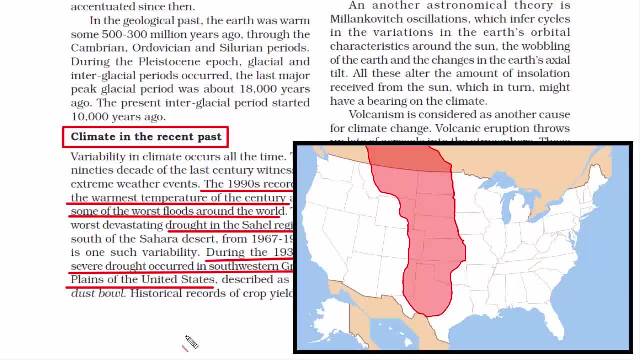 states states. so when we say great plains of united, so when we say great plains of united, so when we say great plains of united states states states, it is this region. if you look at this map, it is this region. if you look at this map, it is this region. if you look at this map of usa. 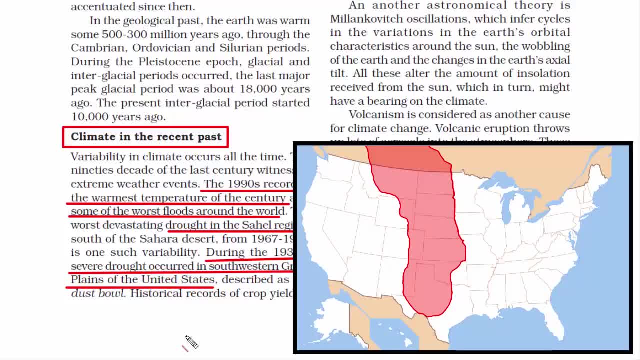 of usa, of usa. this red portion is the region of great. this red portion is the region of great. this red portion is the region of great plains that witnessed severe drought, plains that witnessed severe drought plains that witnessed severe drought during 1930s, during 1930s. 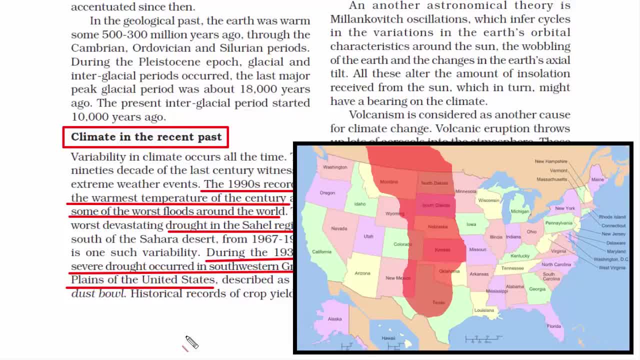 during 1930s. so these are the states that are part of. so these are the states that are part of. so these are the states that are part of this region. just have a look at it. this region, just have a look at it, this region, just have a look at it. so, obviously, if there was a drought, then 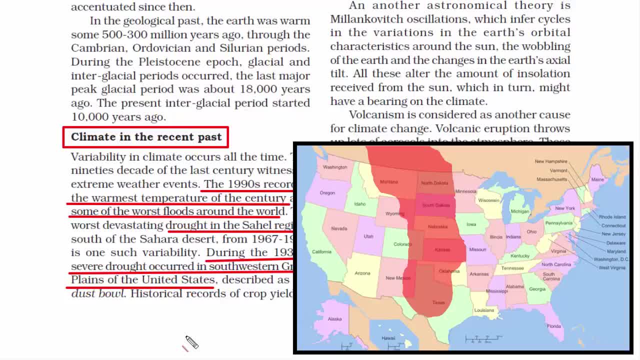 so obviously, if there was a drought then. so obviously, if there was a drought, then it must have affected the agricultural. it must have affected the agricultural, it must have affected the agricultural business, business, business. because when we say great plains that, because when we say great plains that, 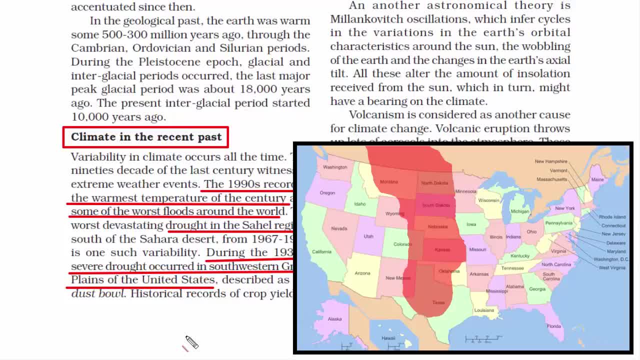 because when we say great plains, that means this region has to be highly means. this region has to be highly means this region has to be highly suitable for agriculture, suitable for agriculture, suitable for agriculture, and because of the 1930s drought there and because of the 1930s drought there, 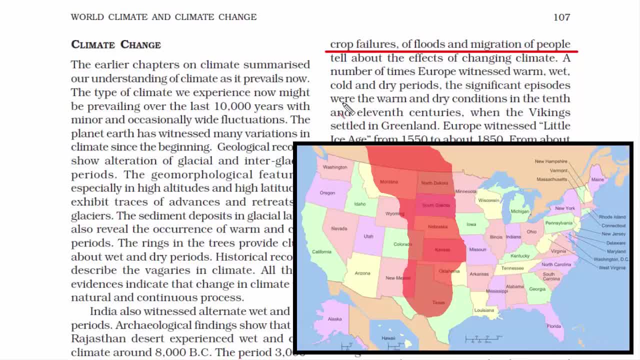 and because of the 1930s drought, there was a massive crop failure, was a massive crop failure, was a massive crop failure. then agriculture business went down. then agriculture business went down. then agriculture business went down. people migrated. so i think it is a good. people migrated, so i think it is a good. 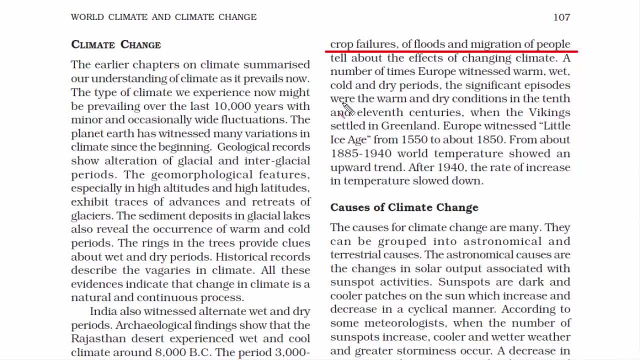 people migrated. so i think it is a good example, example, example of how the changing climate affects, of how the changing climate affects, of how the changing climate affects humans, both socially and economically, humans both socially and economically, humans both socially and economically. even europe witnessed warm, wet, cold and 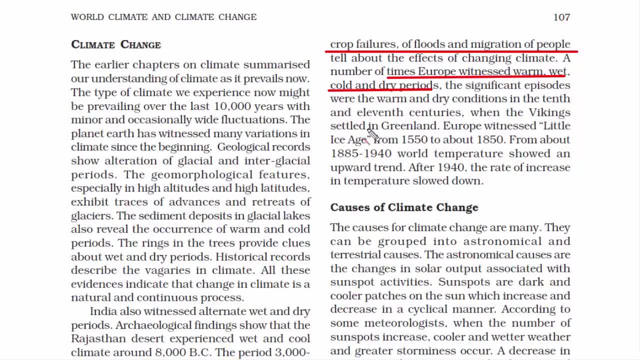 even europe witnessed warm, wet, cold, and even europe witnessed warm, wet, cold and dry periods in the 10th and 11th dry periods in the 10th and 11th dry periods in the 10th and 11th centuries, centuries, centuries. so ice age is an era when huge parts of 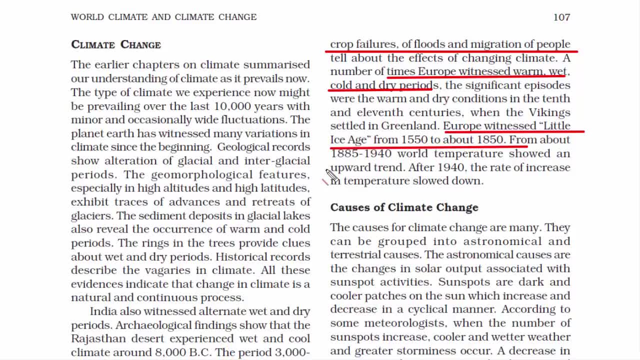 so ice age is an era when huge parts of. so ice age is an era when huge parts of the planet earth was covered with. the planet earth was covered with. the planet earth was covered with glaciers, glaciers, glaciers, and i don't have to tell you where the 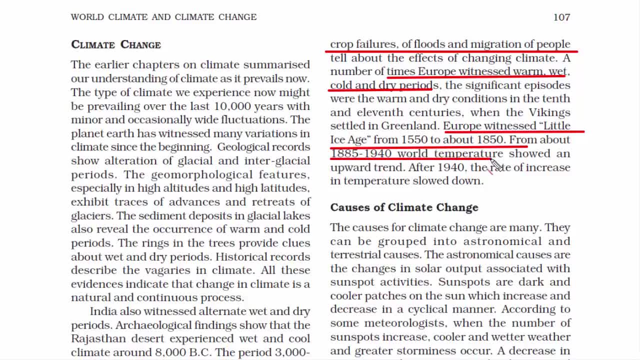 and i don't have to tell you where the and i don't have to tell you where the ice age was super active. ice age was super active. ice age was super active. you know, you can easily figure out that. you know, you can easily figure out that. 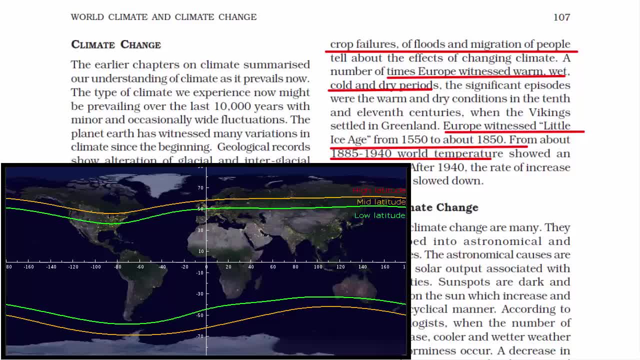 you know, you can easily figure out that is in the higher latitude areas. ice age is in the higher latitude areas, ice age is in the higher latitude areas. ice age was extreme, was extreme, was extreme because we have read numerous times that. because we have read numerous times that 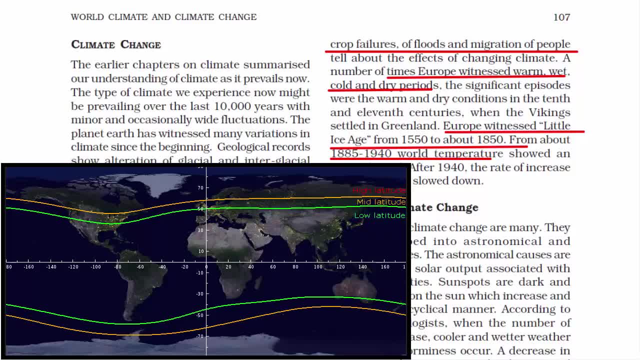 because we have read numerous times that as we go away from the equator, as we go away from the equator, as we go away from the equator, temperature drops, so ice age naturally, temperature drops, so ice age, naturally, temperature drops. so ice age naturally had to be in the higher latitude areas. had to be in the higher latitude areas, had to be in the higher latitude areas. that's why when you go to antarctica, or that's why when you go to antarctica, or that's why when you go to antarctica or arctic region, 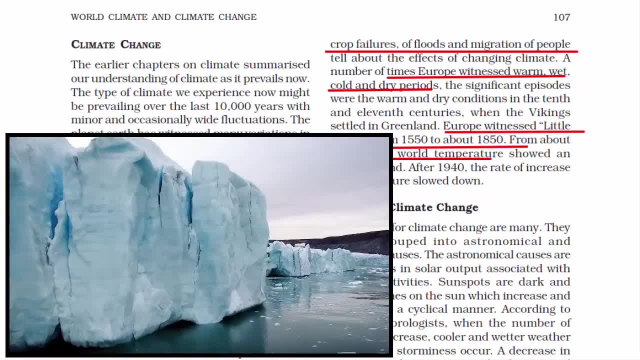 arctic region, arctic region. these are the only places where you will. these are the only places where you will. these are the only places where you will find massive amount of glaciers, find massive amount of glaciers, find massive amount of glaciers all throughout the year. however, there 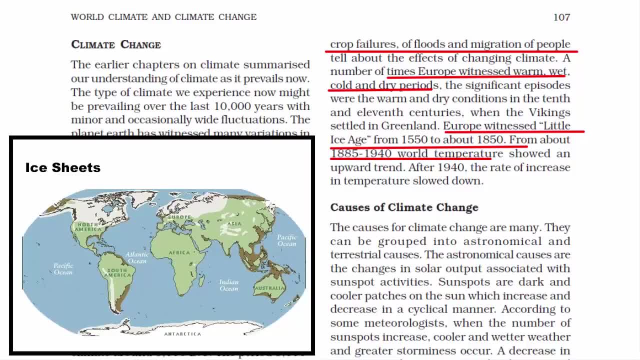 all throughout the year, however, there all throughout the year, however, there was one point in time when massive was one point in time when massive was one point in time when massive sheets of ice from the arctic region and sheets of ice from the arctic region and 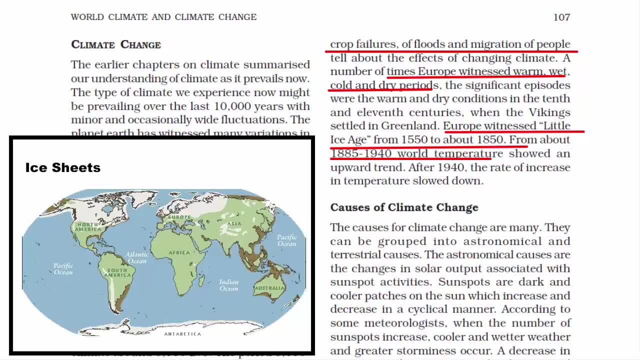 sheets of ice from the arctic region and antarctica covered large parts of europe. antarctica covered large parts of europe. antarctica covered large parts of europe, north america and south america, and also north america and south america, and also north america and south america and also some areas in asia. 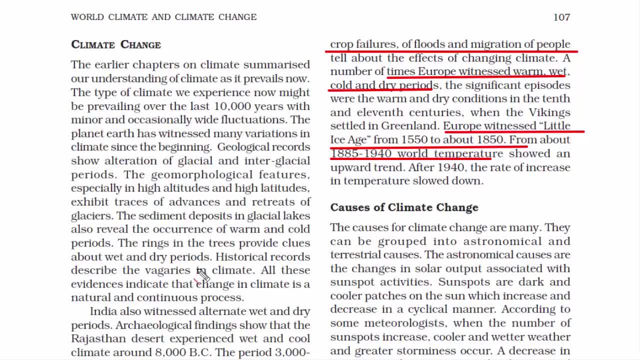 some areas in asia, some areas in asia, and that's why today also these places, and that's why today also these places, and that's why today also these places at times get super cold, at times get super cold, at times get super cold. so anyways, the whole point is that today 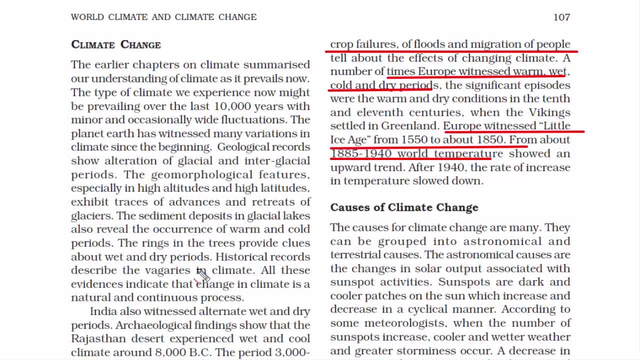 so, anyways, the whole point is that today. so, anyways, the whole point is that today we are no longer in ice age. today we are. we are no longer in ice age. today we are. we are no longer in ice age. today we are in interglacial period, or halocene. 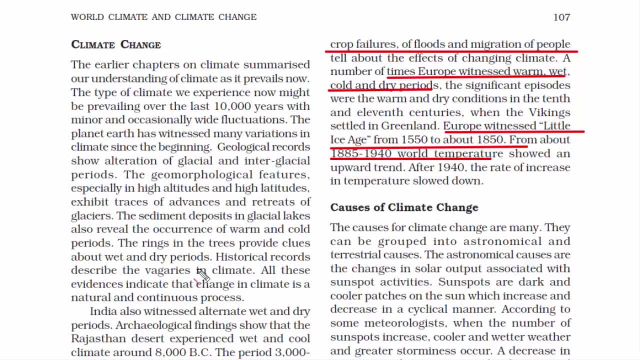 in interglacial period or halocene. in interglacial period or halocene period, period, period. ice age lasted till 11 700 years ago. ice age lasted till 11 700 years ago. ice age lasted till 11 700 years ago. since then, the temperature has slowly. 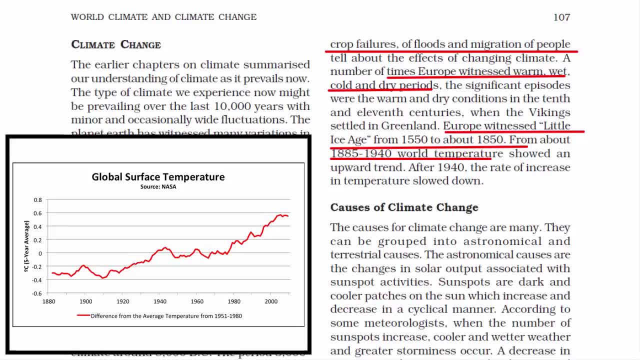 since then, the temperature has slowly. since then, the temperature has slowly gone up and after industrial revolution gone up, and after industrial revolution gone up, and after industrial revolution, it's increasing, it's increasing, it's increasing. i'll talk about all the geological time. i'll talk about all the geological time. 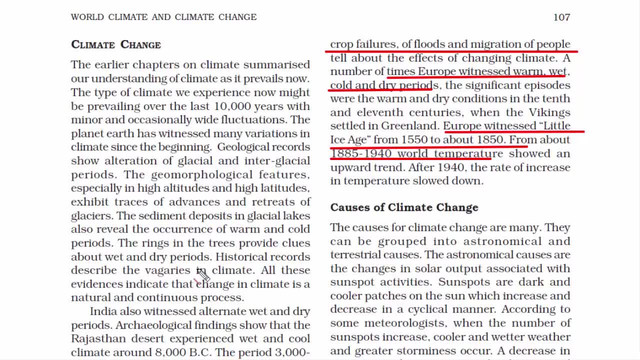 i'll talk about all the geological time scale in a separate video. so there i'll scale in a separate video. so there i'll scale in a separate video. so there i'll explain in detail how the planet earth, explain in detail how the planet earth explain in detail how the planet earth went through different phases. 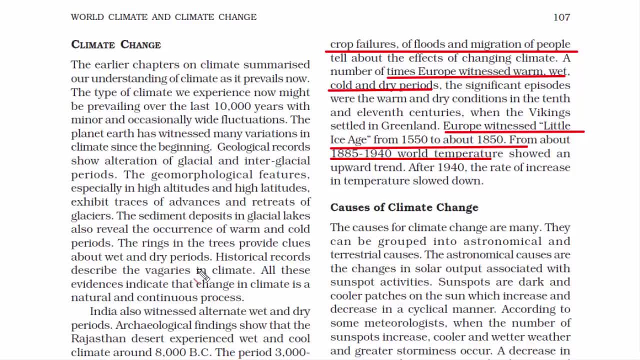 went through different phases, went through different phases. what kind of temperature existed in? what kind of temperature existed in, what kind of temperature existed in those phases and, more importantly, those phases and, more importantly, those phases and, more importantly, how did we all evolved into what we are? how did we all evolved into what we are? 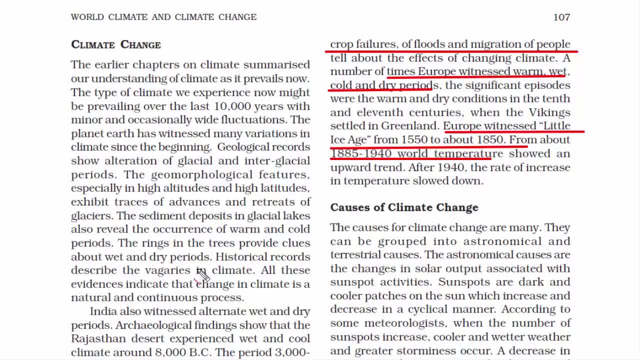 how did we all evolved into what we are today, today, today, so yeah, i'll cover all that in a. so yeah, i'll cover all that in a. so yeah, i'll cover all that in a separate video. anyways, that is all there. separate video, anyways, that is all there. 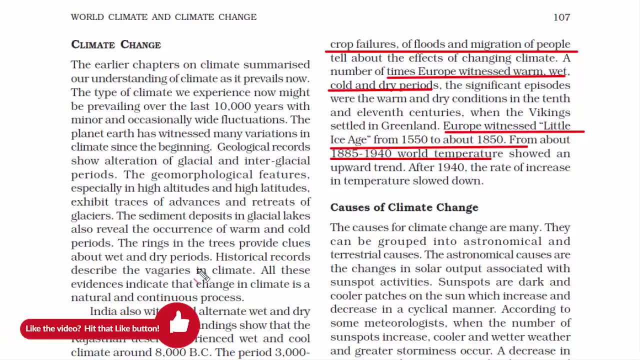 separate video. anyways, that is all there is to read in this topic. pause the video is to read in this topic. pause the video is to read in this topic. pause the video and read it once again and vaguely. and read it once again and vaguely. and read it once again and vaguely. remember the dates. 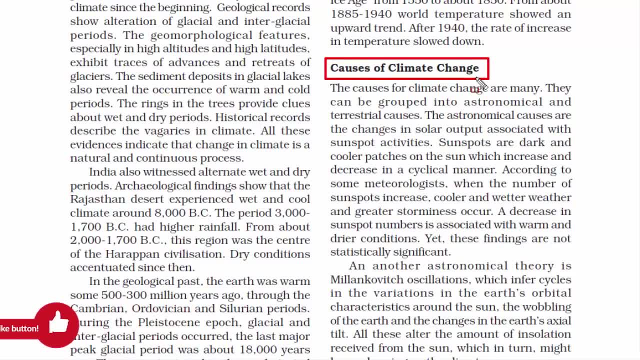 remember the dates. remember the dates. now, let's get to know about the causes now. let's get to know about the causes. now, let's get to know about the causes of climate change, of climate change, of climate change. i'll quickly summarize this entire topic. i'll quickly summarize this entire topic. 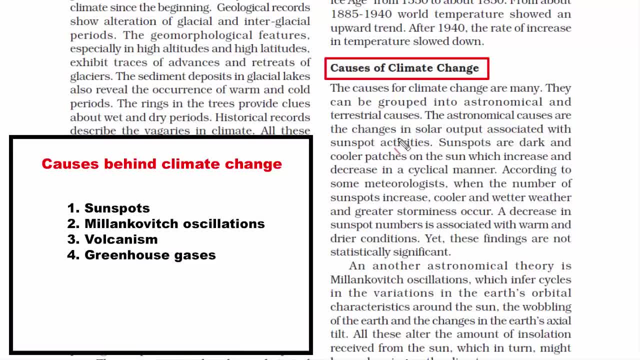 i'll quickly summarize this entire topic. basically there are four factors for. basically there are four factors for. basically there are four factors for climate change: climate change, climate change. so here it's clearly written that it is so. here it's clearly written that it is so. here it's clearly written that it is grouped into astronomical and 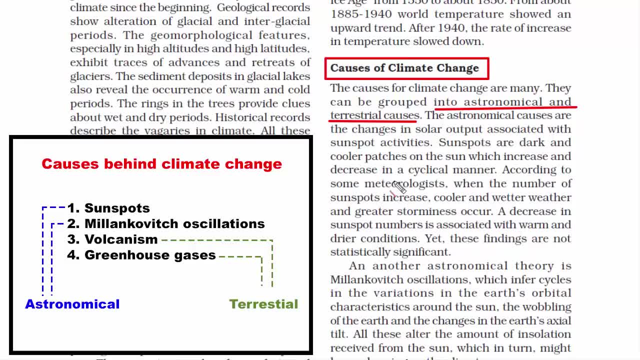 grouped into astronomical, and grouped into astronomical and terrestrial causes. terrestrial causes, terrestrial causes now. astronomical means relating to now. astronomical means relating to now. astronomical means relating to astronomy: you know planetary heavenly astronomy. you know planetary heavenly astronomy. you know planetary heavenly factors, which is far beyond anybody's. 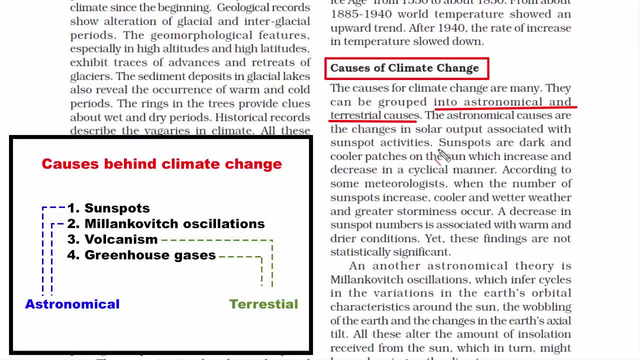 factors, which is far beyond anybody's factors, which is far beyond anybody's control, and it is outside the earth control, and it is outside the earth control. and it is outside the earth i mean earth is smaller in front of, i mean earth is smaller in front of. 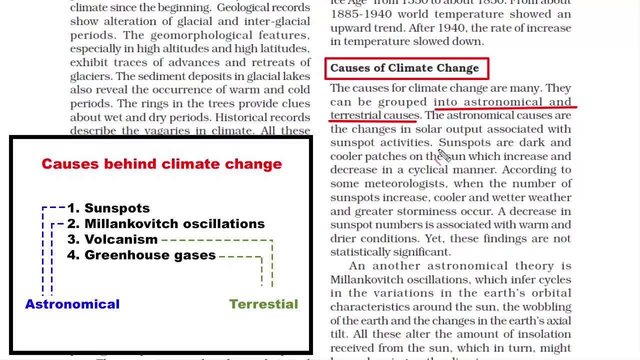 i mean earth is smaller in front of astronomical factors, astronomical factors, astronomical factors, and terrestrial means something which, and terrestrial means something which and terrestrial means something which is related to the earth, is related to the earth, is related to the earth things that happen within the atmosphere, things that happen within the atmosphere. 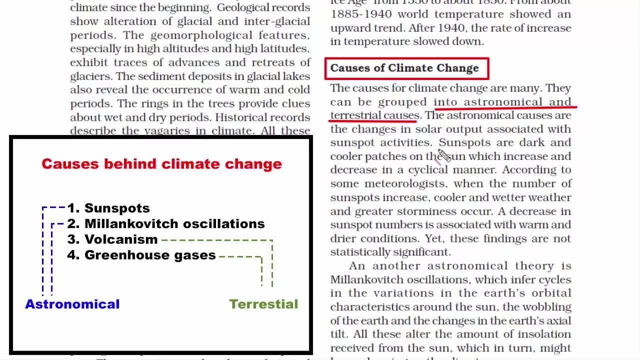 things that happen within the atmosphere of the earth, of the earth, of the earth. so basically the factors for climate. so basically the factors for climate. so basically the factors for climate change has been broadly categorized. change has been broadly categorized. change has been broadly categorized under astronomical, under astronomical. 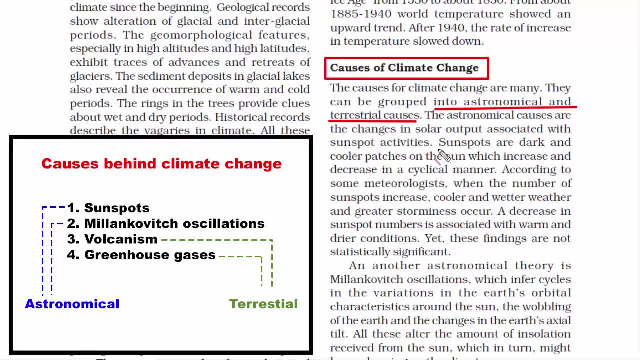 under astronomical and terrestrial causes- all right, let's. and terrestrial causes: all right, let's. and terrestrial causes, all right, let's now understand those four factors. now understand those four factors. now understand those four factors. the first one is sunspots, now sunspots. the first one is sunspots, now sunspots. 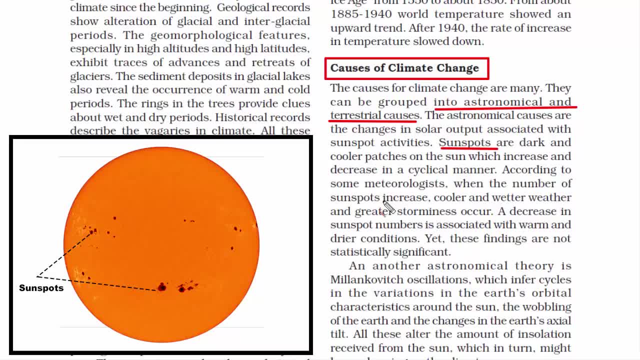 the first one is sunspots. now, sunspots. are these dark spots that appear on the? are these dark spots that appear on the? are these dark spots that appear on the surface of the sun surface of the sun surface of the sun? i know, right, it's kind of crazy to even i know, right, it's kind of crazy to even- i know right, it's kind of crazy to even think of it that way. because think of it that way, because think of it that way? because we have never looked into the sun. we have never looked into the sun. 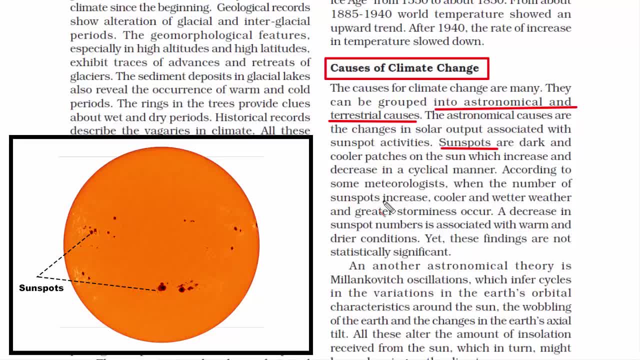 we have never looked into the sun directly and we all have seen spots on directly. and we all have seen spots on directly and we all have seen spots on moon. i'm sure it's highly unlikely that moon. i'm sure it's highly unlikely that moon. i'm sure it's highly unlikely that you have ever noticed spots on the. 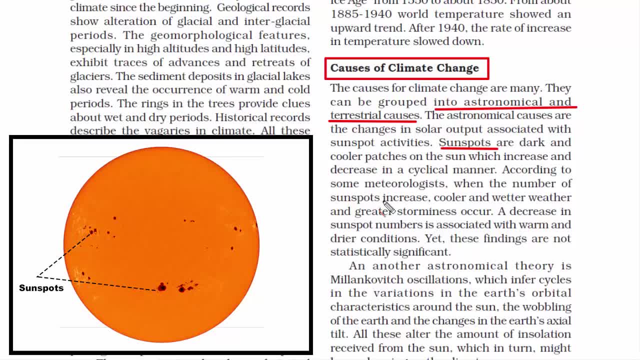 you have ever noticed spots on the? you have ever noticed spots on the surface of the sun, surface of the sun, surface of the sun? so, anyways, there are some spots that. so, anyways, there are some spots that. so, anyways, there are some spots that exist on the sun. 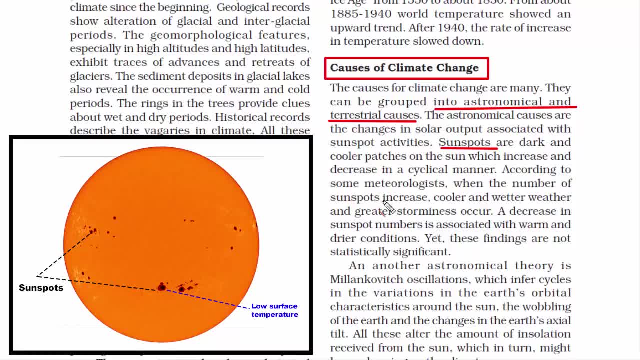 exist on the sun, exist on the sun and these spots have low surface and these spots have low surface and these spots have low surface temperature, temperature, temperature. it's a temporary cool and dark region. it's a temporary cool and dark region. it's a temporary cool and dark region. some of these sun spots are many times. 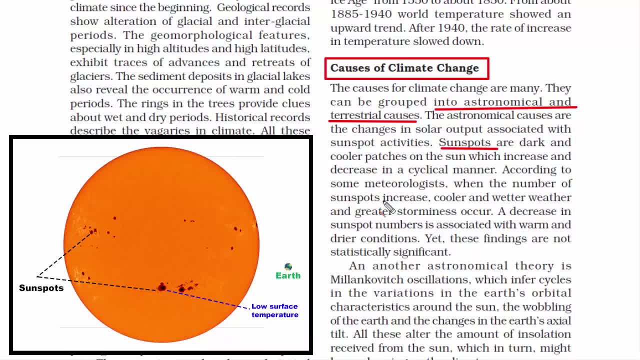 some of these sun spots are many times, some of these sun spots are many times bigger than the earth, bigger than the earth, bigger than the earth. and when i say these sun spots are dark, and when i say these sun spots are dark, and when i say these sun spots are dark and cool, what i mean is that the 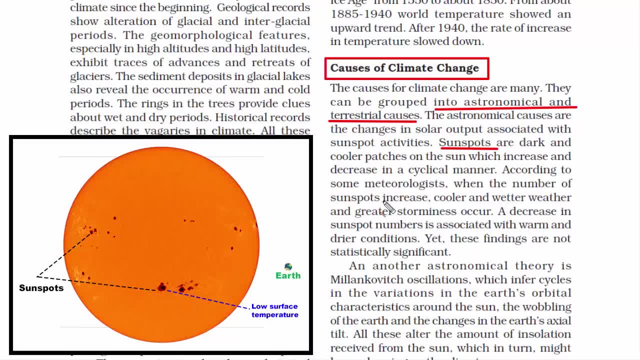 and cool. what i mean is that the and cool. what i mean is that the temperature of these dark spots, temperature of these dark spots, temperature of these dark spots is lesser than the rest of the surface, is lesser than the rest of the surface, is lesser than the rest of the surface of the sun. 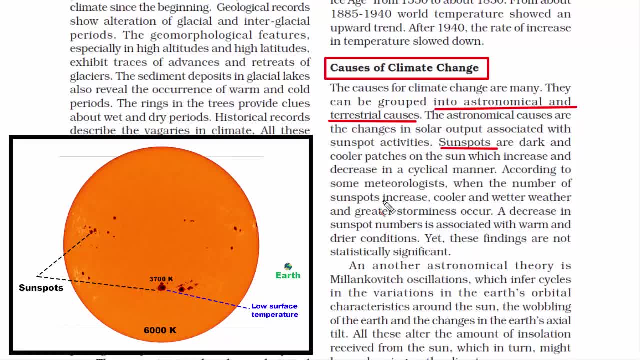 of the sun, of the sun, for example, if the temperature of the sun, for example, if the temperature of the sun, for example, if the temperature of the sun is 6000 kelvin, is 6000 kelvin, is 6000 kelvin, then the temperature of these sun spots. 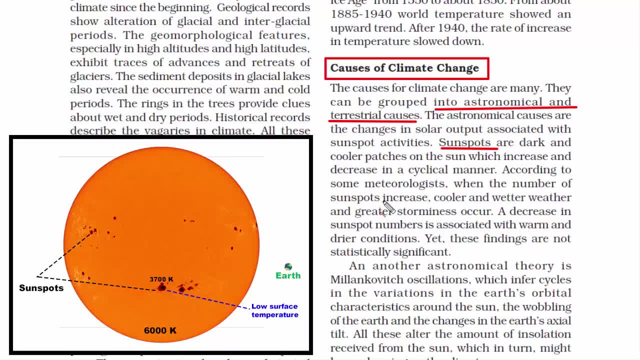 then the temperature of these sun spots, then the temperature of these sun spots are 3700 kelvin, are 3700 kelvin, are 3700 kelvin. so you see it's a bit cooler than the rest. so you see it's a bit cooler than the rest. 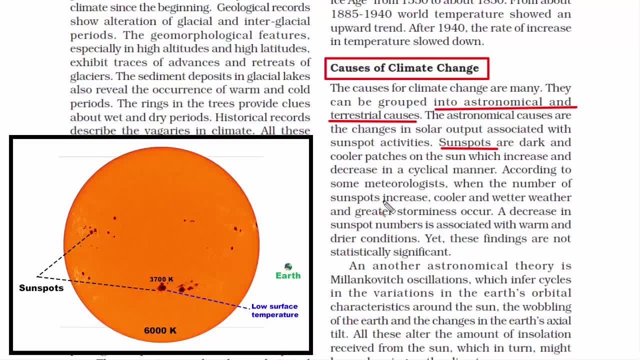 so you see, it's a bit cooler than the rest of the solar surface, of the solar surface, of the solar surface. anyways, the theory goes like this. when, anyways, the theory goes like this. when, anyways, the theory goes like this: when the number of sun spots increases, the number of sun spots increases. 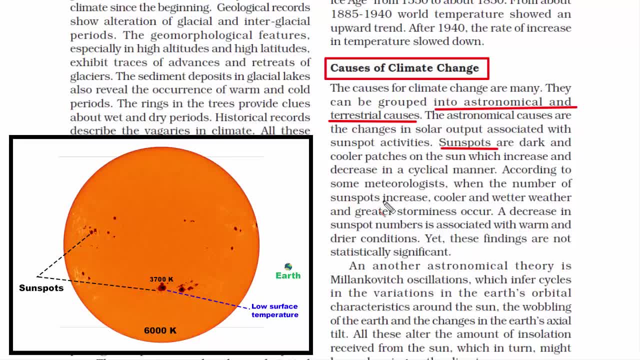 the number of sun spots increases, cooler and wetter weather and greater cooler and wetter weather and greater cooler and wetter weather and greater storminess occur. storminess occur. storminess occur because, moments back i told you some of, because moments back i told you some of 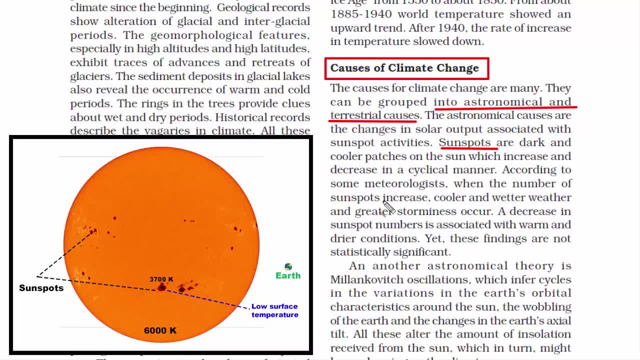 because, moments back, i told you, some of these sun spots are much bigger than the. these sun spots are much bigger than the. these sun spots are much bigger than the size of the earth. size of the earth. size of the earth. just think about it. if the position of 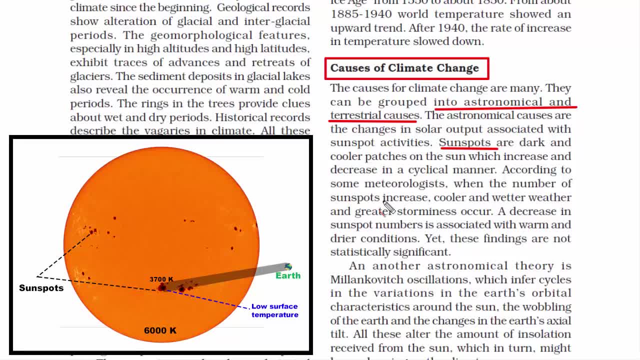 just think about it. if the position of just think about it, if the position of one of the sun spots is such that one of the sun spots is such that one of the sun spots is such that it is in direct conjunction with the, it is in direct conjunction with the. 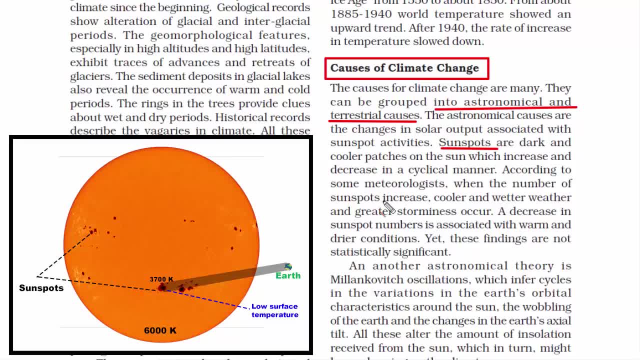 it is in direct conjunction with the earth, then obviously the amount of earth, then obviously the amount of earth, then obviously the amount of incoming solar radiation on earth, will incoming solar radiation on earth, will incoming solar radiation on earth will be affected, be affected, be affected and that can cause cool and wet weather. 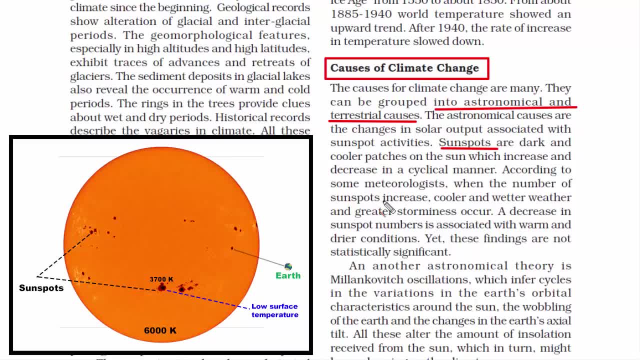 and that can cause cool and wet weather. and that can cause cool and wet weather. similarly, a decrease in sunspot numbers. similarly, a decrease in sunspot numbers. similarly, a decrease in sunspot numbers is associated with warm and drier. is associated with warm and drier. 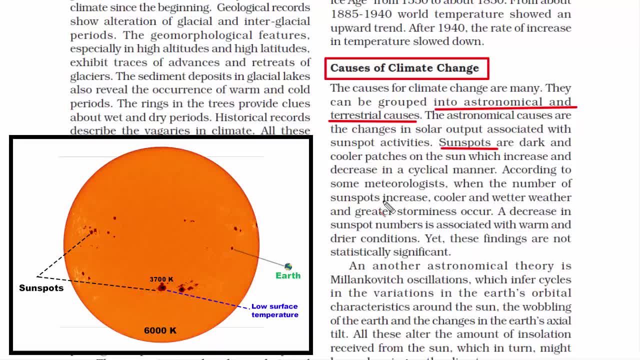 is associated with warm and drier conditions. conditions, conditions that means incoming solar radiation on. that means incoming solar radiation on. that means incoming solar radiation on earth will be in excess. earth will be in excess, earth will be in excess. so this kind of theory falls under. so this kind of theory falls under. 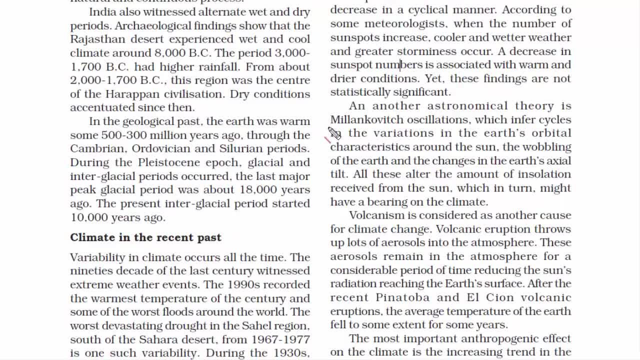 so this kind of theory falls under astronomical causes, astronomical causes, astronomical causes. the second factor for climate change is: the second factor for climate change is: the second factor for climate change is milankovitch oscillation. milankovitch oscillation, milankovitch oscillation. even this one falls under astronomical 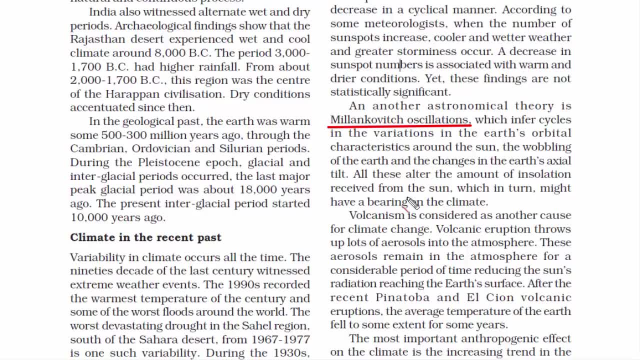 even this one falls under astronomical. even this one falls under astronomical theory theory theory because this factor is beyond anyone's. because this factor is beyond anyone's, because this factor is beyond anyone's control on earth, control on earth, control on earth. no one can do anything about it anyways. 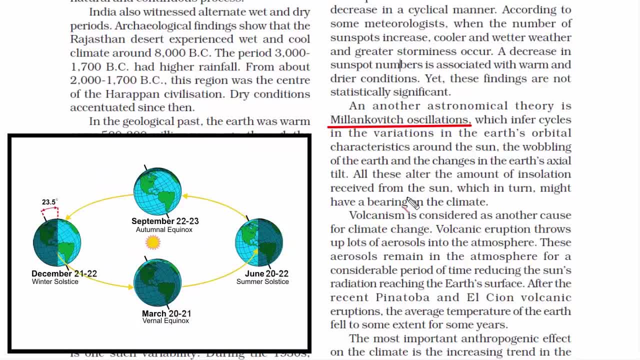 no one can do anything about it anyways. no one can do anything about it anyways. this theory talks about the variation. this theory talks about the variation. this theory talks about the variation in earth's orbital motion around the sun, in earth's orbital motion around the sun, in earth's orbital motion around the sun. i think this shouldn't be hard to think. 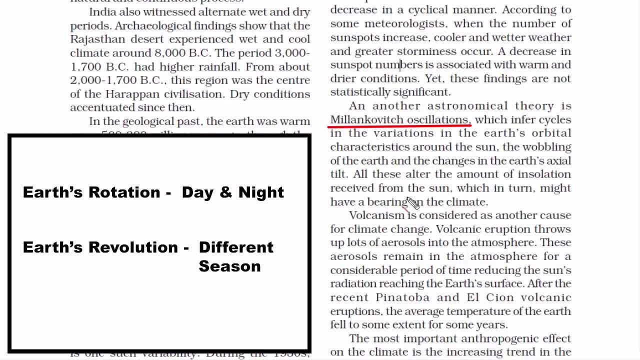 i think this shouldn't be hard to think. i think this shouldn't be hard to think about, about, about, because we know two facts about the. because we know two facts about the. because we know two facts about the earth. one is that earth rotates within earth. one is that earth rotates within. 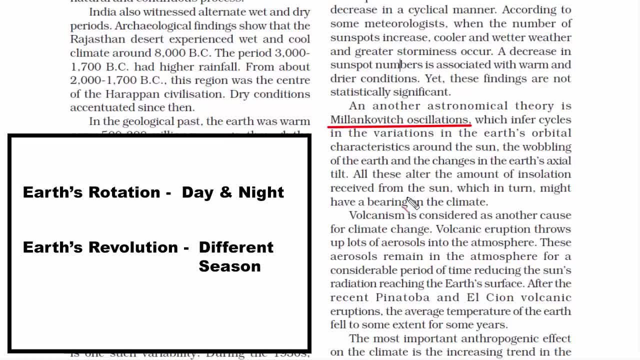 earth. one is that earth rotates within its own axis, its own axis, its own axis which determines our day and night, and which determines our day and night, and which determines our day and night. and the second one is that earth revolves. the second one is that earth revolves. 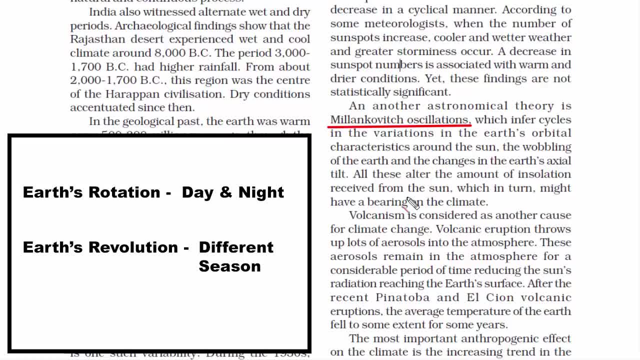 the second one is that earth revolves around the sun, which makes the earth around the sun, which makes the earth around the sun, which makes the earth experience different seasons, experience different seasons, experience different seasons. now we are interested in earth's. now we are interested in earth's. 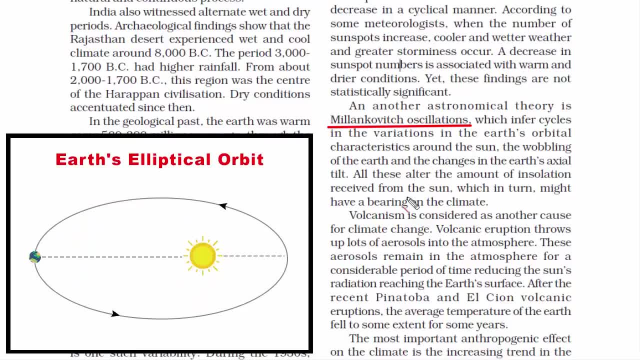 now we are interested in earth's revolution, when earth revolves around revolution, when earth revolves around revolution, when earth revolves around the sun. earth's orbit is not in a perfect the sun. earth's orbit is not in a perfect the sun. earth's orbit is not in a perfect circle. 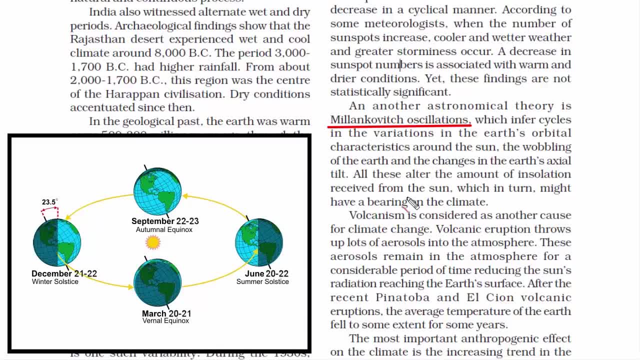 circle, circle. actually, this is the picture that we actually this is the picture that we actually this is the picture that we have always seen here we see the earth's have always seen here. we see the earth's have always seen here. we see the earth's orbital motion being a perfect circle. 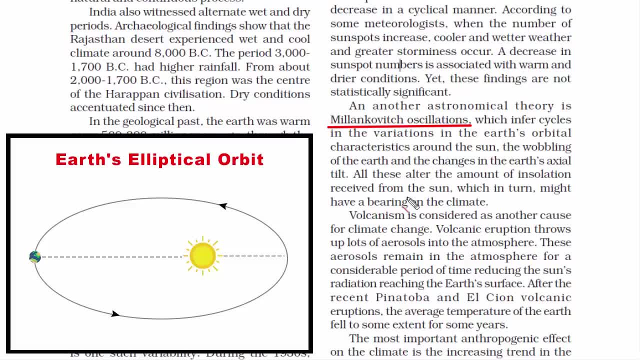 orbital motion being a perfect circle. orbital motion being a perfect circle, but that's not true. it is more of an, but that's not true. it is more of an, but that's not true. it is more of an elliptical shape where the sun is nearer. elliptical shape where the sun is nearer. 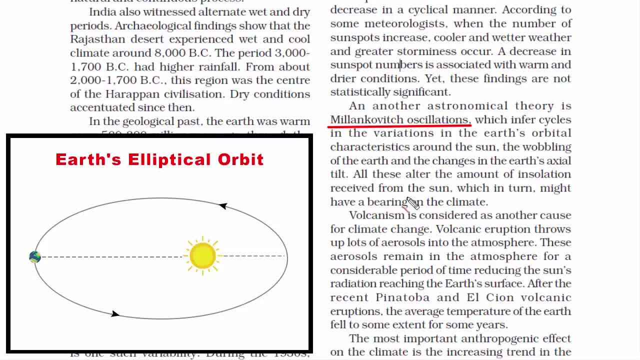 elliptical shape where the sun is nearer to one end of the ellipse, to one end of the ellipse, to one end of the ellipse. so this is the actual illustration of, so this is the actual illustration of, so this is the actual illustration of how the earth revolves around the sun. 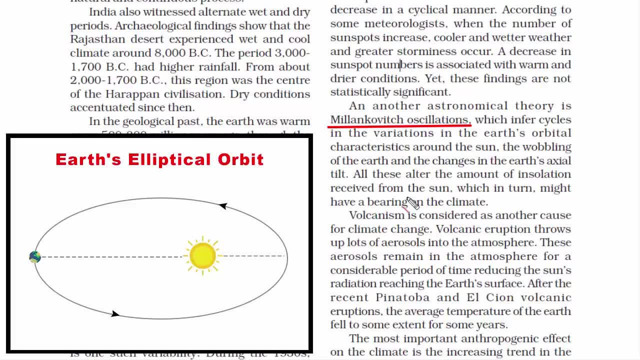 how the earth revolves around the sun, how the earth revolves around the sun, and one more thing that i want to, and one more thing that i want to, and one more thing that i want to specifically mention, is that specifically mention. is that specifically mention is that when the earth travels, one entire trip. 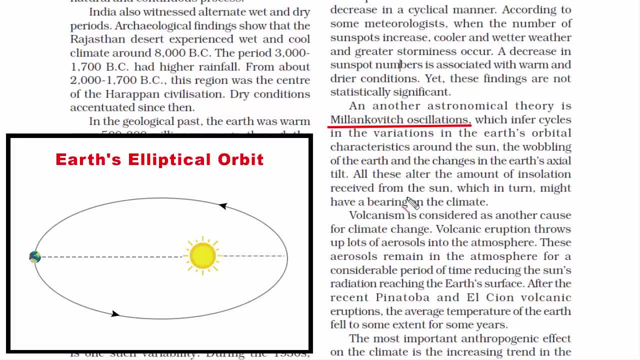 when the earth travels one entire trip, when the earth travels one entire trip around the sun, it does not return to the around the sun. it does not return to the around the sun. it does not return to the same starting point. same starting point, same starting point: there is deviation in the elliptical path. 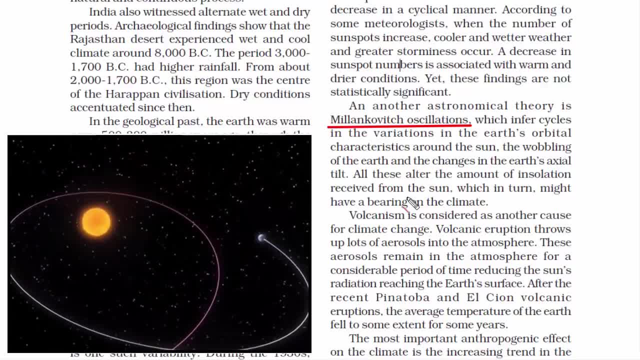 there is deviation in the elliptical path. there is deviation in the elliptical path after the earth has completed one, after the earth has completed one, after the earth has completed one revolution around the sun, revolution around the sun, revolution around the sun. and the reason behind this deviation is 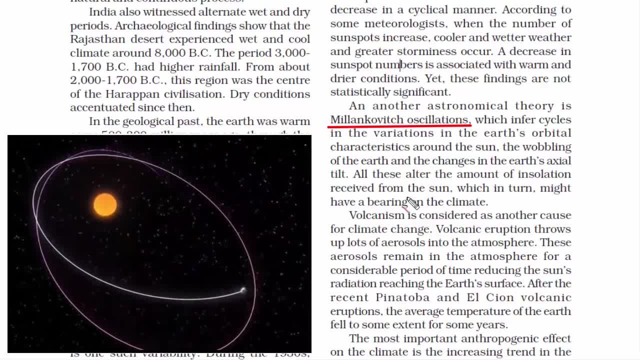 and the reason behind this deviation is, and the reason behind this deviation is the result of gravitational attraction, the result of gravitational attraction, the result of gravitational attraction among other planets, among other planets, among other planets. you see, after all, every planet is. you see, after all, every planet is. 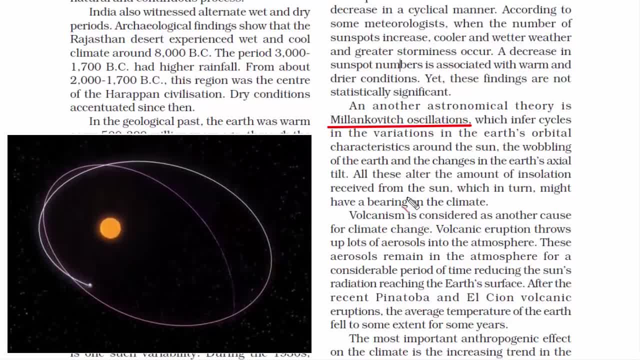 you see, after all, every planet is revolving around the sun, and then there revolving around the sun, and then there revolving around the sun, and then there are planets like jupiter and saturn are planets like jupiter and saturn are planets like jupiter and saturn. they are much bigger than earth. hence, 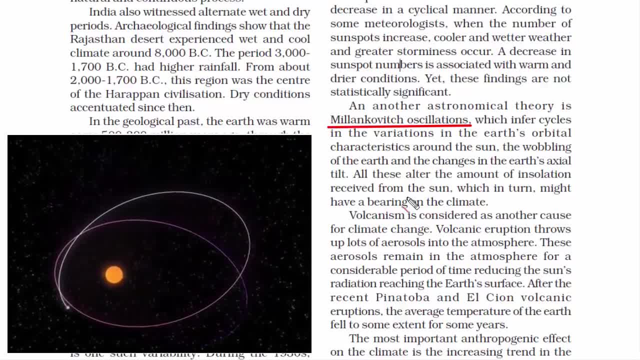 they are much bigger than earth. hence, they are much bigger than earth. hence the moving pattern around the sun, in the moving pattern around the sun, in the moving pattern around the sun. in other words, the elliptical path has other words, the elliptical path has other words. the elliptical path has some effect on earth's elliptical path. 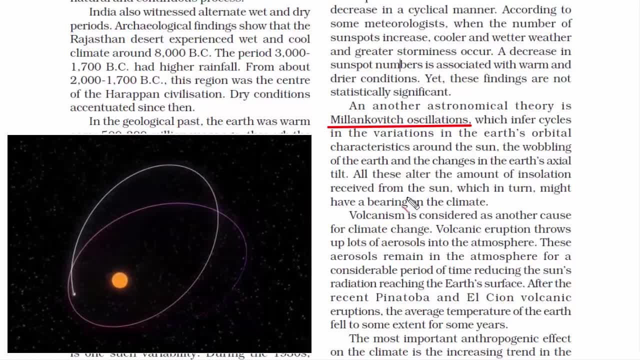 some effect on earth's elliptical path, some effect on earth's elliptical path. that's why the earth after completing, that's why the earth after completing, that's why the earth, after completing its one revolution, never returns to the. its one revolution never returns to the. 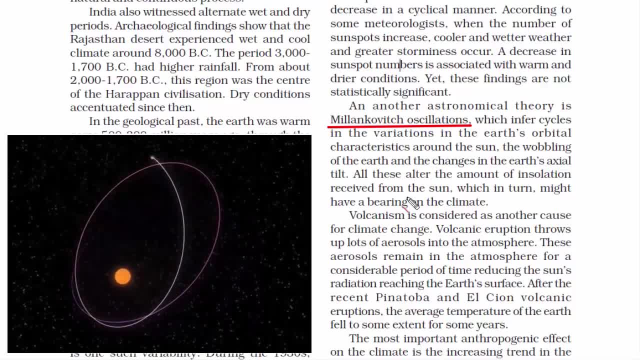 its one revolution never returns to the same starting point, and that is also the same starting point. and that is also the same starting point, and that is also the reason behind coordinating our calendar, reason behind coordinating our calendar, reason behind coordinating our calendar with the earth's motion which gives us 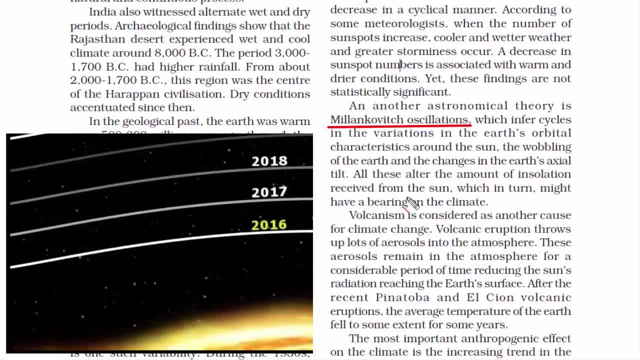 with the earth's motion which gives us, with the earth's motion which gives us, leap year. if i have to sum up this leap year, if i have to sum up this leap year, if i have to sum up this concept in the most simplest manner, then, concept in the most simplest manner, then 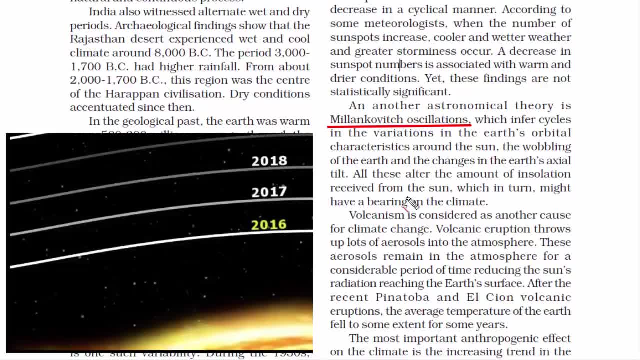 concept in the most simplest manner, then just remember. this earth is not exactly just remember. this earth is not exactly just remember. this earth is not exactly at the same spot in its orbit on your, at the same spot in its orbit on your. at the same spot in its orbit on your birthday, every year. 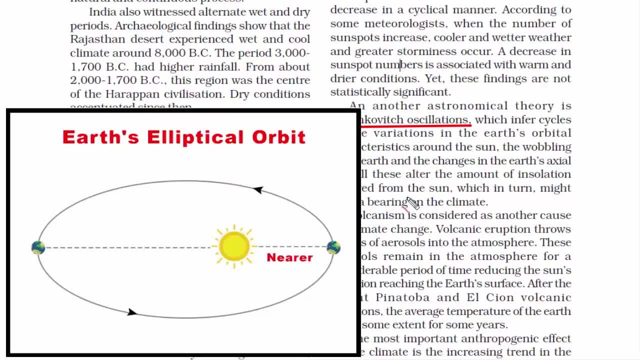 birthday every year. birthday every year. all right now you need to know. is that all right now you need to know? is that all right now you need to know? is that the speed of the earth in this elliptical, the speed of the earth in this elliptical? 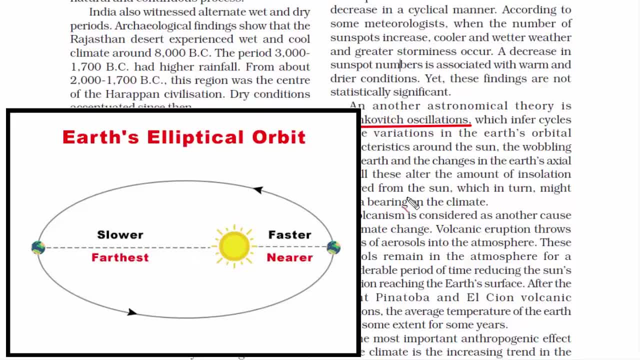 the speed of the earth in this elliptical orbit is maximum when it is closest to orbit, is maximum when it is closest to orbit, is maximum when it is closest to the sun and when it is far. the speed is the sun and when it is far, the speed is. 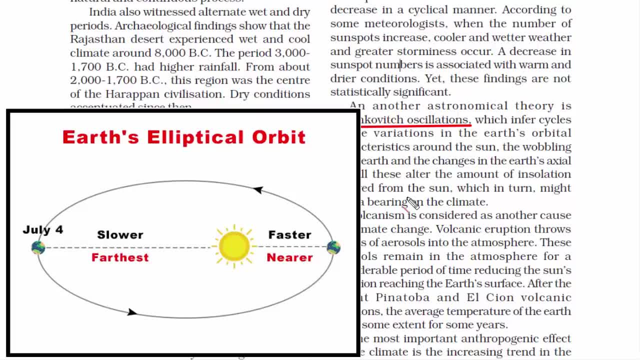 the sun and when it is far, the speed is minimum. so during the month of july, that minimum. so during the month of july, that minimum. so during the month of july, that is fourth july- the earth is farthest- is fourth july, the earth is farthest. 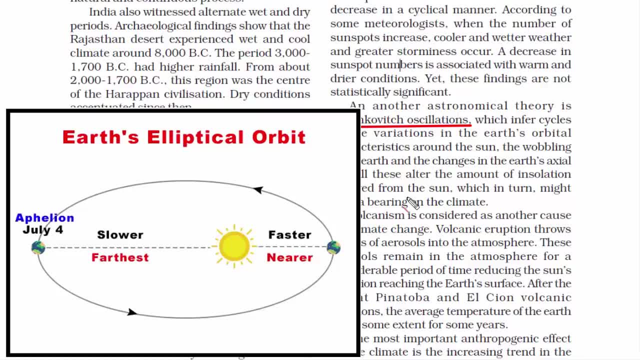 is fourth july. the earth is farthest from the sun. this position of earth is from the sun. this position of earth is from the sun. this position of earth is called aphelion, wherein we are 152.6. called aphelion, wherein we are 152.6. 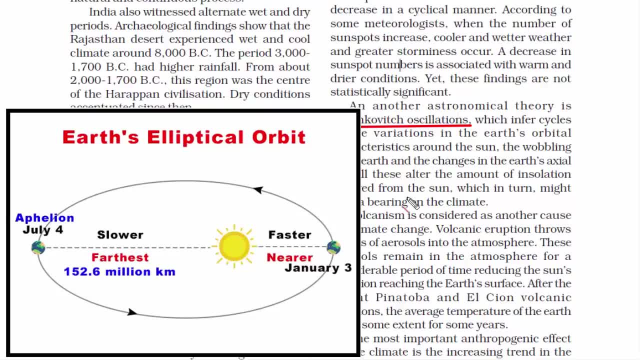 called aphelion, wherein we are 152.6 million kilometers away from the sun and million kilometers away from the sun and million kilometers away from the sun, and, on the other hand, on 3rd january the. on the other hand, on 3rd january the. 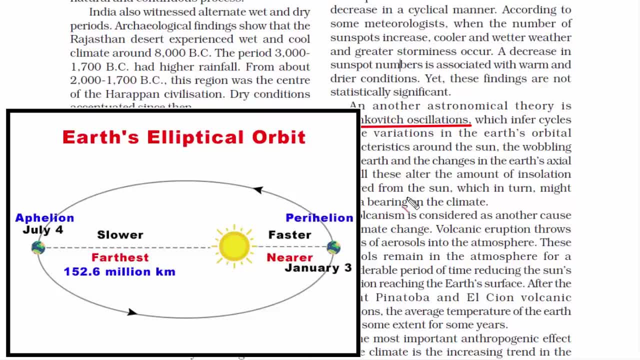 on the other hand, on 3rd january, the earth is nearest to the sun and this earth is nearest to the sun and this earth is nearest to the sun. and this position is called perihelion- here we. position is called perihelion- here we. 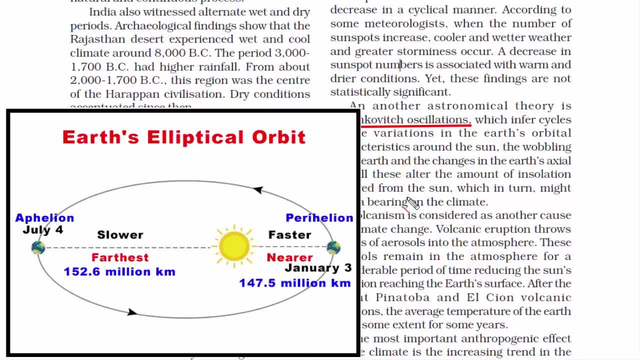 position is called perihelion. here we are 147.5 million kilometers away from. are 147.5 million kilometers away from, are 147.5 million kilometers away from the sun, the sun, the sun. hence we can say that the annual. hence we can say that the annual. 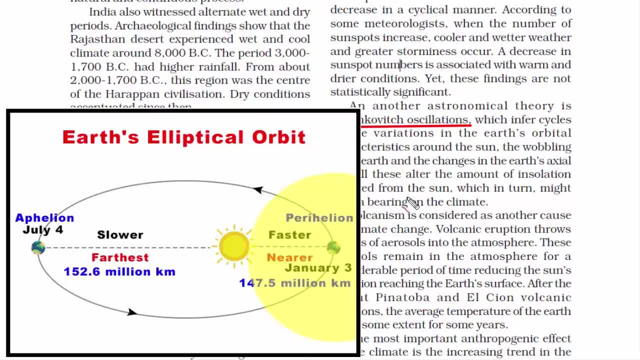 hence we can say that the annual insulation, that is the incoming solar insulation, that is the incoming solar insulation, that is the incoming solar energy or sun rays is more on 3rd energy or sun rays is more on 3rd energy or sun rays is more on 3rd january and incoming solar energy is. 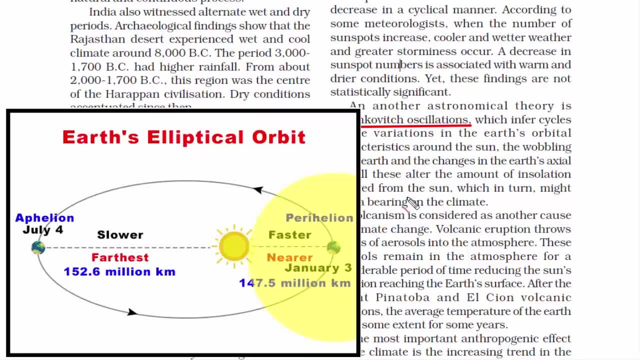 january and incoming solar energy is january and incoming solar energy is less, slightly less on 4th july of every less, slightly less on 4th july of every less, slightly less on 4th july of every year. now, obviously, this is not a very 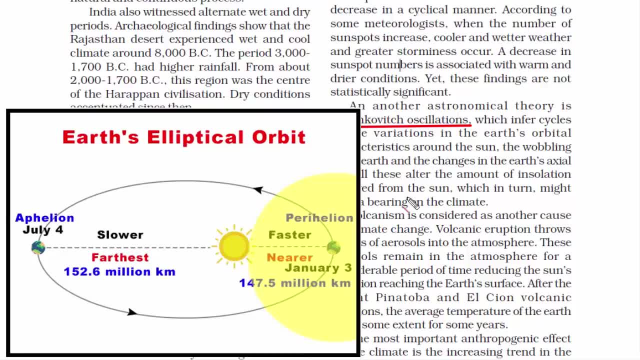 year now. obviously this is not a very year now. obviously this is not a very big variation that you and i can feel big variation, that you and i can feel big variation, that you and i can feel. this is the theory part in reality we. this is the theory part in reality we. 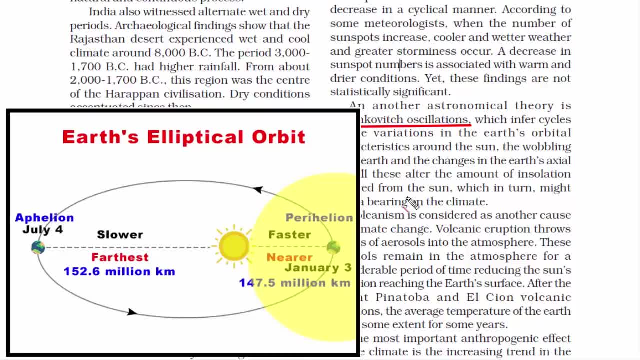 this is the theory part. in reality, we will not see the effect. i mean on july, will not see the effect. i mean on july, will not see the effect, i mean on july 4th. you will not feel that the heat is 4th. you will not feel that the heat is. 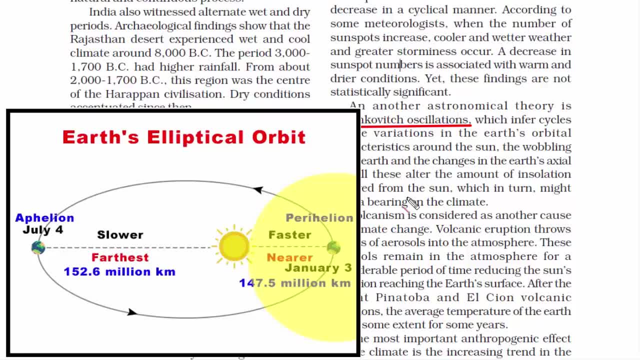 4th you will not feel that the heat is less, or maybe 3rd january you will not less. or maybe 3rd january you will not less. or maybe 3rd january you will not feel that the day is very warm. 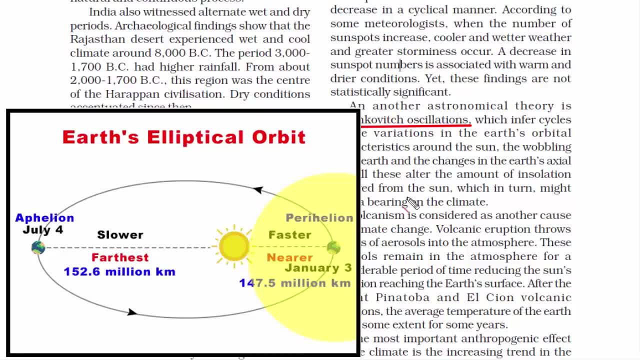 feel that the day is very warm, feel that the day is very warm because there are many factors in the, because there are many factors in the, because there are many factors in the atmosphere that hides the effect of atmosphere, that hides the effect of atmosphere, that hides the effect of insulation caused by aphelion and 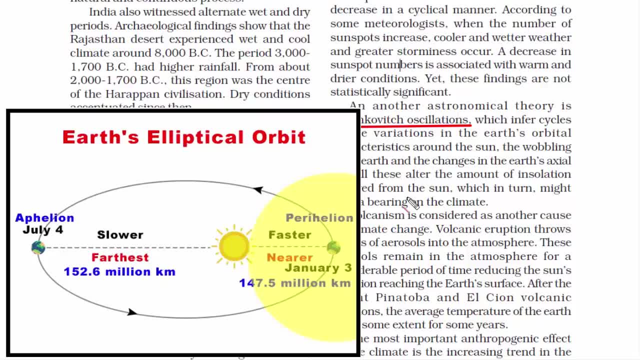 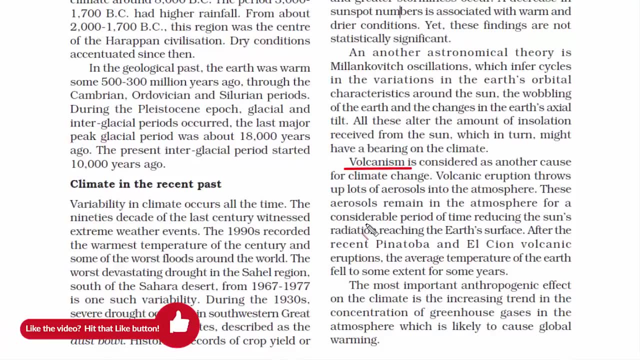 insulation caused by aphelion and insulation caused by aphelion and perihelion: perihelion, perihelion. third factor is volcanism. so i want you. third factor is volcanism, so i want you. third factor is volcanism, so i want you to pause the video and guess under which. 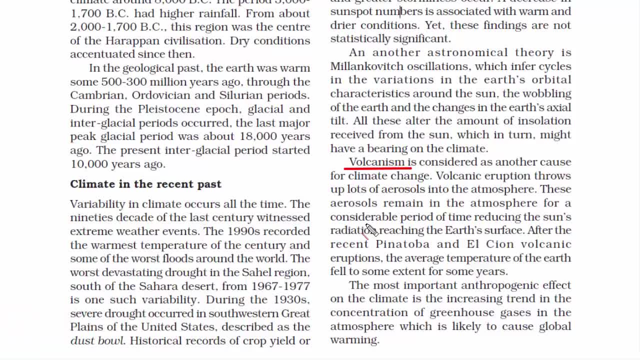 to pause the video and guess under which. to pause the video and guess under which category it falls. category it falls. category it falls: is it astronomical or terrestrial, all? is it astronomical or terrestrial all? is it astronomical or terrestrial? all right, i'm guessing that your answer right? i'm guessing that your answer. 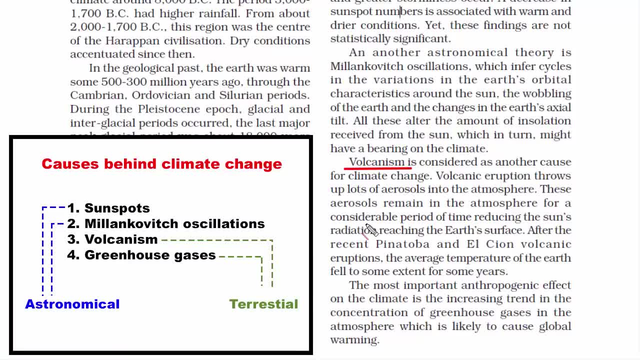 right? i'm guessing that your answer would be terrestrial, would be terrestrial, would be terrestrial. so volcano exists on the surface of the, so volcano exists on the surface of the, so volcano exists on the surface of the earth, and terrestrial means something earth and terrestrial means something earth and terrestrial means something that is related to earth. 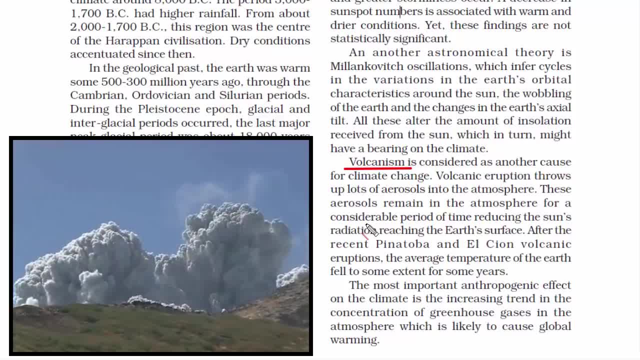 that is related to earth. that is related to earth now. we all must have seen a volcanic now. we all must have seen a volcanic now we all must have seen a volcanic eruption. i mean not in literal sense, but eruption. i mean not in literal sense, but eruption. i mean not in literal sense, but we must have watched it on tv or the. 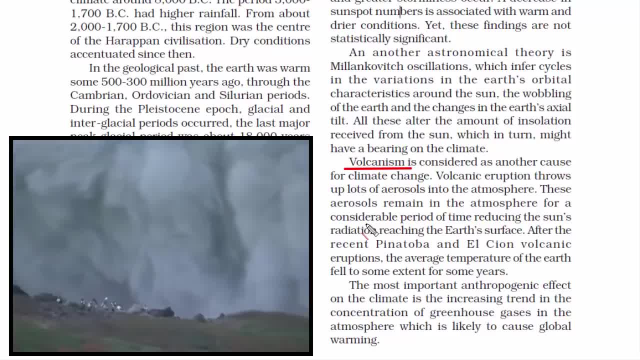 we must have watched it on tv or the. we must have watched it on tv or the internet, internet, internet. so volcanic eruption throws up lots of. so volcanic eruption throws up lots of. so volcanic eruption throws up lots of aerosols into the atmosphere. aerosols into the atmosphere. 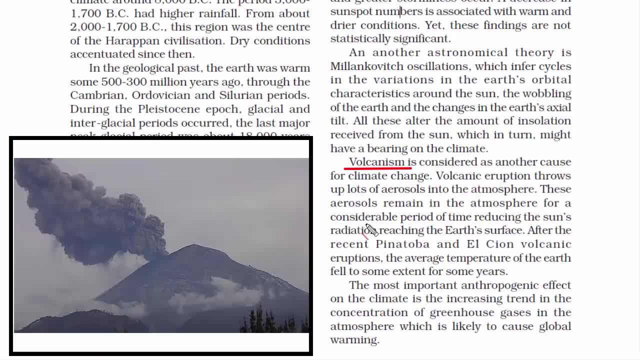 aerosols into the atmosphere, and these aerosols remain in the. and these aerosols remain in the. and these aerosols remain in the atmosphere for a long period of time. atmosphere for a long period of time. atmosphere for a long period of time, and causes dull and gray sky. 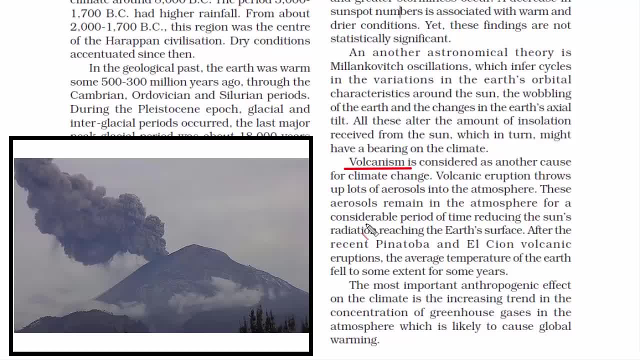 and causes dull and gray sky. and causes dull and gray sky. if the sky is not clear, then it will. if the sky is not clear, then it will. if the sky is not clear, then it will definitely block incoming solar radiation, definitely block incoming solar radiation, definitely block incoming solar radiation. so this question might come in your 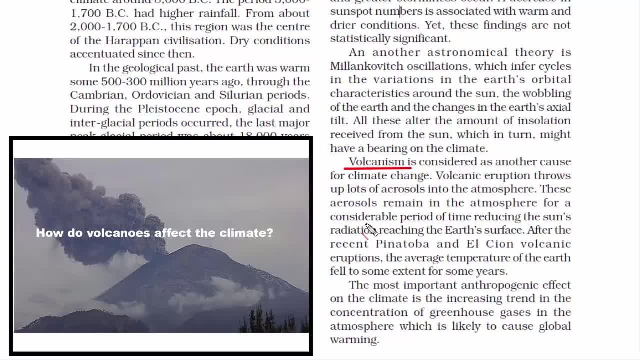 so this question might come in your, so this question might come in your exam. how do volcanoes affect the climate exam. how do volcanoes affect the climate exam? how do volcanoes affect the climate? then you should immediately think of, then you should immediately think of, then you should immediately think of volcanic eruption. when volcanoes erupt. 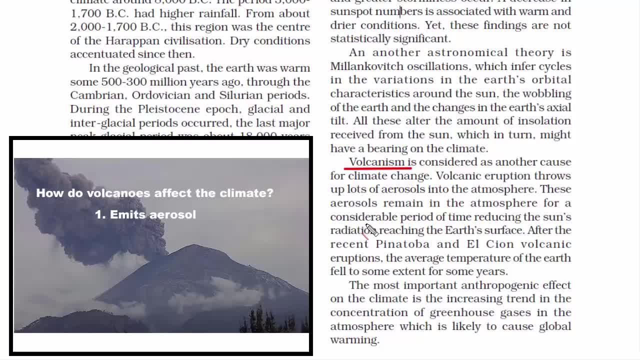 volcanic eruption. when volcanoes erupt. volcanic eruption, when volcanoes erupt, they emit mixtures of gases and they emit mixtures of gases, and they emit mixtures of gases and particles into the air, which are called particles into the air, which are called particles into the air, which are called aerosol. 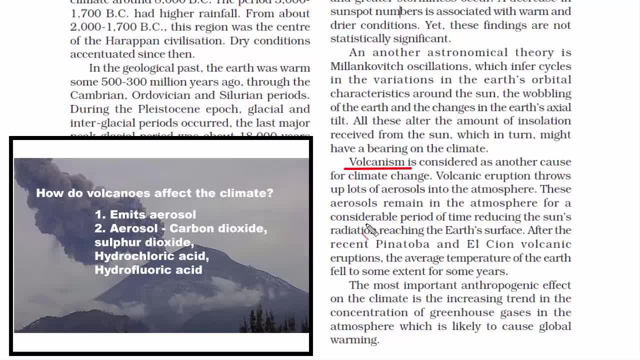 aerosol aerosol. these aerosol includes carbon dioxide. these aerosol includes carbon dioxide. these aerosol includes carbon dioxide, sulphur dioxide, hydrochloric acid, sulphur dioxide, hydrochloric acid, sulphur dioxide, hydrochloric acid, hydrofluoric acid and all of these mineral. 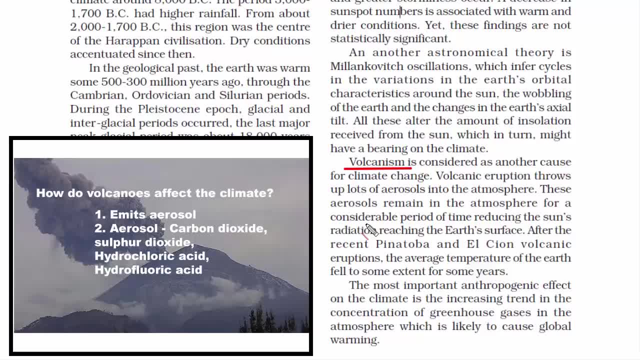 hydrofluoric acid and all of these mineral hydrofluoric acid and all of these mineral particles have serious effect on particles, have serious effect on particles. have serious effect on human health. if exposed, in fact, they can human health. if exposed, in fact, they can. human health. if exposed, in fact, they can also poison lakes and rivers turning. 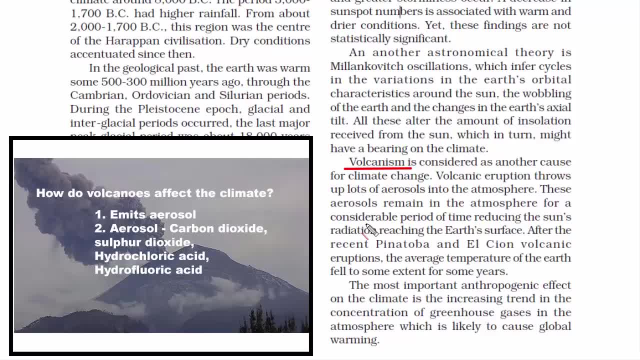 also poison lakes and rivers, turning also poison lakes and rivers, turning them into pools of burning acid. that can them into pools of burning acid. that can them into pools of burning acid that can dissolve all marine organisms, dissolve all marine organisms, dissolve all marine organisms. and i also said that these aerosols 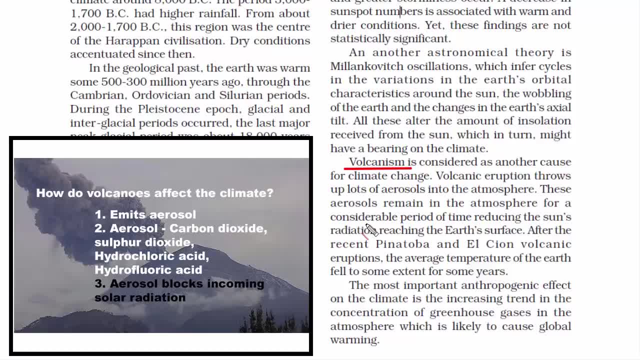 and i also said that these aerosols, and i also said that these aerosols remain in the atmosphere for a long, remain in the atmosphere for a long, remain in the atmosphere for a long period of time, period of time, period of time, and then it blocks incoming solar 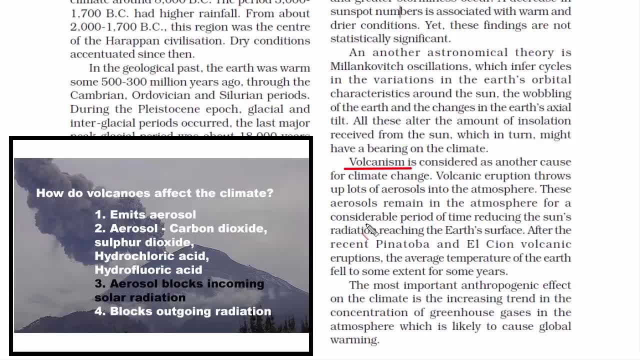 and then it blocks incoming solar, and then it blocks incoming solar radiation. similarly, it also blocks the radiation. similarly, it also blocks the radiation. similarly, it also blocks the outgoing radiation. outgoing radiation, outgoing radiation. all of this becomes a defining factor. all of this becomes a defining factor. all of this becomes a defining factor for climate change. 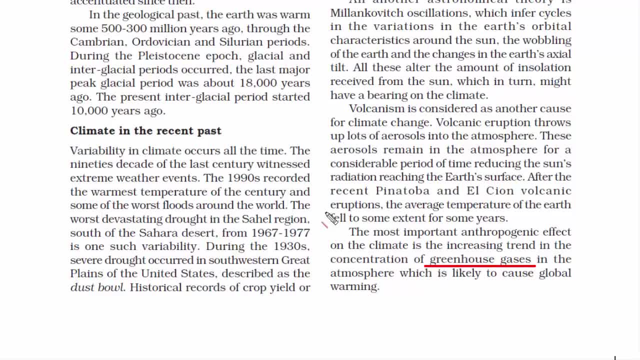 for climate change. for climate change, and the last factor is increase in the, and the last factor is increase in the, and the last factor is increase in the concentration of greenhouse gases, in the concentration of greenhouse gases, in the concentration of greenhouse gases in the atmosphere, atmosphere, atmosphere. now greenhouse gases are basically. i'll. 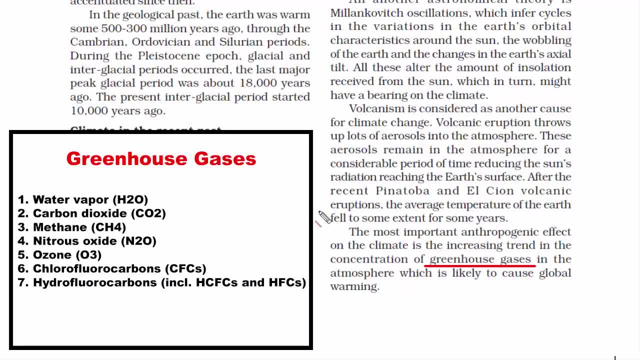 now greenhouse gases are basically. i'll now greenhouse gases are basically. i'll just put all the gases, just put all the gases, just put all the gases. that falls under the greenhouse gas, just that falls under the greenhouse gas, just that falls under the greenhouse gas. just pause the video and have a look at it. pause the video and have a look at it. pause the video and have a look at it now. these are bunch of gases in the now. these are bunch of gases in the now. these are bunch of gases in the atmosphere that blocks the earth's atmosphere. that blocks the earth's. 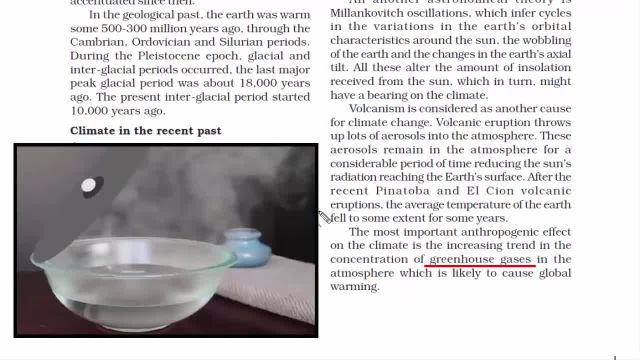 atmosphere that blocks the earth's radiation from going out in the space, radiation from going out in the space, radiation from going out in the space. these greenhouse gas traps the heat. these greenhouse gas traps the heat. these greenhouse gas traps the heat within the earth's atmosphere and makes 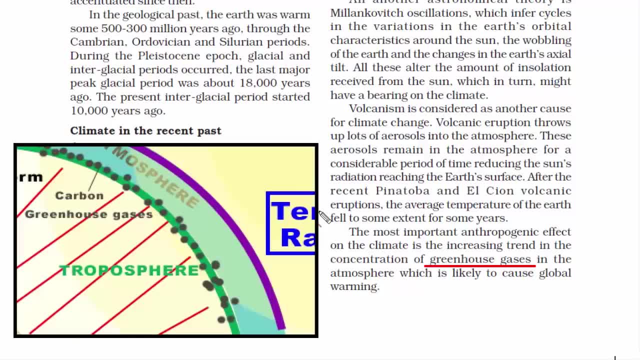 within the earth's atmosphere and makes within the earth's atmosphere and makes the earth warmer, the earth warmer, the earth warmer. now the interesting part to note is that now the interesting part to note is that now the interesting part to note is that the volume of other gases is constant. 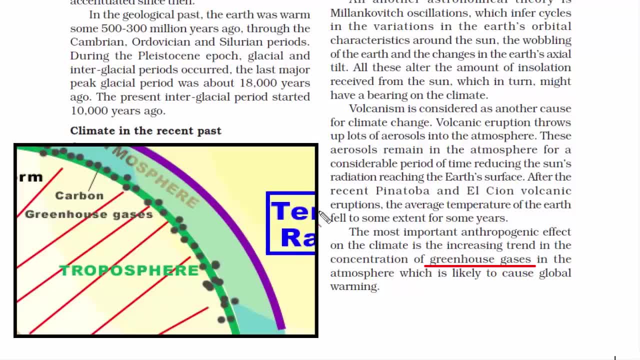 the volume of other gases is constant. the volume of other gases is constant, but the volume of carbon dioxide has. but the volume of carbon dioxide has. but the volume of carbon dioxide has been rising in the past few decades, been rising in the past few decades. been rising in the past few decades mainly because of the burning of fossil. 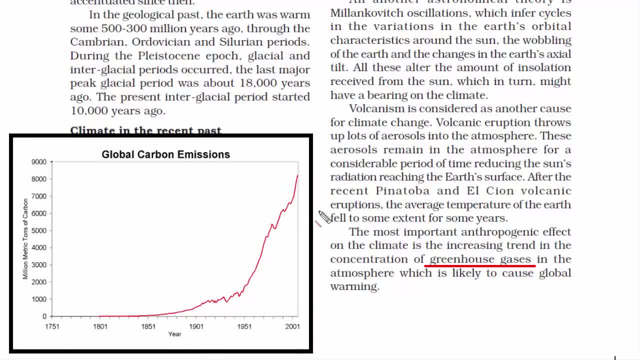 mainly because of the burning of fossil, mainly because of the burning of fossil fuels, fuels, fuels since the industrial revolution, that is, since the industrial revolution, that is, since the industrial revolution, that is, from mid 18th century, the amount of from mid 18th century, the amount of. 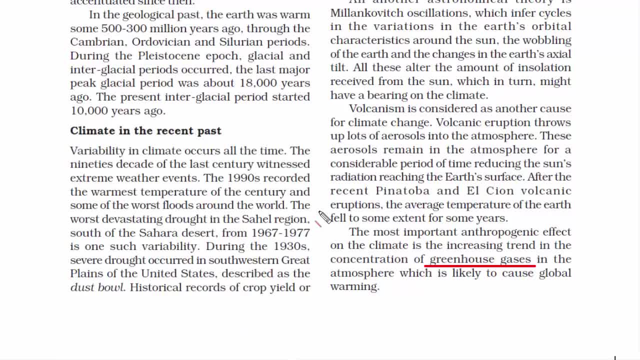 from mid 18th century, the amount of carbon dioxide has increased. machines on carbon dioxide has increased. machines on carbon dioxide has increased. machines on daily basis are using fossil fuels like daily basis, are using fossil fuels like daily basis, are using fossil fuels like diesel, petrol and that's emitting more. 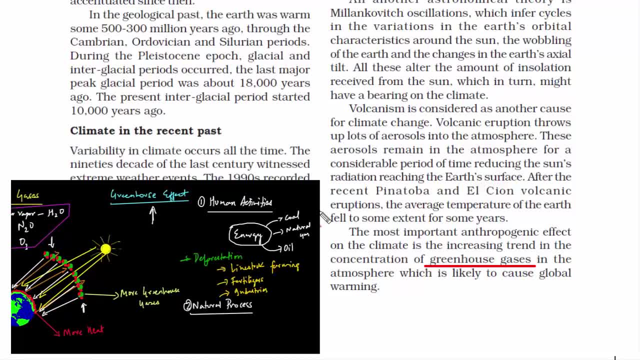 diesel petrol and that's emitting more diesel petrol and that's emitting more video on it as well. i'll put the link of video on it as well. i'll put the link of video on it as well. i'll put the link of that video in the description, just have. 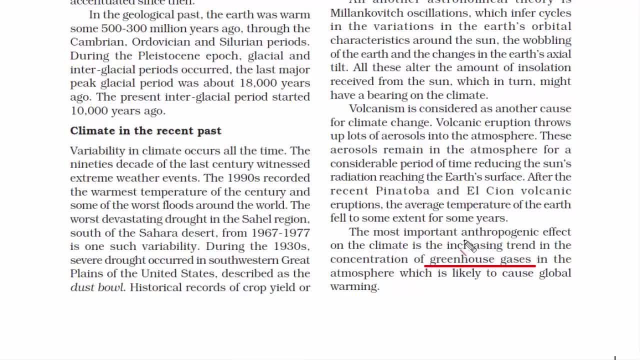 that video in the description. just have that video in the description. just have a look at it, a look at it, a look at it. so if you read here, it says it is an. so if you read here, it says it is an. so if you read here, it says it is an anthropogenic effect. anthropogenic is. 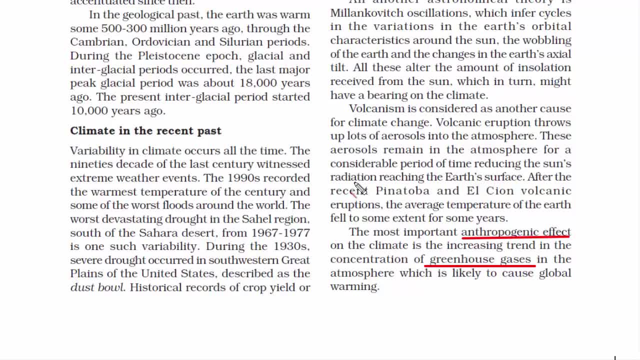 anthropogenic effect. anthropogenic is anthropogenic effect. anthropogenic is related to environmental pollution, that related to environmental pollution, that related to environmental pollution. that occurs due to human activity. so occurs due to human activity. so occurs due to human activity. so basically, it's a terrestrial cause. 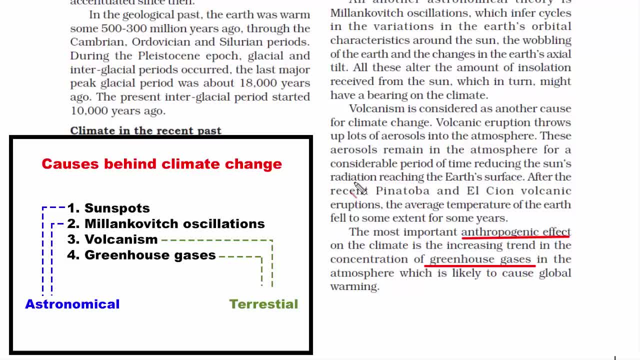 basically, it's a terrestrial cause, alright. so with this we have completed. alright. so with this we have completed alright. so with this we have completed the four main factors that causes climate, the four main factors that causes climate, the four main factors that causes climate change, change, change. actually, we are pretty much done with 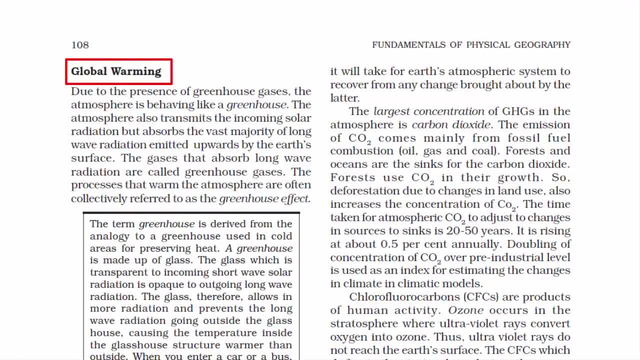 actually we are pretty much done with. actually, we are pretty much done with this chapter, except for this last topic. this chapter, except for this last topic, this chapter, except for this last topic: global warming, global warming, global warming. even this topic includes matter that i've. even this topic includes matter that i've. 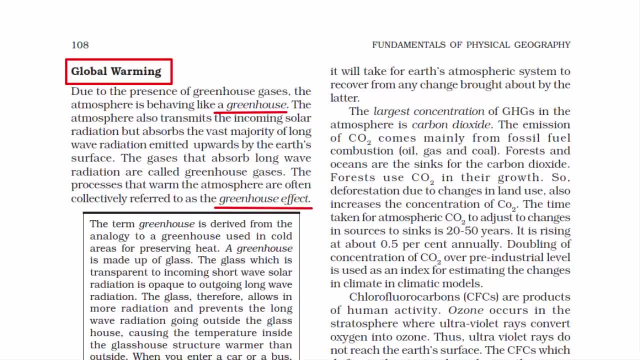 even this topic includes matter that i've already covered in this chapter, already covered in this chapter, already covered in this chapter. moments back i told you about greenhouse. moments back i told you about greenhouse. moments back i told you about greenhouse gases, gases, gases. then i also have a separate video on it. 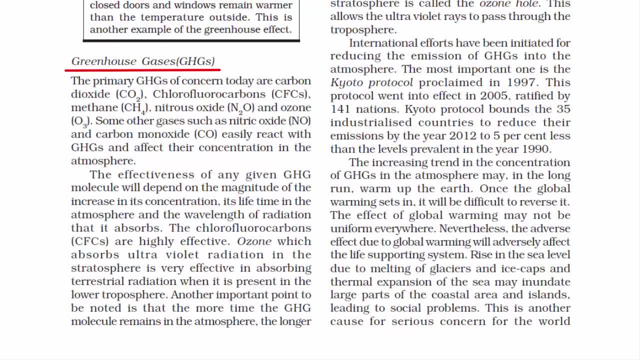 then i also have a separate video on it. then i also have a separate video on it. i have put the link in the description. i have put the link in the description. i have put the link in the description. then i've also spoken about climate. then i've also spoken about climate. 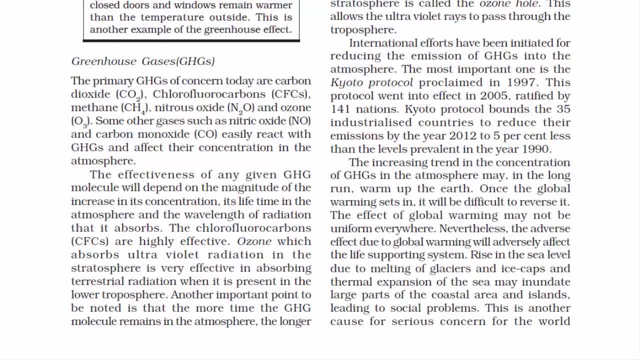 then i've also spoken about climate change: how it blocks the incoming solar change. how it blocks the incoming solar change. how it blocks the incoming solar radiation, as well as outgoing earth's radiation, as well as outgoing earth's radiation, as well as outgoing earth's radiation radiation. 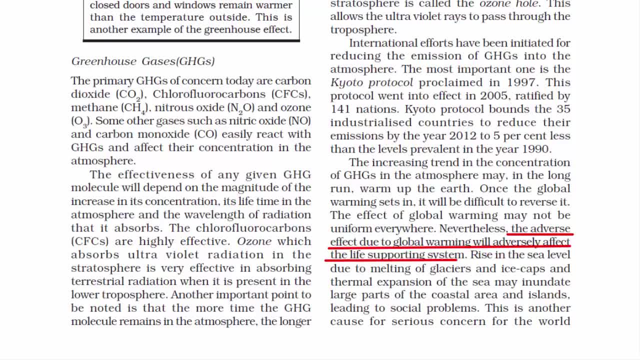 radiation. but this thing over here global warming. but this thing over here global warming, but this thing over here global warming adversely affects the life supporting, adversely affects the life supporting, adversely affects the life supporting system, system system. now this particular topic is something. now this particular topic is something. 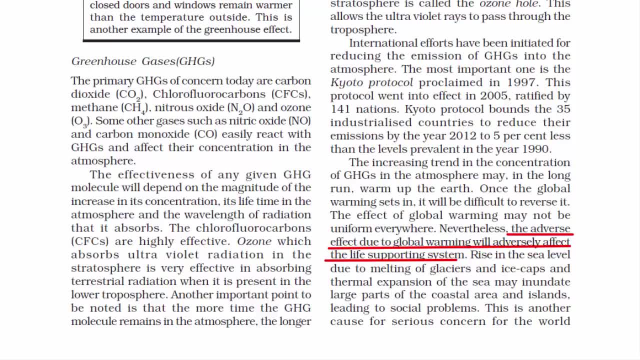 now, this particular topic is something that i feel is very important. because that i feel is very important, because that i feel is very important, because, if i have to rephrase this question, how? if i have to rephrase this question, how, if i have to rephrase this question, how does climate change affects humans and 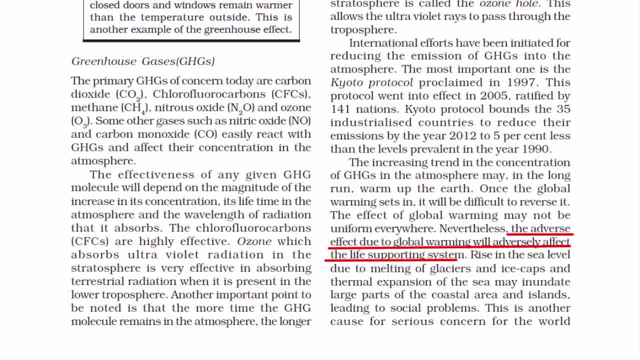 does climate change affects humans and does climate change affects humans and nations both socially and economically, nations both socially and economically, nations both socially and economically? so that will be the bottom line question. so that will be the bottom line question. so that will be the bottom line question, if i have to rephrase it. 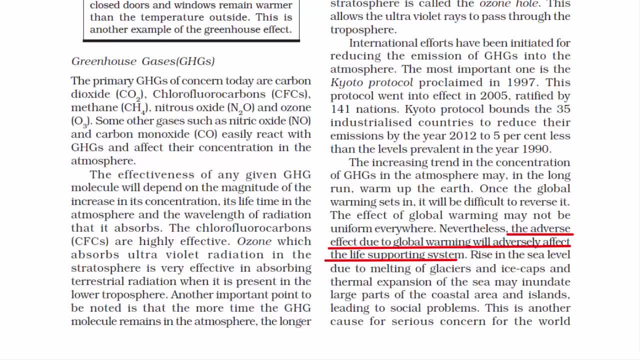 if i have to rephrase it, if i have to rephrase it. so what i'm going to do is i will. so what i'm going to do is i will. so what i'm going to do is i will quickly explain this. i already have a. 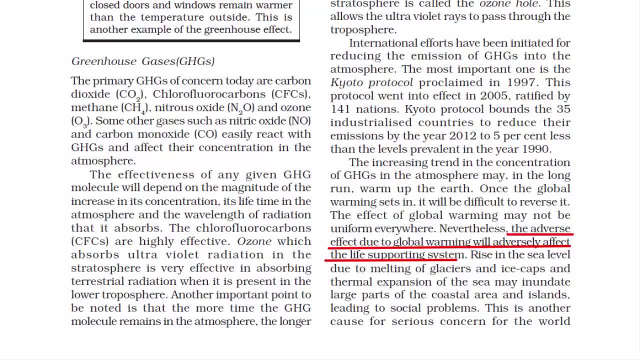 quickly explain this. i already have a quickly explain this. i already have a recorded version of this particular recorded version of this particular recorded version of this particular topic that i have spoken in the past topic that i have spoken in the past, topic that i have spoken in the past. i will simply put that clip and i want 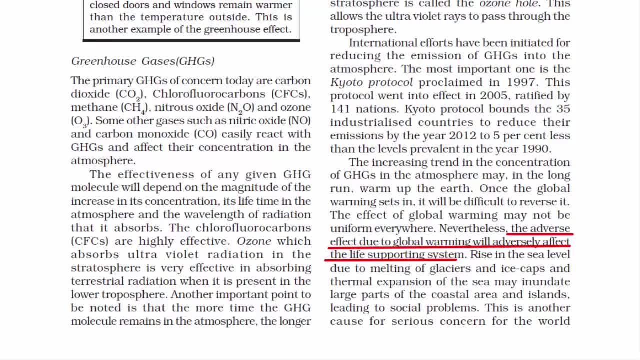 i will simply put that clip and i want i will simply put that clip and i want you to listen to it, and you will get you to listen to it, and you will get you to listen to it, and you will get everything, everything, everything. so here we go, let's get to know about. 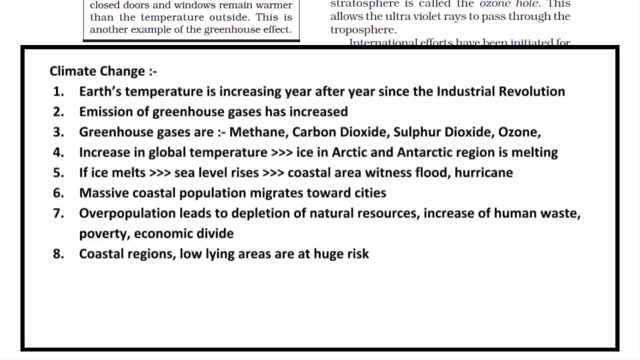 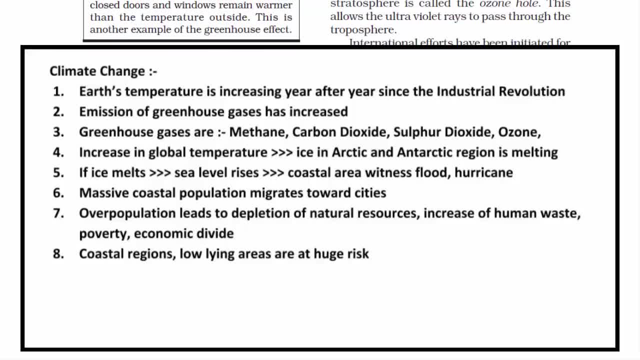 story or a hoax. it's. it's a reality story or a hoax, it's. it's a reality, and by climate change we mean that earth's, and by climate change we mean that earth's. and by climate change we mean that earth's temperature is going up year by year. 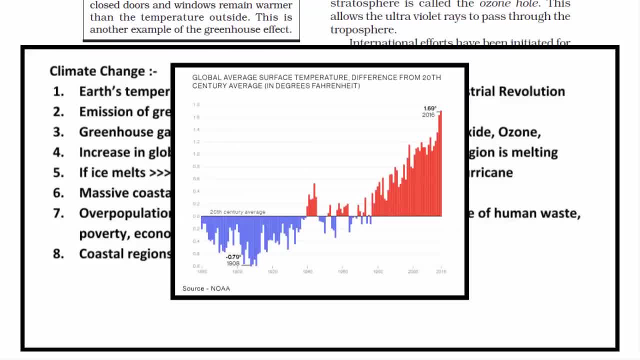 temperature is going up year by year. temperature is going up year by year. so since the industrial revolution, the so since the industrial revolution, the so since the industrial revolution, the temperature of earth has gone up, like temperature of earth has gone up. like temperature of earth has gone up like anything. industrial revolution gave birth. 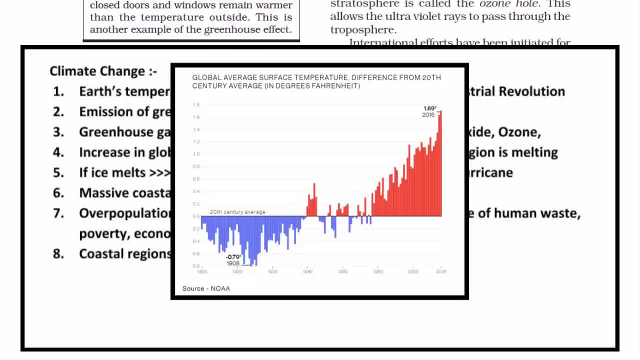 anything industrial revolution gave birth. anything industrial revolution gave birth to machines and machines are very to machines and machines are very to machines, and machines are very important aspect of our day-to-day life, important aspect of our day-to-day life, important aspect of our day-to-day life. it helps us a lot but it consumes fossil. 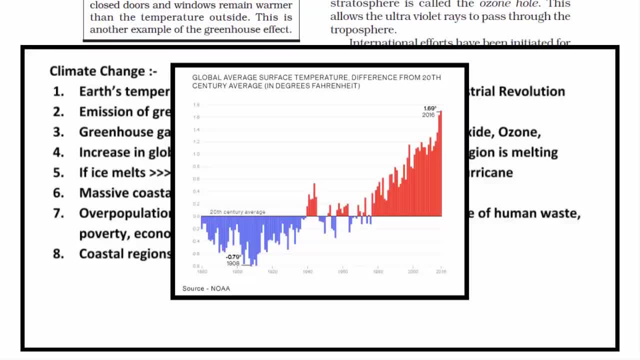 it helps us a lot, but it consumes fossil. it helps us a lot, but it consumes fossil fuel and, due to fossil fuel, greenhouse fuel and due to fossil fuel, greenhouse fuel and due to fossil fuel, greenhouse gas emission has increased. now what are? gas emission has increased. now, what are? 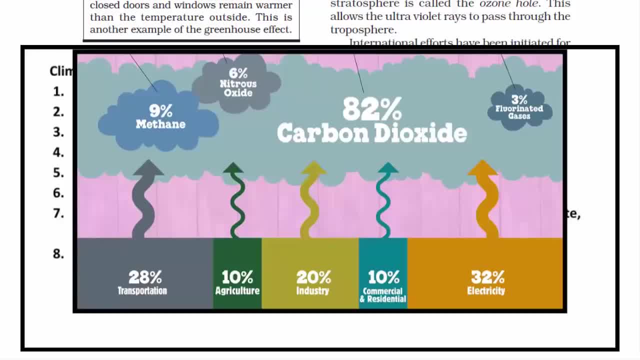 gas emission has increased. now, what are these greenhouse gases? we are talking these greenhouse gases. we are talking these greenhouse gases. we are talking about carbon dioxide, methane, nitrous. about carbon dioxide, methane, nitrous. about carbon dioxide, methane, nitrous, oxide ozone, then sulfur dioxide all. oxide ozone, then sulfur dioxide all. 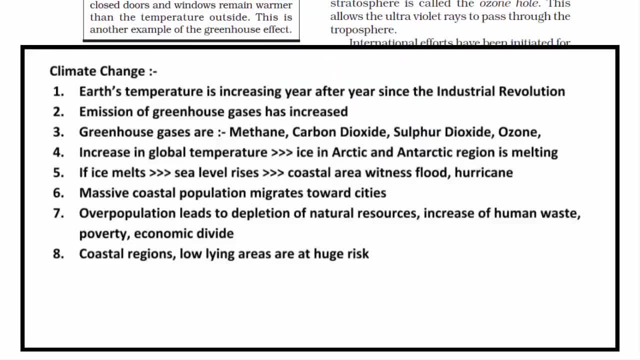 oxide, ozone, then sulfur dioxide- all these are called greenhouse gases. now, these are called greenhouse gases. now, these are called greenhouse gases. now, the thing that these greenhouse gases do, the thing that these greenhouse gases do, the thing that these greenhouse gases do, is that it blocks the earth's 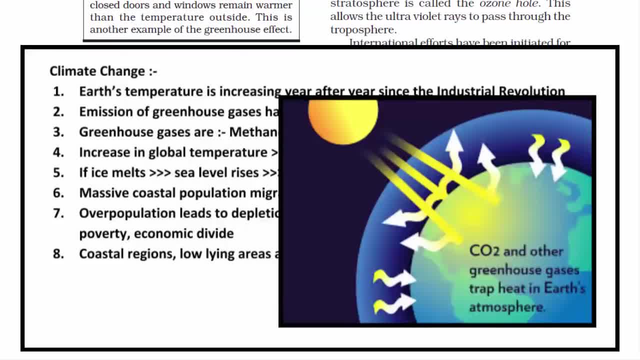 is that it blocks the earth's, is that it blocks the earth's temperature meaning. temperature meaning, temperature meaning. so the sun rays come inside the earth's, so the sun rays come inside the earth's, so the sun rays come inside the earth's atmosphere and that's what keeps us warm. atmosphere and that's what keeps us warm. atmosphere and that's what keeps us warm. if there is no sun rays, then we would. if there is no sun rays, then we would. if there is no sun rays, then we would have been frozen like anything. so have been frozen like anything, so. 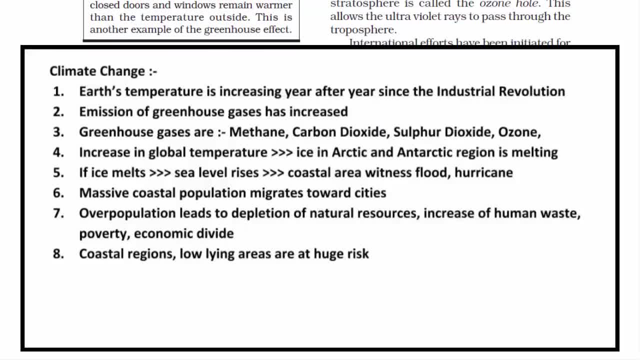 have been frozen like anything. so sun rays are good, but the thing is that sun rays are good, but the thing is that sun rays are good, but the thing is that when the earth's surface gets heated, the when the earth's surface gets heated, the when the earth's surface gets heated, the heat does not go out of the atmosphere. 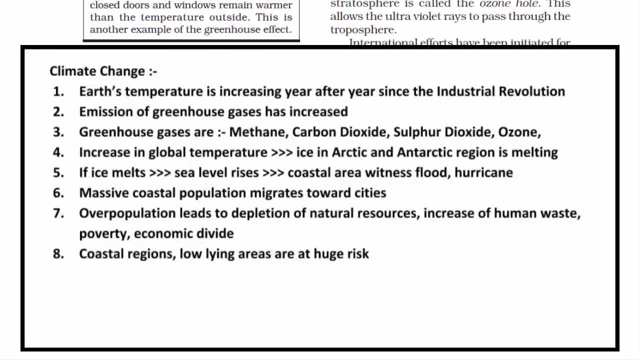 heat does not go out of the atmosphere. heat does not go out of the atmosphere, it gets trapped, and it is because of it gets trapped, and it is because of it gets trapped and it is because of greenhouse gases and, over time, what greenhouse gases and, over time, what? 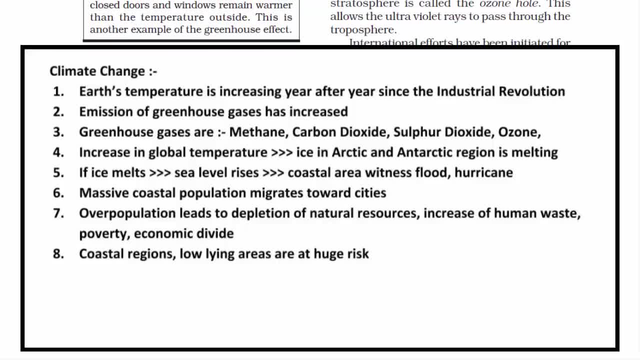 greenhouse gases and, over time, what happens is the temperature of the earth. happens is the temperature of the earth happens is the temperature of the earth increases. it's like a pressure cooker. if increases, it's like a pressure cooker. if increases, it's like a pressure cooker. if it is closed from all end, the steam is. 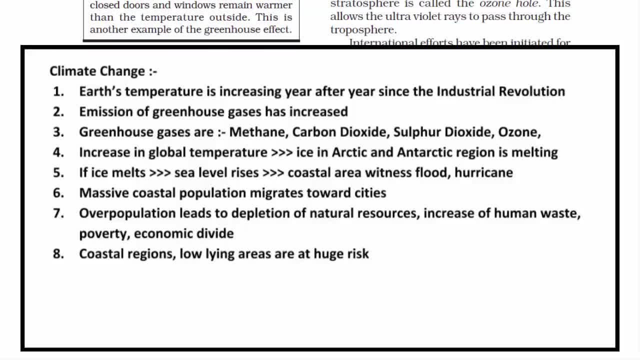 it is closed from all end. the steam is. it is closed from all end. the steam is inside, and if there is no way for the inside and if there is no way for the inside and if there is no way for the steam to go out, the temperature inside. 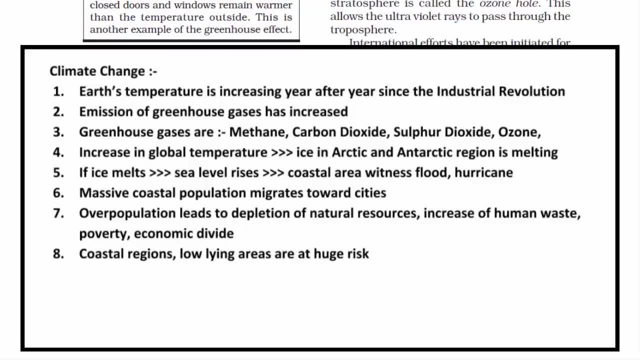 steam to go out, the temperature inside steam to go out, the temperature inside increases, increases, increases. so today, if you see everyone's focus is so today, if you see everyone's focus is so today, if you see everyone's focus is on carbon dioxide, everyone is trying to. 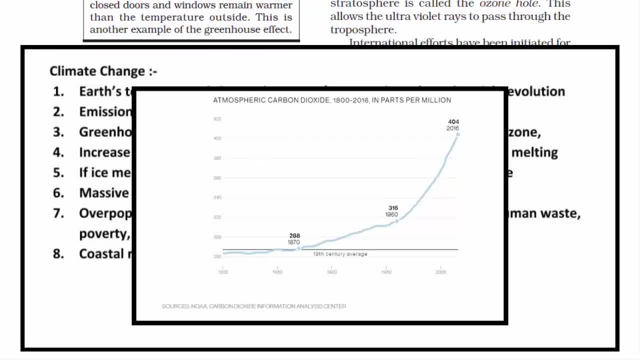 on carbon dioxide. everyone is trying to on carbon dioxide. everyone is trying to reduce carbon emission. and why? because reduce carbon emission. and why? because reduce carbon emission. and why? because we modern humans have produced it and we modern humans have produced it and we modern humans have produced it and making it the largest greenhouse gas and 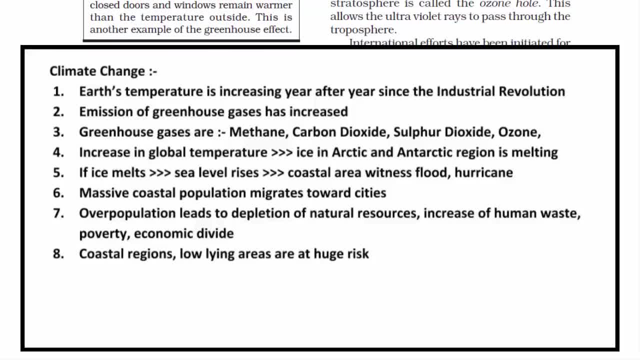 making it the largest greenhouse gas and making it the largest greenhouse gas, and i've given you the reason because of i've given you the reason because of i've given you the reason because of burning fossil fuels and another thing: burning fossil fuels. and another thing: burning fossil fuels- and another thing that is happening is deforestation. that 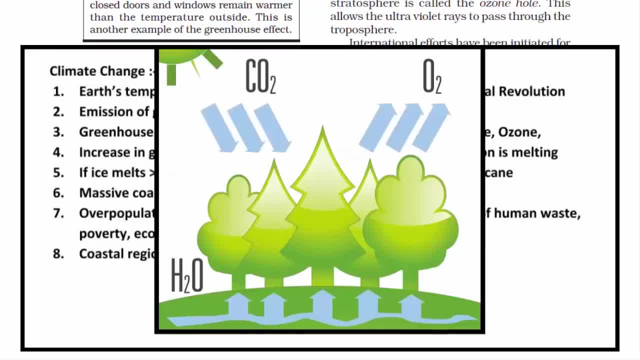 that is happening is deforestation. that that is happening is deforestation. that is cutting down forest cover. is cutting down forest cover, is cutting down forest cover. so i hope you know the role of trees, so i hope you know the role of trees. so i hope you know the role of trees. right, they take in the carbon dioxide. 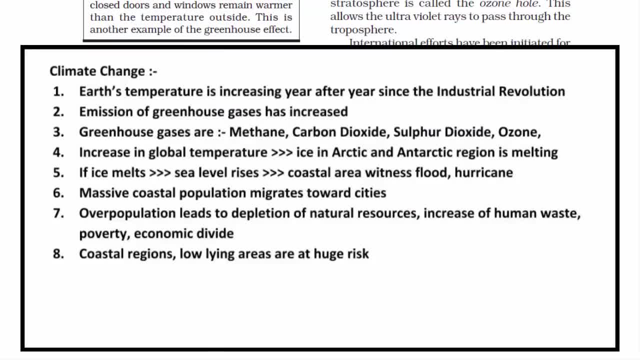 right, they take in the carbon dioxide. right, they take in the carbon dioxide and they throw out oxygen for us, and they throw out oxygen for us, and they throw out oxygen for us. so just think about it, we are increasing. so just think about it, we are increasing. 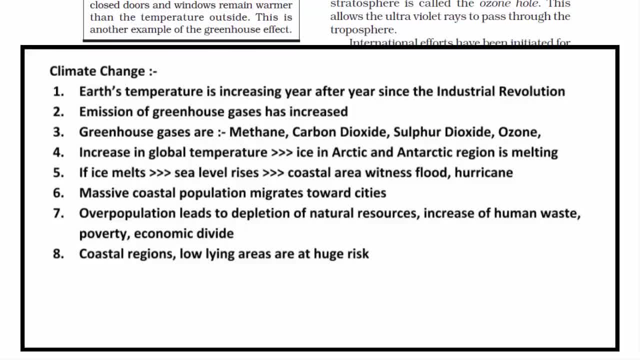 so just think about it: we are increasing the carbon content, and then we are also the carbon content, and then we are also the carbon content, and then we are also cutting down forest. it's a vicious cycle cutting down forest. it's a vicious cycle, cutting down forest. it's a vicious cycle, all right. so this was the initial story. 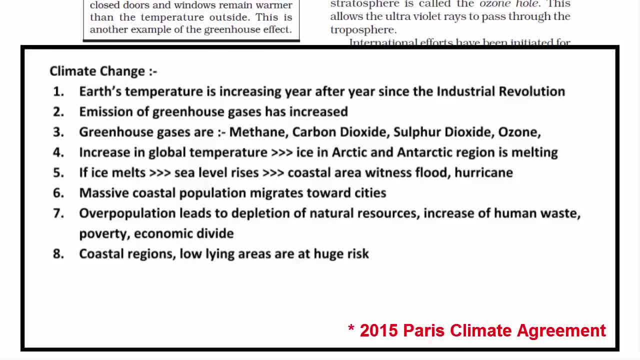 all right, so this was the initial story. all right, so this was the initial story of climate change, of climate change, of climate change. now last year, during paris climate deal, now last year during paris climate deal, now last year during paris climate deal, it was suggested that let's keep the 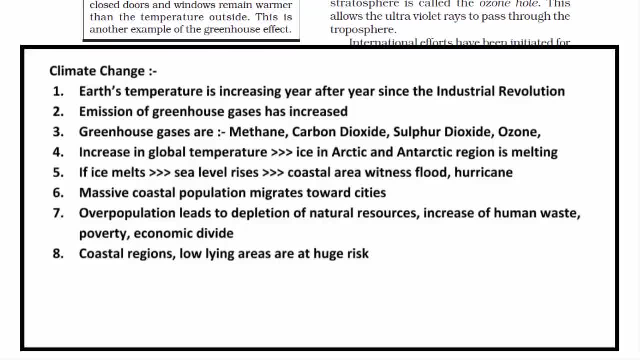 it was suggested that let's keep the. it was suggested that let's keep the melt, and that's going to cause a big melt, and that's going to cause a big melt, and that's going to cause a big tragedy, tragedy, tragedy. so the plan is to keep the global. 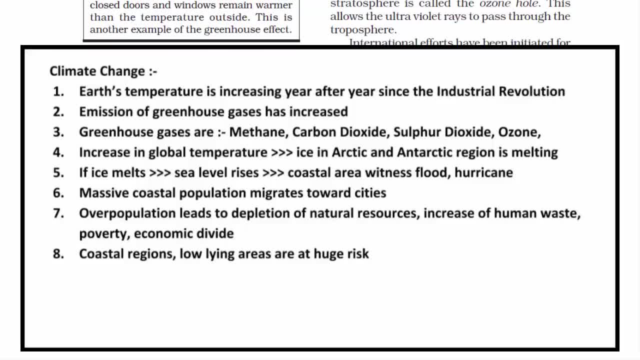 so the plan is to keep the global. so the plan is to keep the global average temperature low average temperature. low average temperature low. now people don't understand when now people don't understand when now people don't understand when scientists talk about one or two degree. scientists talk about one or two degree. 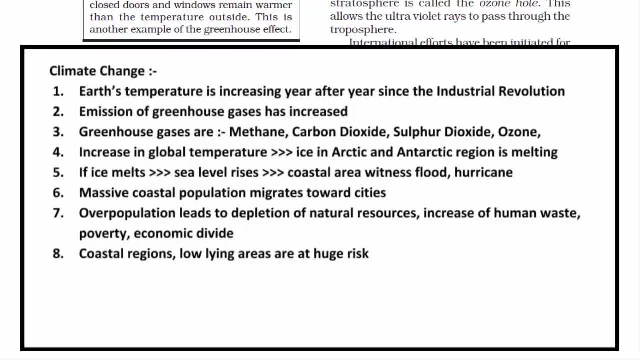 scientists talk about one or two degree increase in temperature. people feel that increase in temperature. people feel that increase in temperature. people feel that, uh, it's all right, you know last summer. uh, it's all right, you know last summer. uh, it's all right, you know, last summer it was. 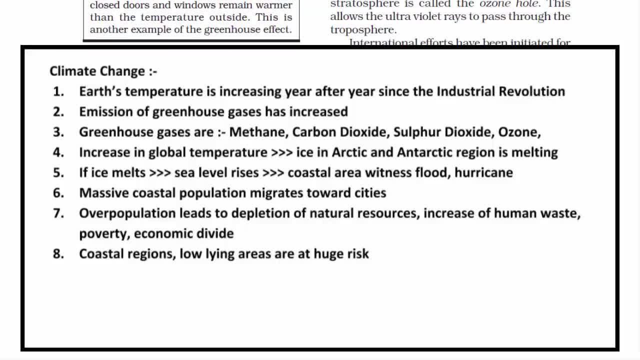 it was, it was 45. today it is 50, it's fine. you know, 45 today it is 50, it is fine. you know 45 today it is 50, it is fine, you know it's it's not a big deal. but then if 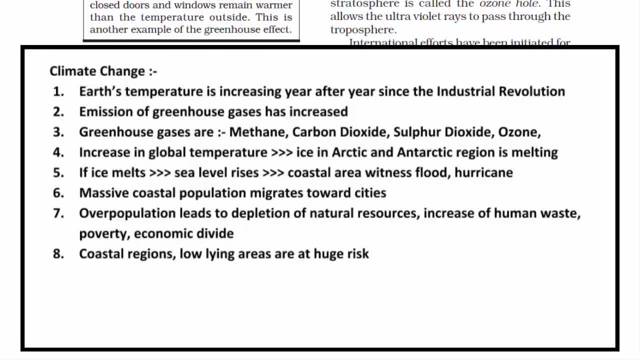 it's, it's not a big deal, but then, if it's, it's not a big deal, but then if you take the entire temperature of the, you take the entire temperature of the, you take the entire temperature of the earth, and then you have to say that it. 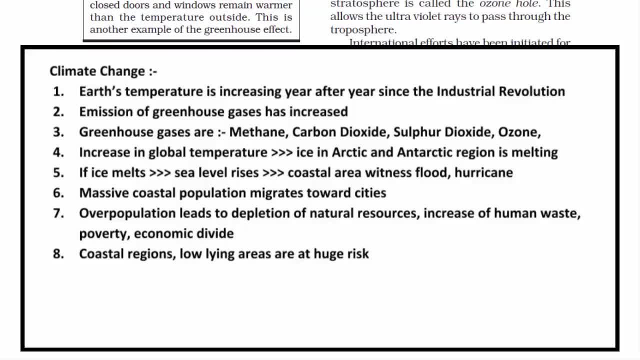 earth, and then you have to say that it earth, and then you have to say that it is going to increase one or two degree, is going to increase one or two degree, is going to increase one or two degree celsius. it's a lot because there are a 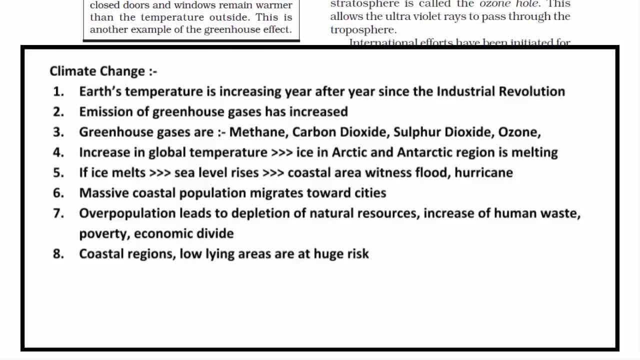 celsius it's a lot, because there are a. celsius, it's a lot because there are a lot of places, then there are a lot of lot of places, then there are a lot of lot of places, then there are a lot of species that cannot live beyond a. 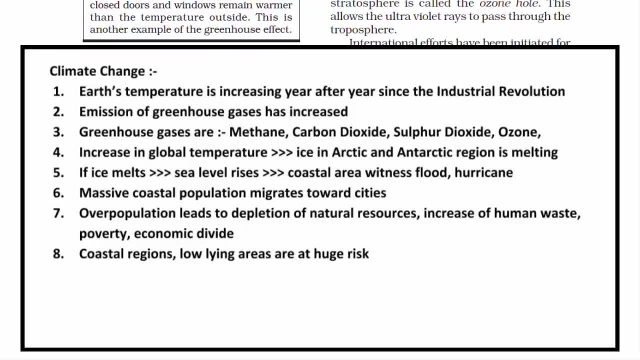 species that cannot live beyond, a species that cannot live beyond a certain temperature, certain temperature, certain temperature. we humans are exception because human, we humans are exception because human, we humans are exception because human beings stay in beings, stay in beings, stay in hot temperature, like like in the african. 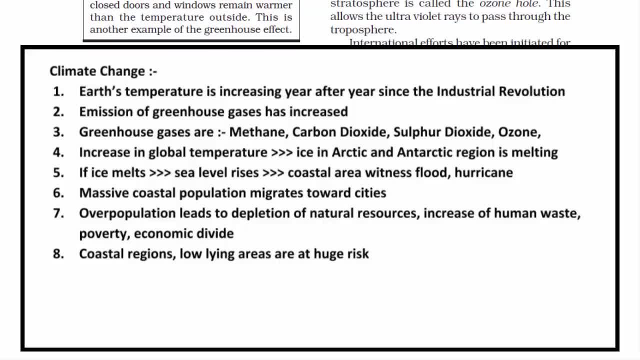 hot temperature, like like in the african hot temperature, like like in the african desert, and then there are human beings desert, and then there are human beings desert, and then there are human beings who are staying in cold temperatures, who are staying in cold temperatures, who are staying in cold temperatures like in siberia, greenland, iceland, all. 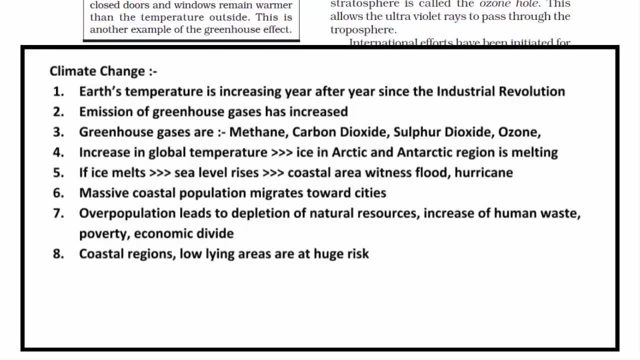 like in siberia, greenland, iceland, all like in siberia, greenland, iceland, all these kind of places, these kind of places, these kind of places, but then there are certain species that, but then there are certain species that, but then there are certain species that cannot live beyond a certain 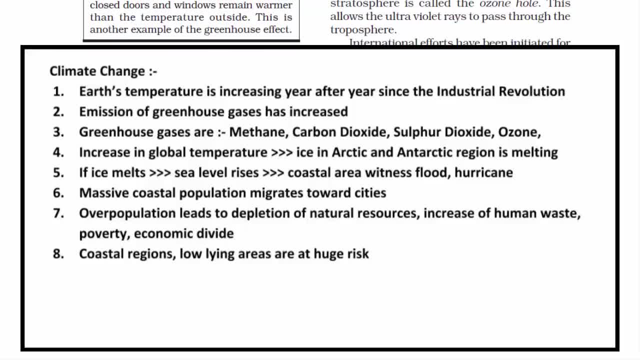 cannot live beyond a certain temperature: temperature, temperature now. the crux of the matter is that. if now the crux of the matter is that, if now the crux of the matter is that if the earth's temperature increases, the earth's temperature increases, the earth's temperature increases, then all the ice in north and south 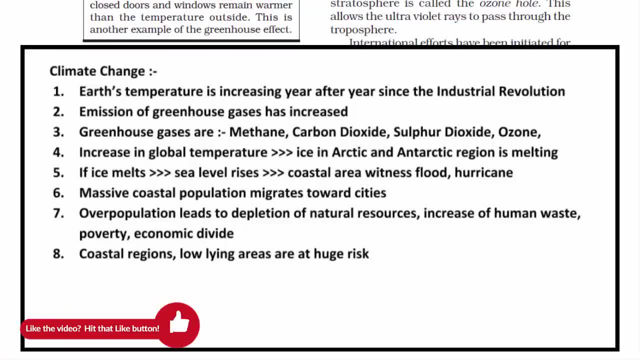 then all the ice in north and south, then all the ice in north and south pole will melt, pole will melt, pole will melt. now what happens when ice melts the sea now, what happens when ice melts the sea? now, what happens when ice melts? the sea level rises. 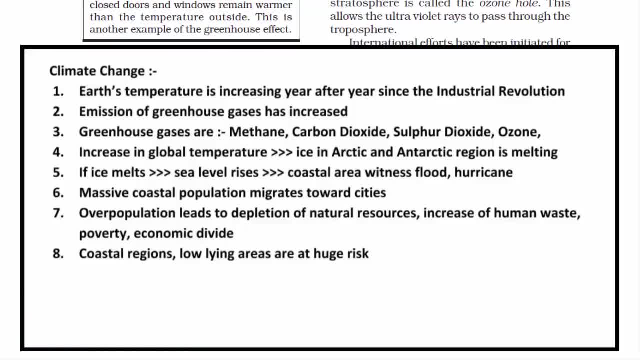 level rises. level rises. it's very simple to understand. when a. it's very simple to understand when a. it's very simple to understand when a big portion of ice melts, then the water. big portion of ice melts, then the water. big portion of ice melts, then the water from that. 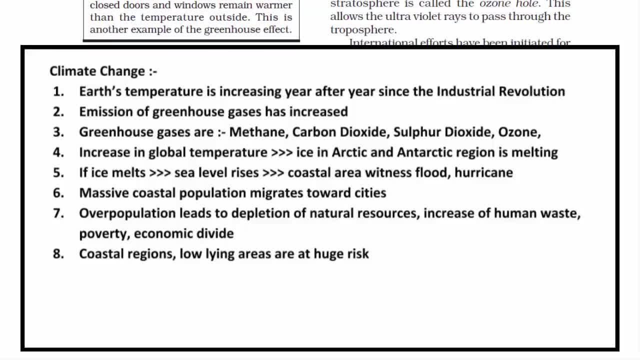 from that, from that ice, it goes into the hydrological cycle. ice it goes into the hydrological cycle. ice it goes into the hydrological cycle, which is the ocean, and when ocean gets, which is the ocean. and when ocean gets, which is the ocean, and when ocean gets more and more water. 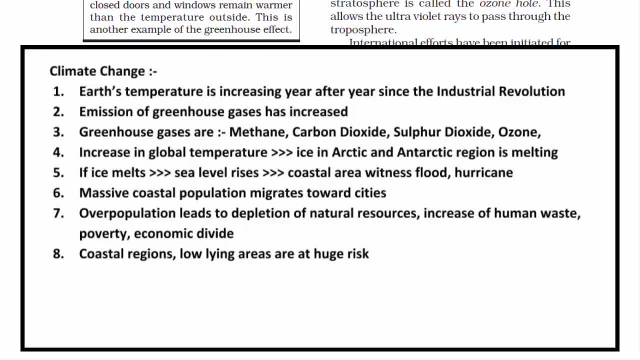 more and more water, more and more water. it increases. and if the level increases, it increases. and if the level increases, it increases. and if the level increases, you know what can happen. right, it will. you know what can happen, right it will. you know what can happen. right. it will cause floods, hurricanes at coastal region. 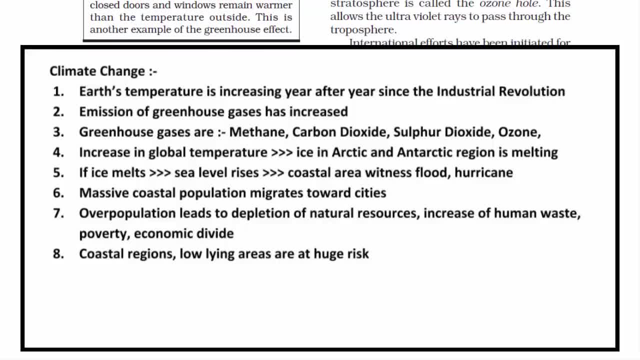 cause floods, hurricanes at coastal region, cause floods, hurricanes at coastal region. so it will cause a massive geographical. so it will cause a massive geographical. so it will cause a massive geographical, social and economical turmoil, social and economical turmoil, social and economical turmoil. so i want you to imagine this scenario. 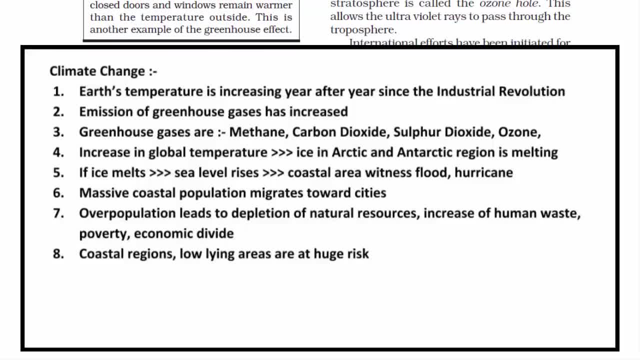 so i want you to imagine this scenario. so i want you to imagine this scenario. suppose you're staying in a coastal area. suppose you're staying in a coastal area. suppose you're staying in a coastal area and there's a rise in sea level, so your. and there's a rise in sea level, so your. 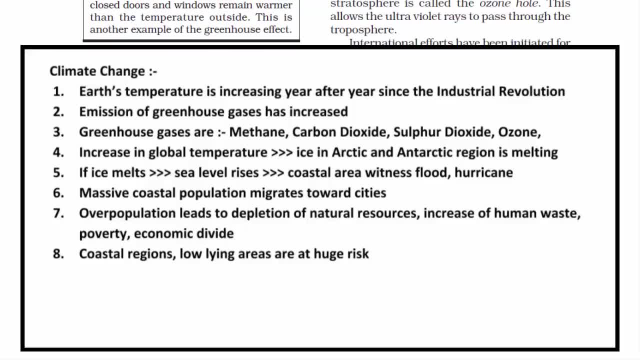 and there's a rise in sea level. so your coastal area is going to hit by flood. coastal area is going to hit by flood, coastal area is going to hit by flood and if flood hits your area, you're going. and if flood hits your area, you're going. 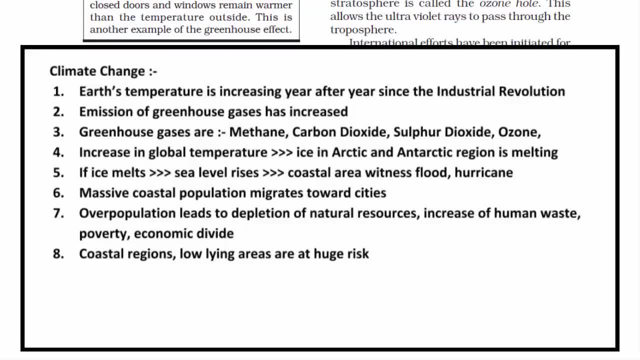 and if flood hits your area, you're going to go towards the plain area. you're to go towards the plain area. you're to go towards the plain area. you're going to move, going to move, going to move a little inside. one good example is a little inside. one good example is: 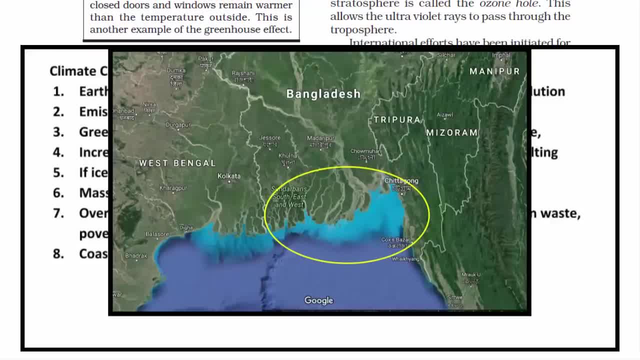 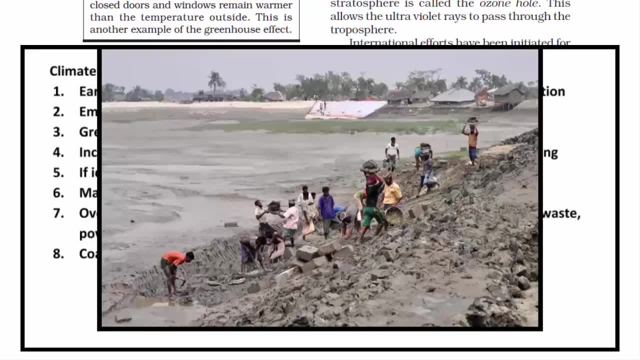 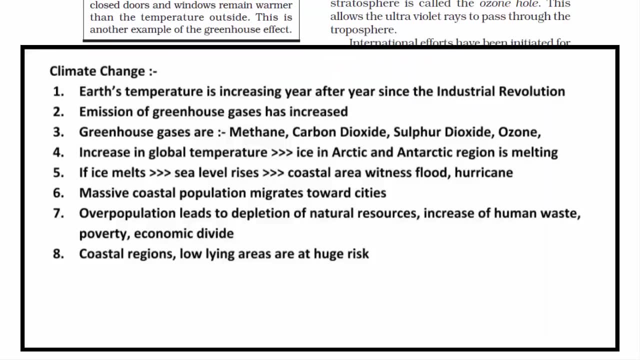 a little inside. one good example is bangladesh, the region near bangladesh, bangladesh, the region near bangladesh, bangladesh, the region near bangladesh, and sundarban area, and sundarban area and sundarban area. these people who have been affected, these people who have been affected. 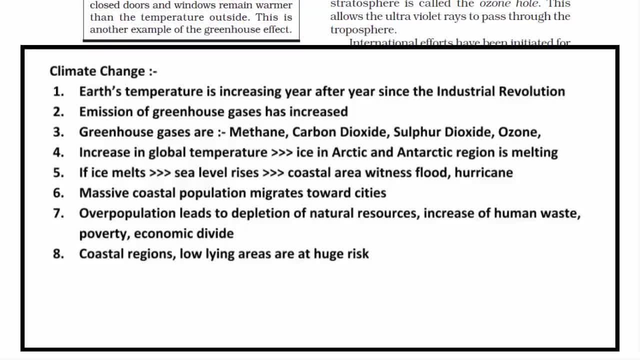 these people who have been affected because of flood. they don't have house because of flood. they don't have house because of flood. they don't have house, they don't have any job. they are, they don't have any job, they are, they don't have any job, they are destitutes. 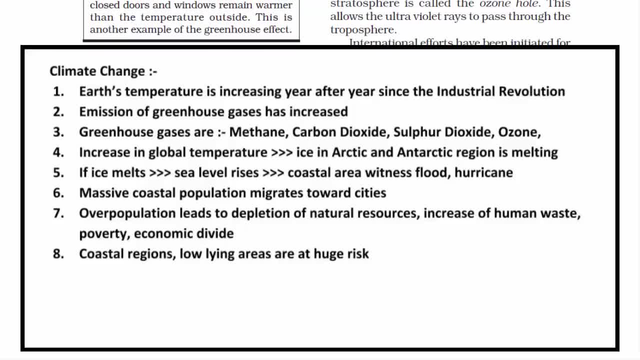 destitutes, destitutes. now, what is going to happen? it's going now. what is going to happen. it's going now. what is going to happen? it's going to increase the population of the city, to increase the population of the city, to increase the population of the city. so, because of this internal migration, 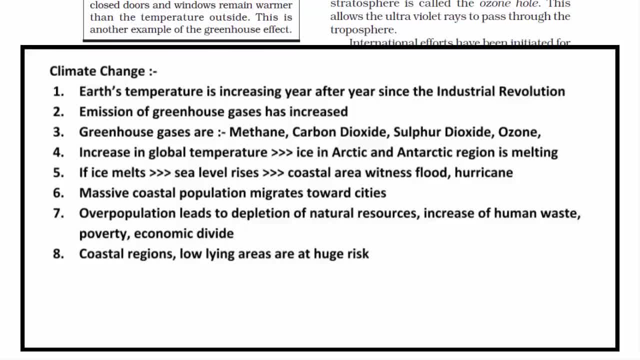 so, because of this internal migration, so, because of this internal migration, domestic migration, that is people domestic migration, that is people domestic migration, that is people shifting from one place to another, shifting from one place to another, shifting from one place to another the domestic population of a particular 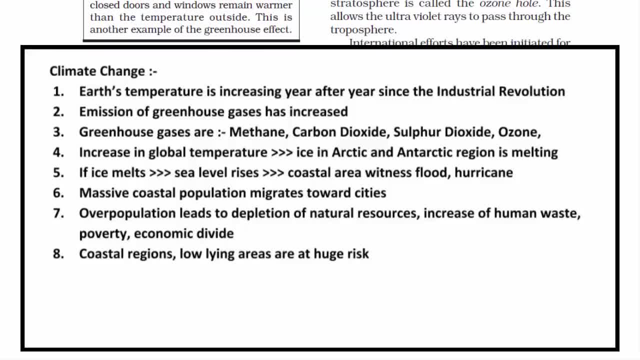 the domestic population of a particular, the domestic population of a particular place will increase. place will increase. place will increase and that will put pressure on that, and that will put pressure on that and that will put pressure on that particular place's resources, particular place's resources, particular place's resources- human waste will increase. then there will 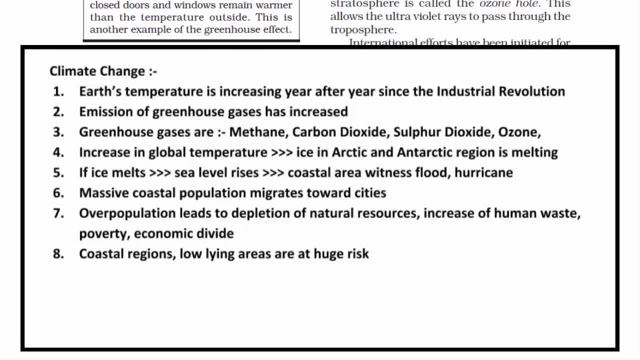 human waste will increase. then there will human waste will increase. then there will be massive economic divide. be massive economic divide, be massive economic divide. so i hope you're understanding the. so i hope you're understanding the. so i hope you're understanding the trickle-down effect. trickle-down effect. 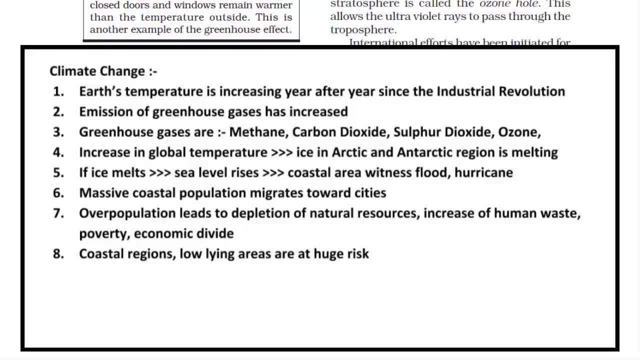 trickle-down effect. so right now, if you see arctic sea ice, so right now if you see arctic sea ice, so right now if you see arctic sea ice is shrinking and glaciers are melting, is shrinking and glaciers are melting, is shrinking and glaciers are melting. and if you want to know what's happening, 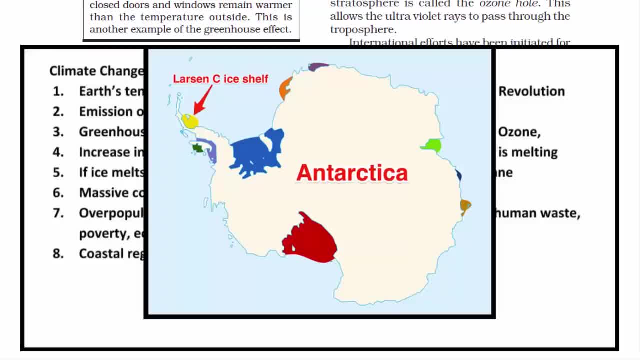 and if you want to know what's happening and if you want to know what's happening in antarctica- a massive trillion ton in antarctica, a massive trillion ton in antarctica, a massive trillion ton iceberg broke from antarctica, just look. iceberg broke from antarctica, just look. 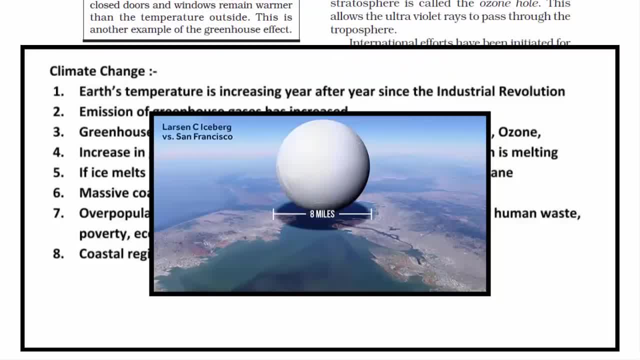 iceberg broke from antarctica. just look at the size of this iceberg, at the size of this iceberg, at the size of this iceberg. now this iceberg is going to melt. and now this iceberg is going to melt, and now this iceberg is going to melt, and when it melts, the sea level will rise. 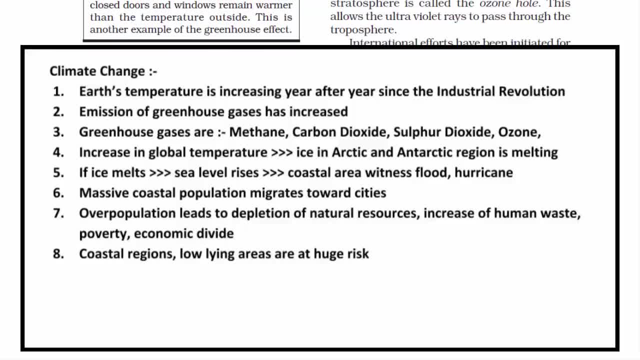 when it melts, the sea level will rise. when it melts, the sea level will rise, and then most of the coastal region of, and then most of the coastal region of, and then most of the coastal region of united states, then indian subcontinent, united states, then indian subcontinent. 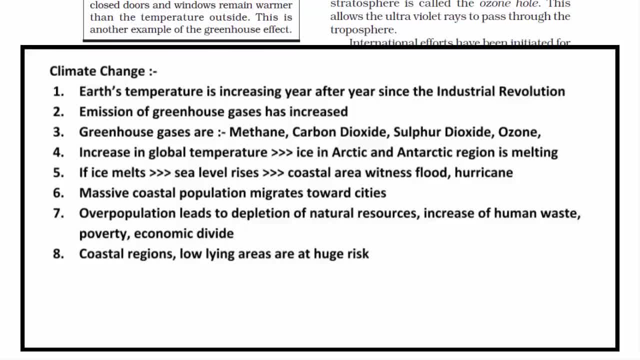 united states, then indian subcontinent, then bangladesh- most of the low-lying, then bangladesh- most of the low-lying, then bangladesh- most of the low-lying areas will get affected. areas will get affected. areas will get affected. so this is the story behind climate. 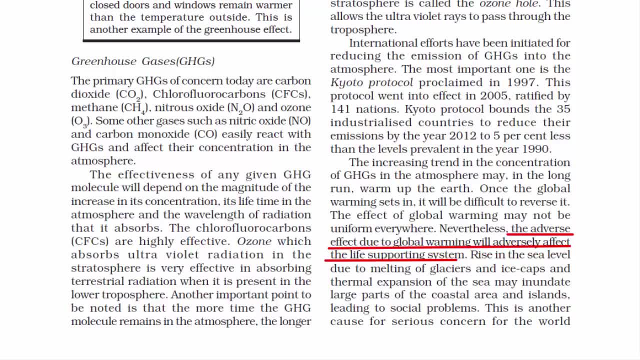 so this is the story behind climate. so this is the story behind climate change, change, change. all right, i hope you now understand what. all right, i hope you now understand what. all right, i hope you now understand what is climate change, global warming, and how is climate change, global warming and how? 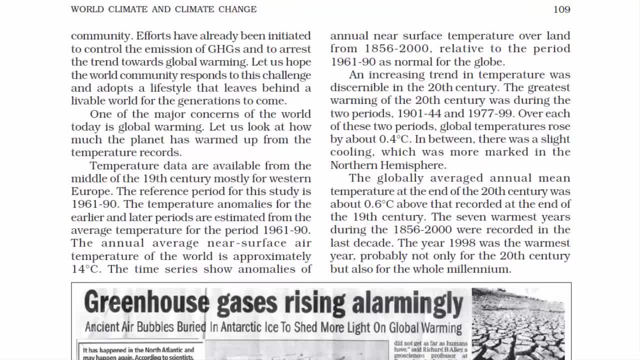 is climate change, global warming and how it affects all of us. it affects all of us. it affects all of us. i just want you to go through all these. i just want you to go through all these. i just want you to go through all these data. you just have to broadly go through. 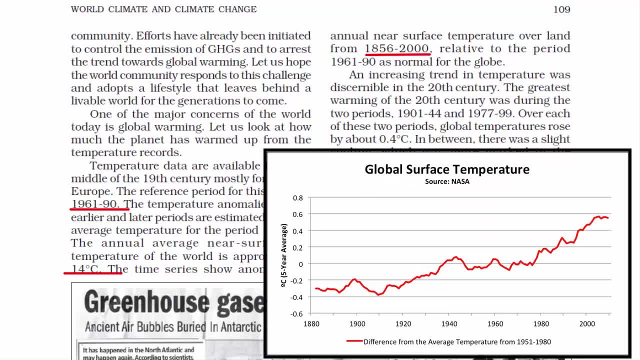 data. you just have to broadly go through data. you just have to broadly go through it again. i've also pretty much covered it again. i've also pretty much covered it again. i've also pretty much covered it when i was talking about the global. it when i was talking about the global. 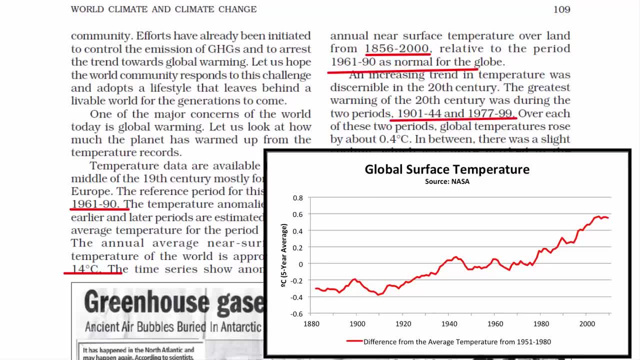 it when i was talking about the global surface temperature. there's a picture surface temperature. there's a picture surface temperature. there's a picture also that i put up, so just go back. and also that i put up, so just go back. and also that i put up. so just go back and listen to it again. 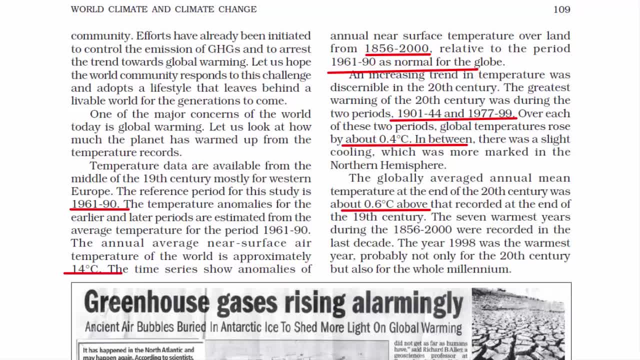 listen to it again. listen to it again. otherwise, just pause the video and read. otherwise, just pause the video and read. otherwise, just pause the video and read it. or you read it from your book and it, or you read it from your book and it, or you read it from your book and that's it. you don't have to remember. 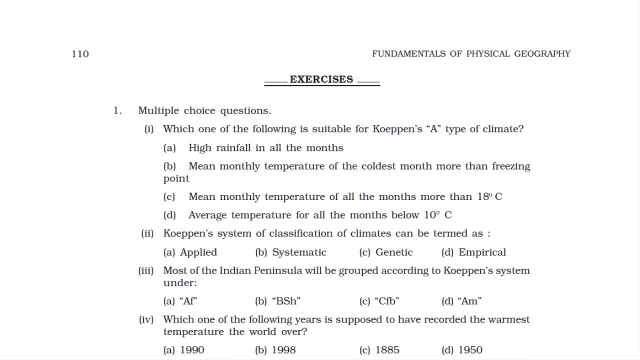 that's it. you don't have to remember, that's it. you don't have to remember everything. just just give it a quick everything. just just give it a quick everything. just just give it a quick glimpse, glimpse, glimpse. all right, then, with this we have come to. 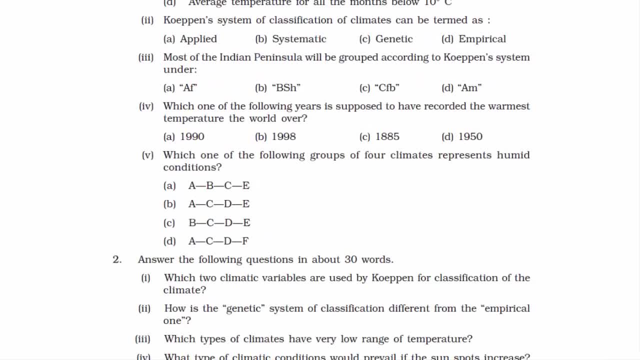 all right, then, with this we have come to. all right, then, with this we have come to an end of this chapter. the question an end of this chapter. the question an end of this chapter. the question answers of this chapter is available on. answers of this chapter is available on. 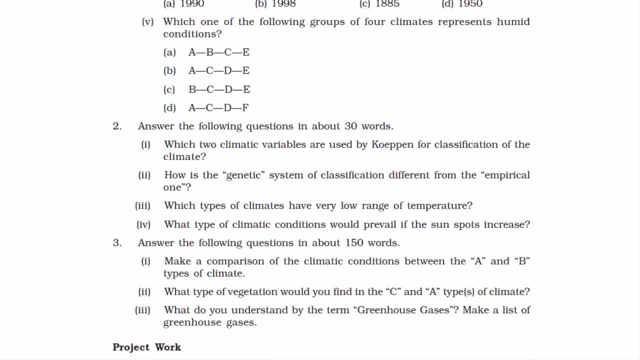 answers of this chapter is available on the website. i put the link in the the website. i put the link in the the website. i put the link in the description. please have a look at it. description. please have a look at it. description. please have a look at it. and i also urge you to watch that. 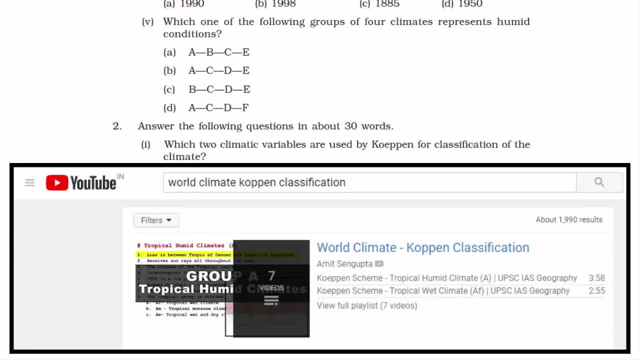 and i also urge you to watch that, and i also urge you to watch that playlist that i've mentioned in the playlist that i've mentioned, in the playlist that i've mentioned in the beginning. that playlist contains short beginning. that playlist contains short beginning. that playlist contains short videos on various climatic groups.